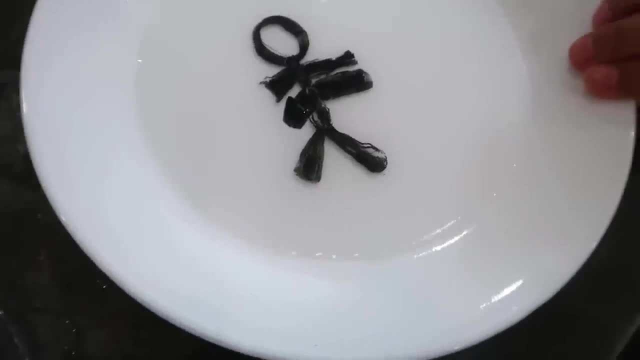 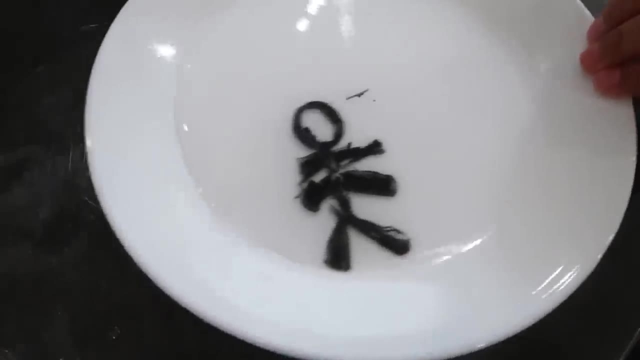 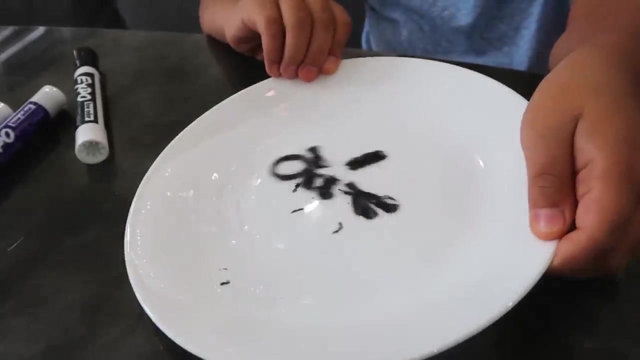 Ah, I feel like the arms or legs are gonna break. Oh, it's moving now. Yay, Now he can just walk. Do do, do, do, do, do. There you go. This is an easy way to make your stick figure float. Do do, do. 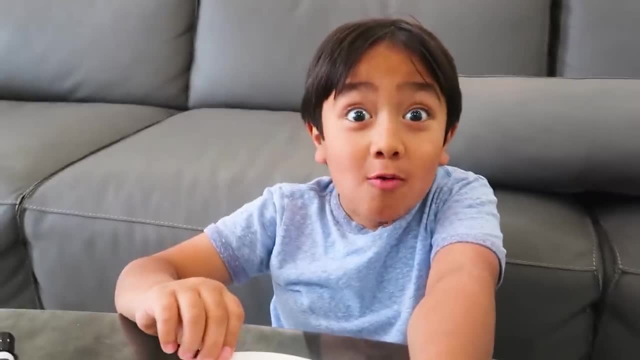 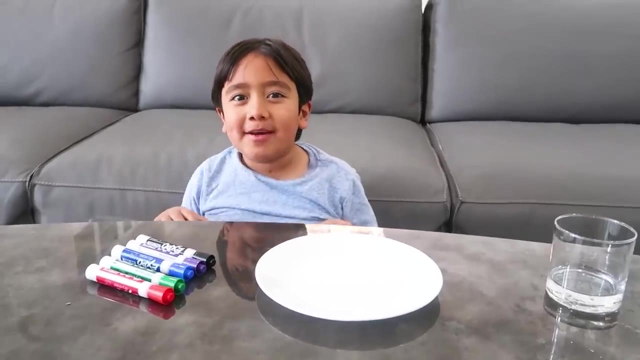 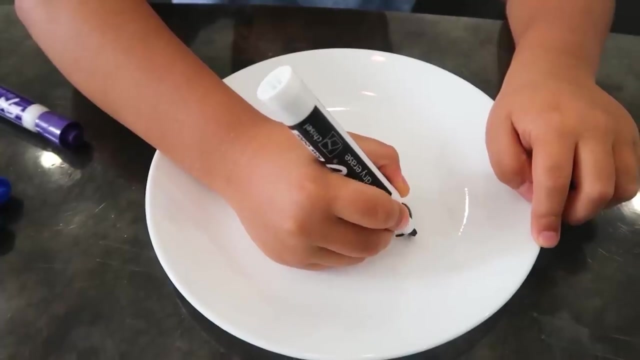 Oh, He broke. This is so cool, You can hold it. Okay, guys, for the next one, I'm gonna make a dog. It should be like this, And then maybe I can put like ears, Ears. I feel like I'm making a cat. 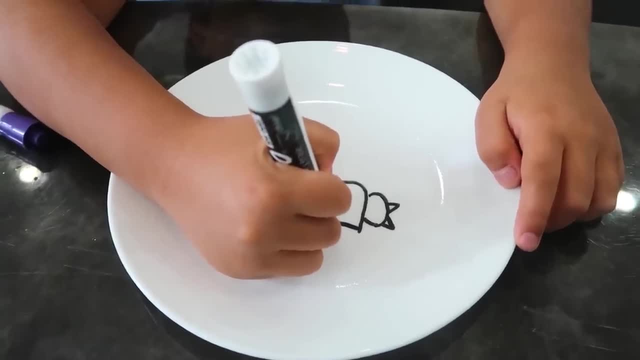 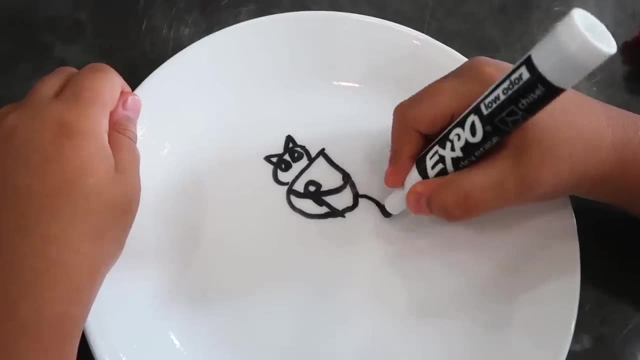 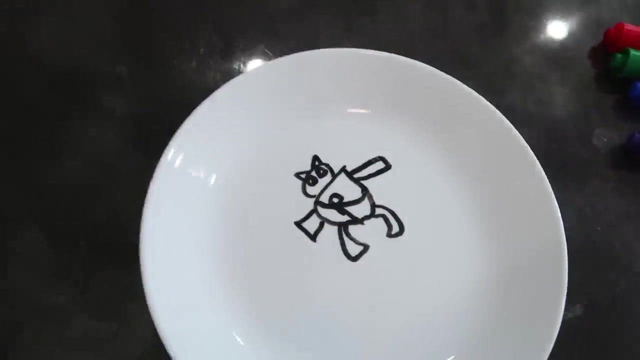 I'm making a big dog or cat. Oh, I can't do it right, Unless I do like this: I put an R, Okay, then I'll make the legs And then the arms. I feel like I'm making like a super strong cat or something. 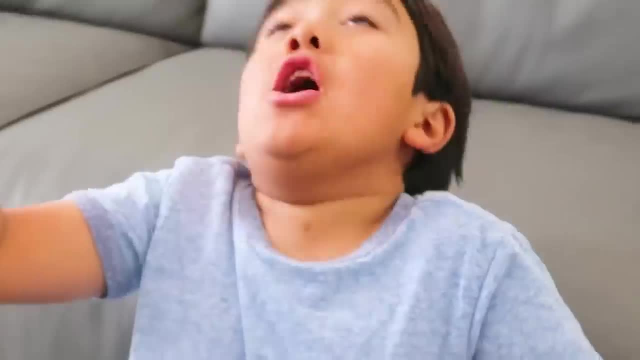 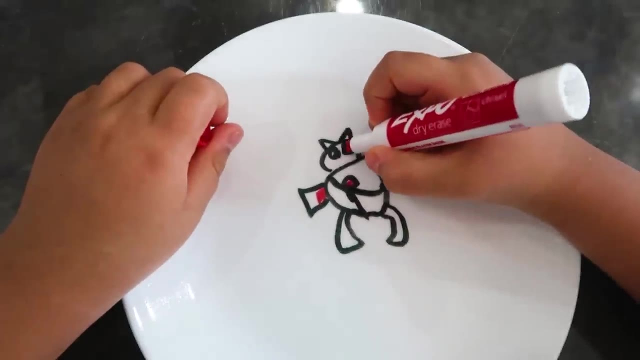 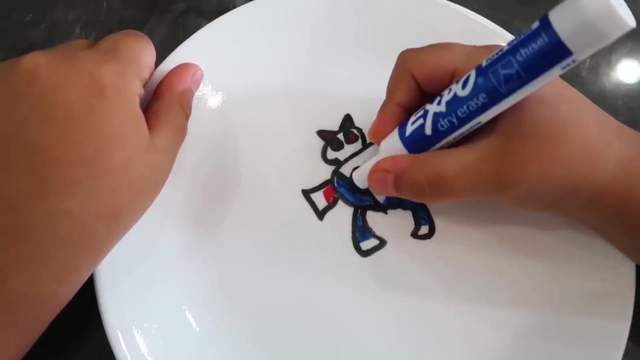 Okay, now I'm going to draw Red right here And then I'm gonna make this red, And then I'll make the eyes red On the ears. Okay, so I'm coloring the pants. He has jeans. Okay, I'm gonna make the skin color purple. 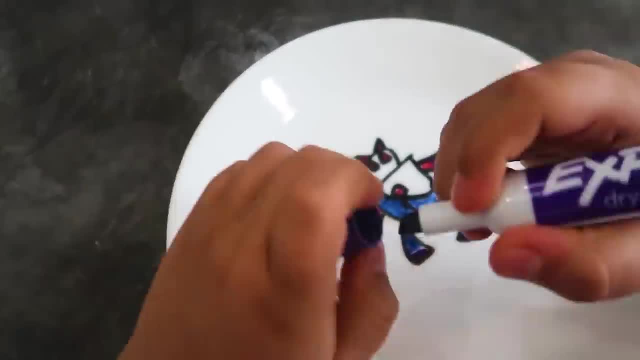 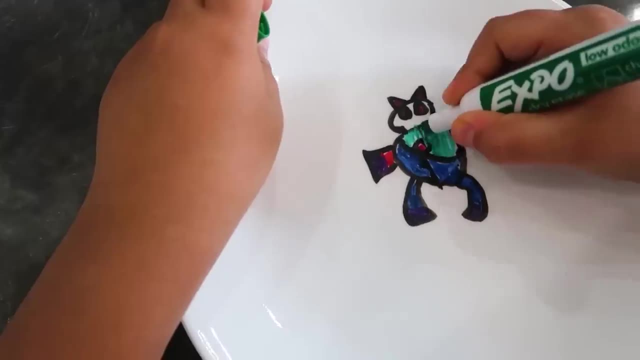 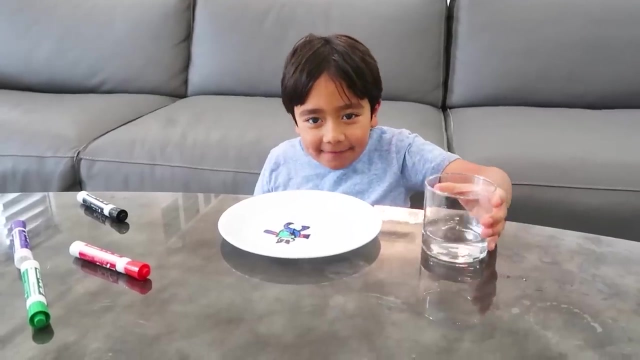 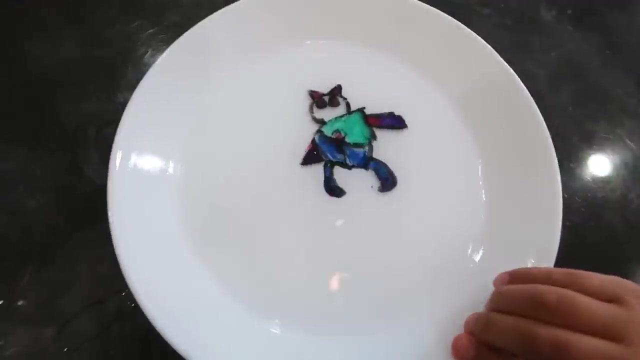 Okay, I'm gonna put it here And I'm gonna put this part green. Okay, Like this, And Perfect. Okay, guys, let's see the float. Okay, That's good. Oh, I'm missing one leg. Oh no, the other leg broke off. 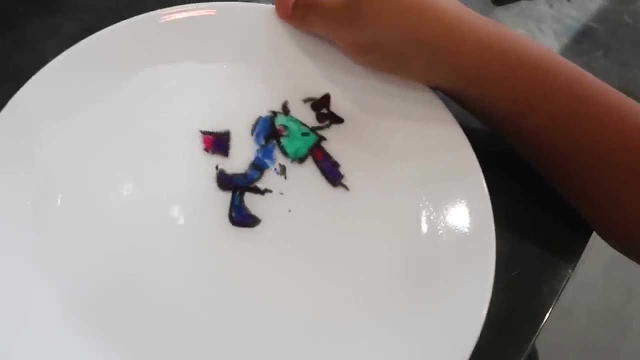 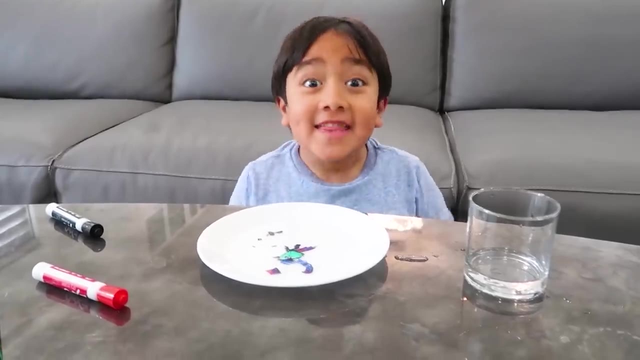 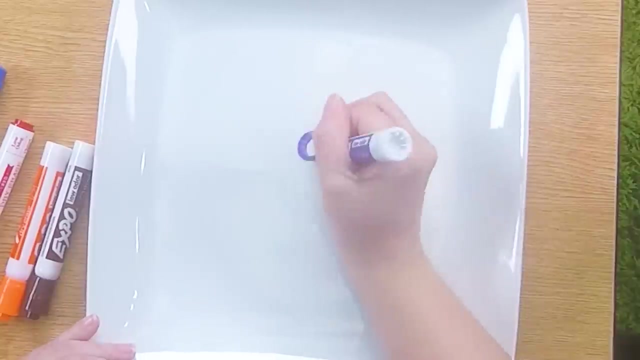 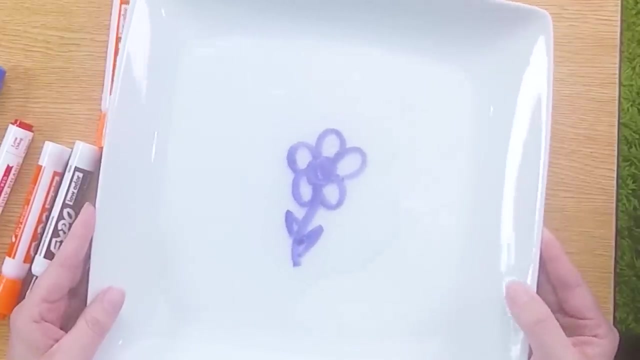 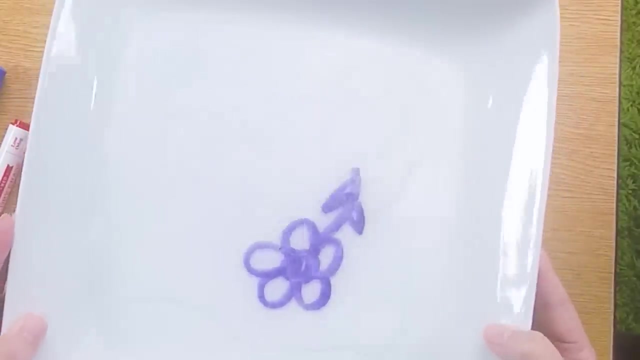 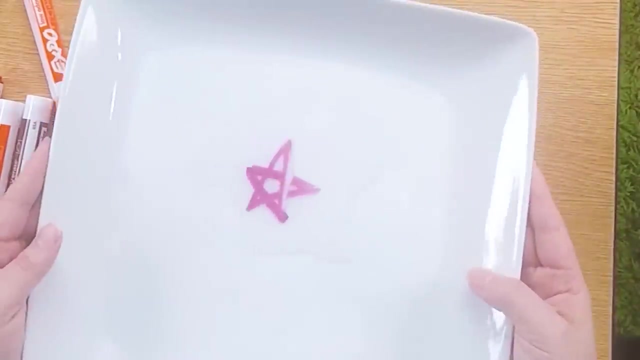 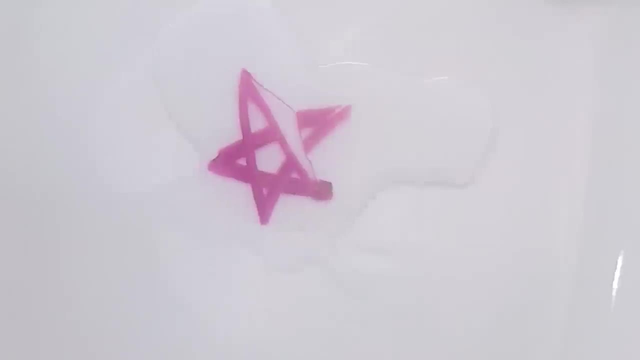 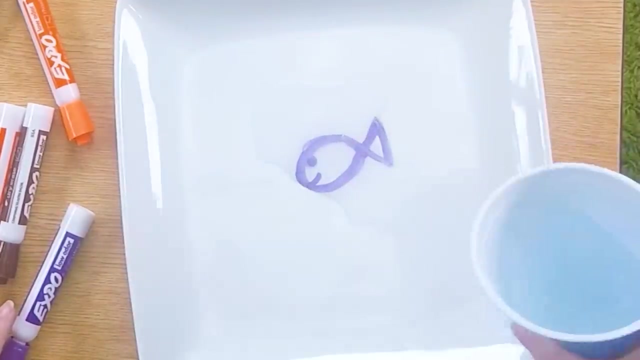 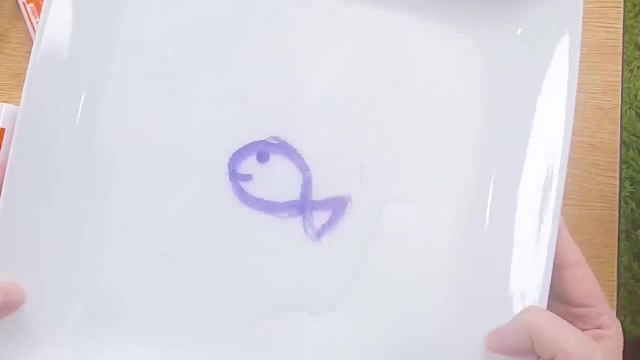 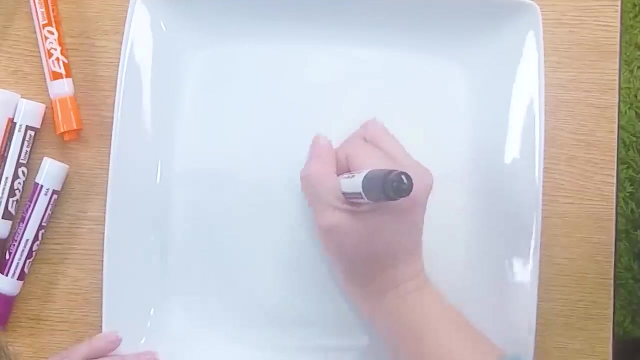 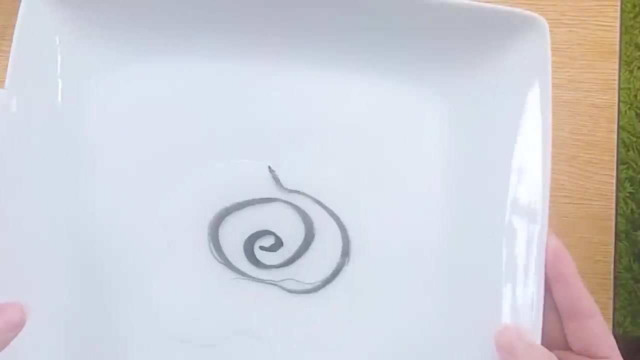 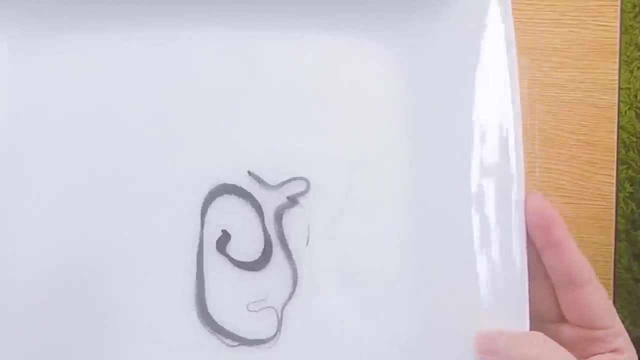 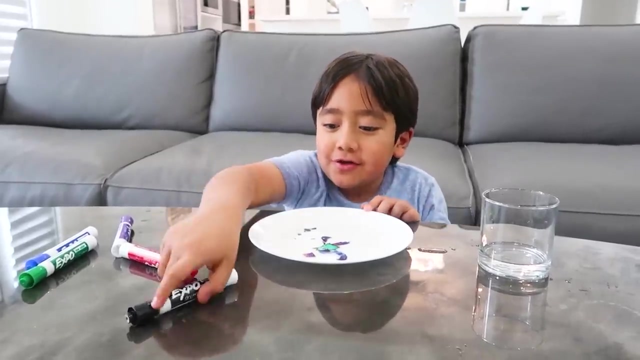 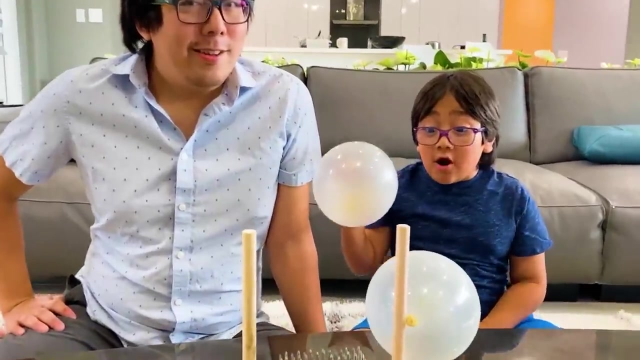 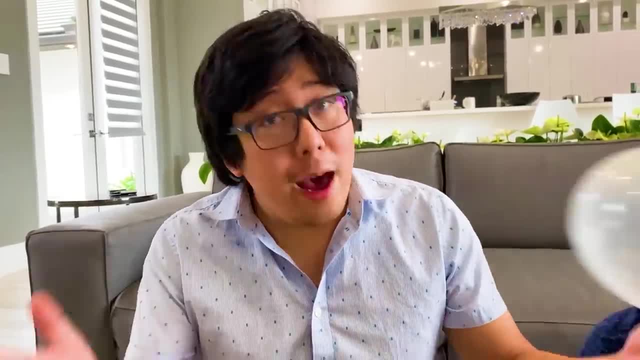 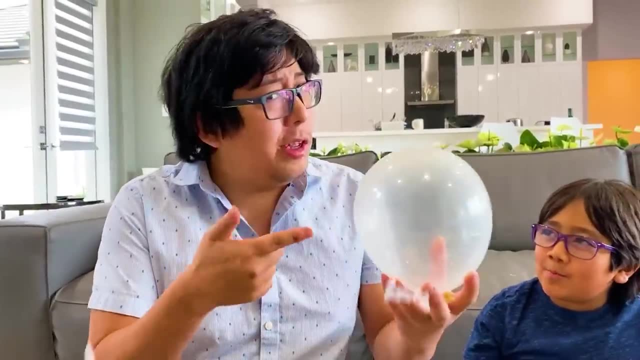 So, guys, if you do this at home, make sure you ask your parents for help. Alright, so today I'm in charge, Ryan, Yeah. So what do you guys think? Do you think the balloon is going to pop or stay the same? 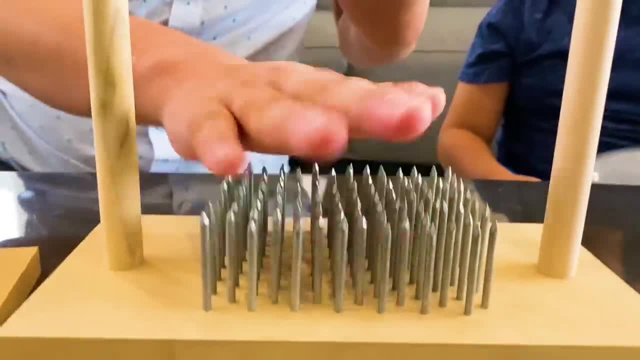 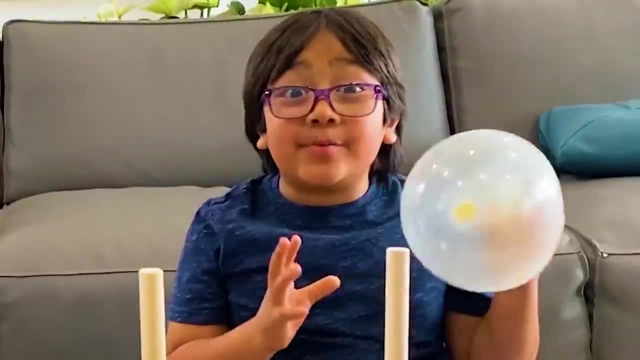 I wonder, Yeah, on top of these nails, Instead of trying it out with a lot of nails, let's do it with one. Let's see what happens. I think it's going to pop a bit. I don't know if you put a lot of pressure. 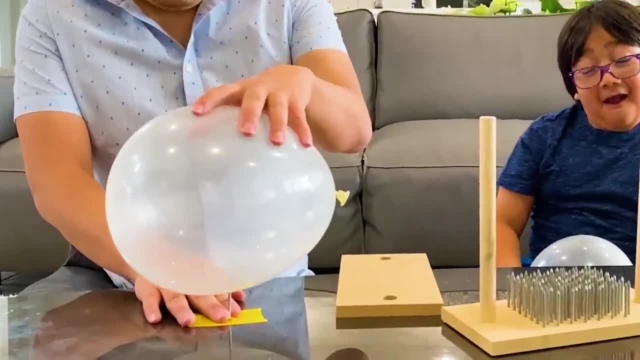 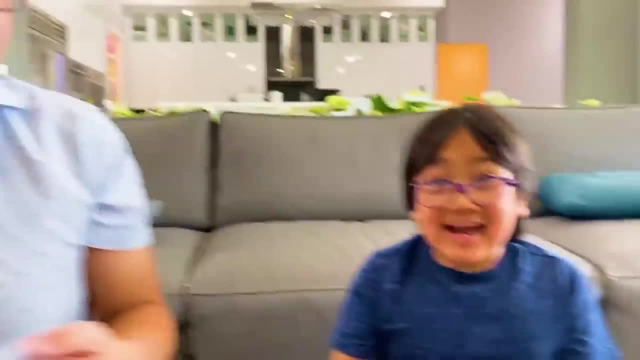 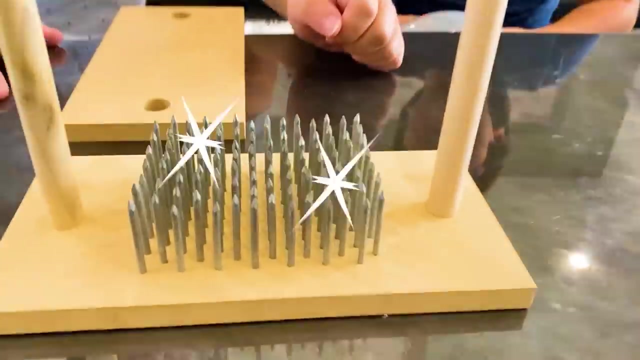 Alright, let's see what happens. You guys ready? Yeah, Alright, probably the same pressure. It did pop. That was scary, Alright. so, guys, now let's try the same thing with a lot of nails. Yeah, Guys, remember there are a lot of nails. 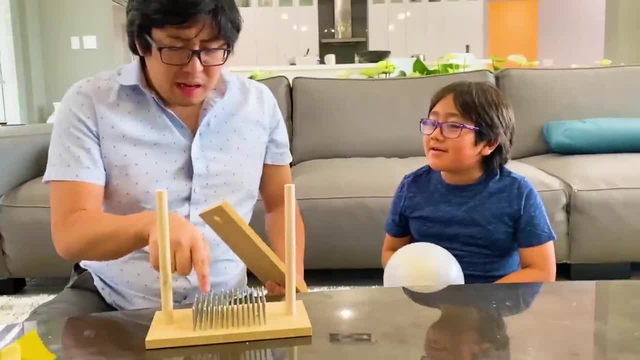 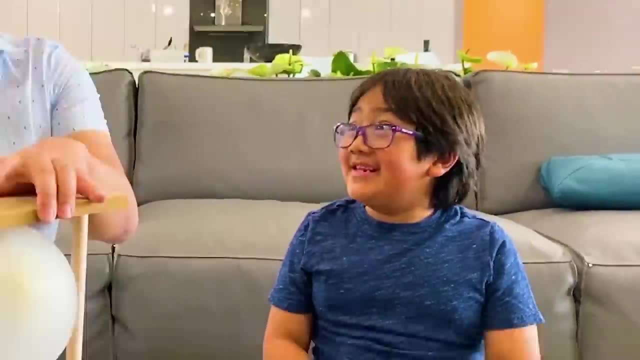 So remember to ask your grown-up for help. Yeah, because they are pointy right, So you don't want to touch it Here. Alright, Ready, So set the balloon. I think I know what's going to happen, Alright, and I'm going to use this board so it won't go anywhere. 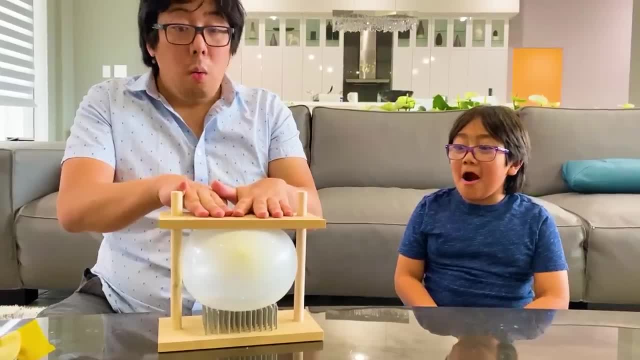 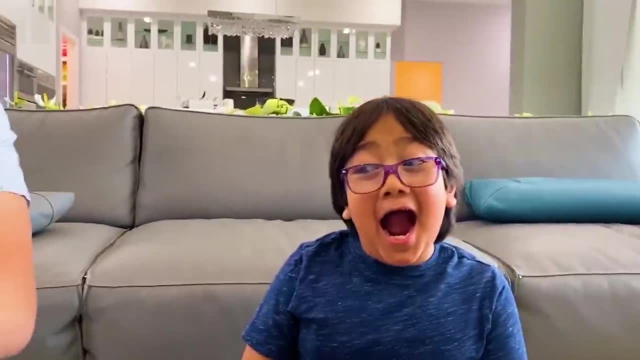 Ready? Mm-hmm, I'm going to press it. Whoa, Good Guys, I'm pressing really hard, but it's still not popping. You see it? Whoa, How come there are so many nails, Daddy, but it didn't pop? 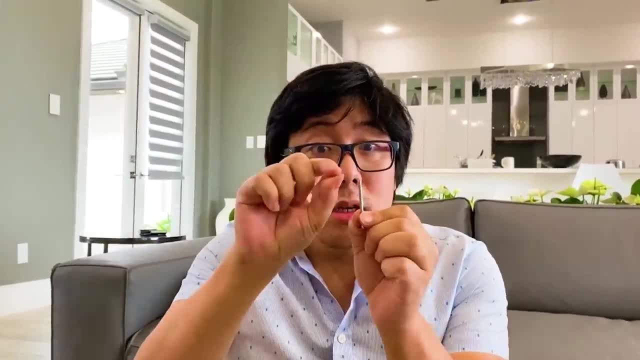 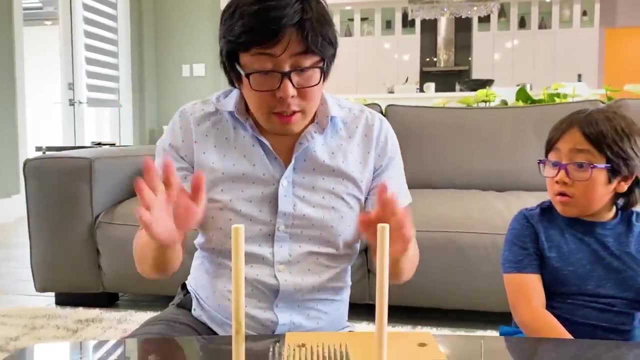 The first time we applied the force into one nail. So the area that we applied the force it's a very tiny area right here. The second time we applied the same amount of force, but this big of an area, For example, if I press you with my finger. 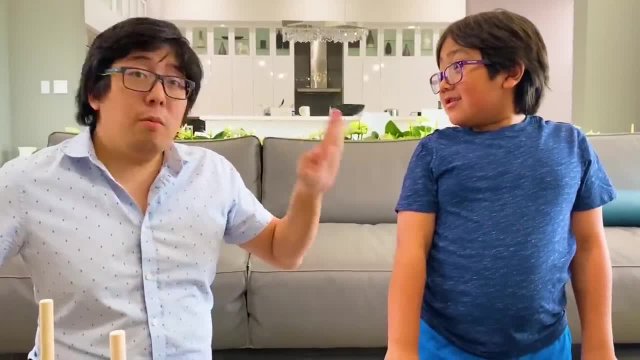 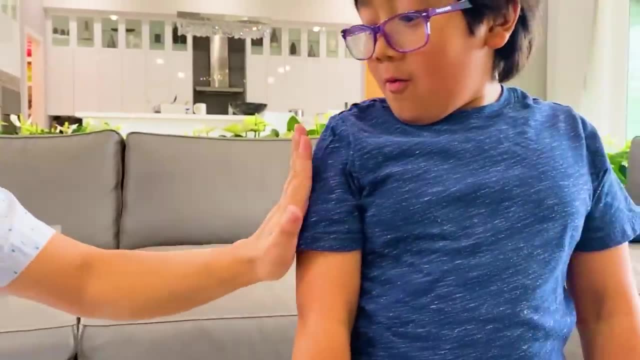 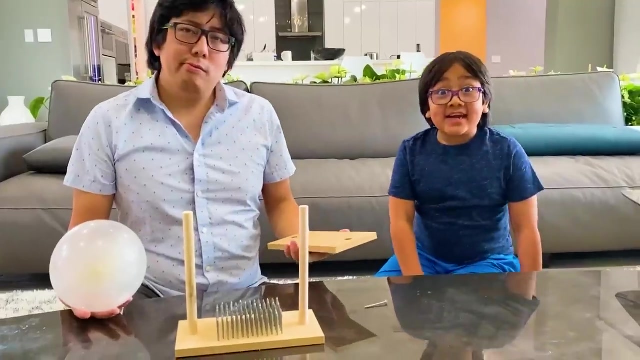 Ow, Right, So the same amount of force, but if I do it with my palm it doesn't hurt, right? No, But I'm applying the same force, but in a different area. Ow See, Ow. But Daddy, can we see how much force it takes to pop the balloon with the giant area? 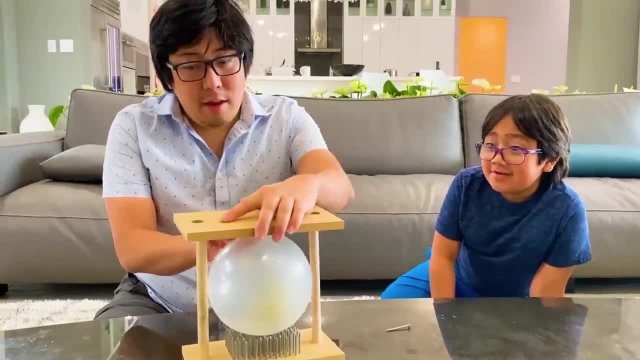 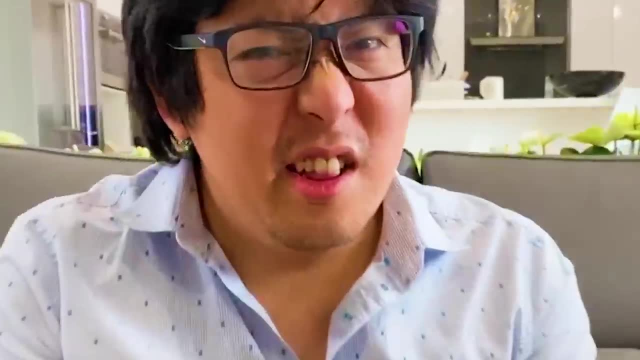 All right, Let's see, Because earlier we couldn't pop it, Daddy, it was like all the way down here. But if I press it with my 100% force, what's going to happen? Are you doing 100%? 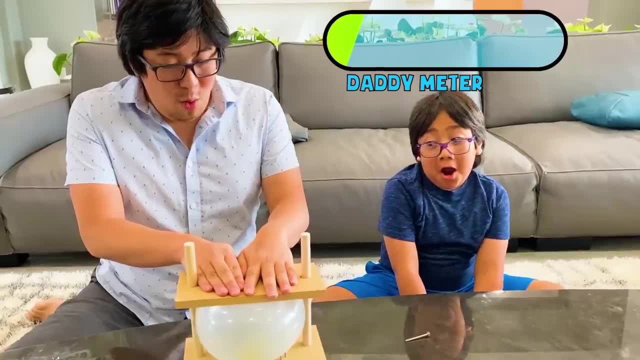 Not yet. Oh my gosh, It's still not popping. Can I even pop? No way, It's still not popping. Are you at 100% yet? No, Oh my gosh, It's still not popping. 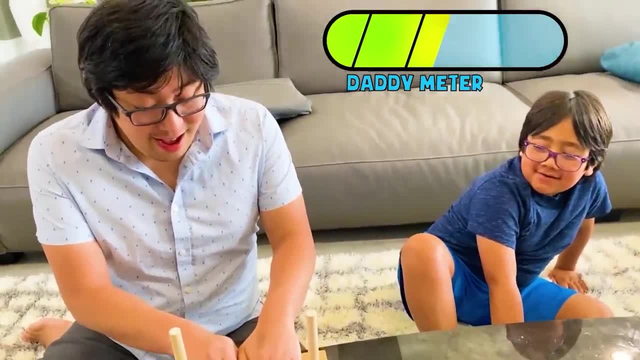 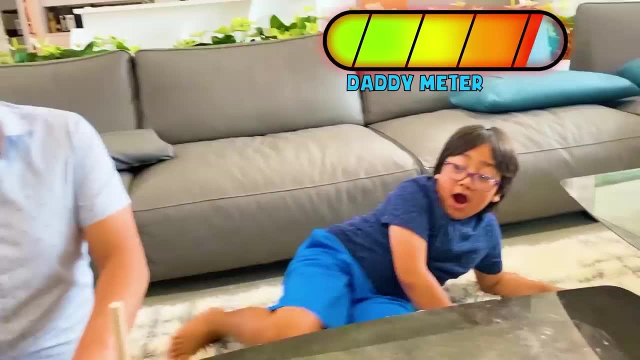 Can I even pop? No way. Are you at 100% yet? Yeah, Oh my gosh, You ready, Okay, I'm going to reach my 100%. You ready, Okay, Okay, Okay, Still not popping. 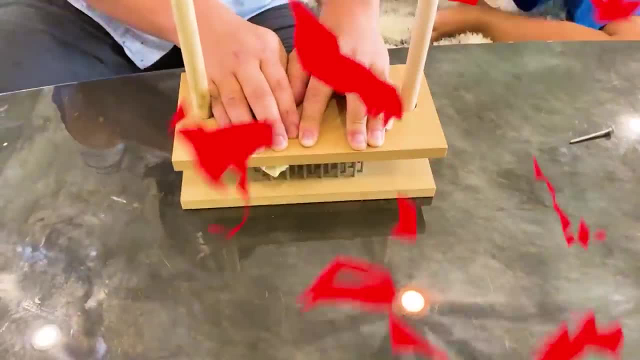 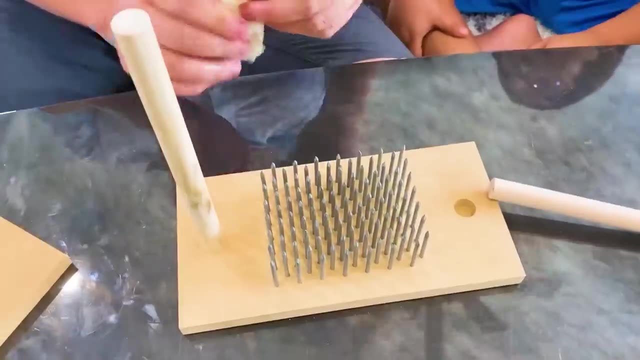 Look at this, Look at that, Look at that. Wow, That was hard, But did you see how much force I applied? Yeah, Because the area was so much bigger so I had to apply a lot bigger force, But I did it. 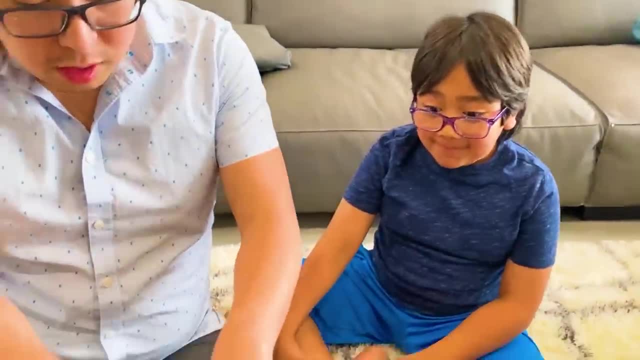 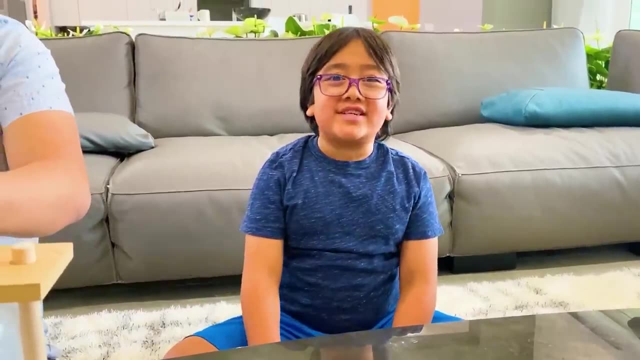 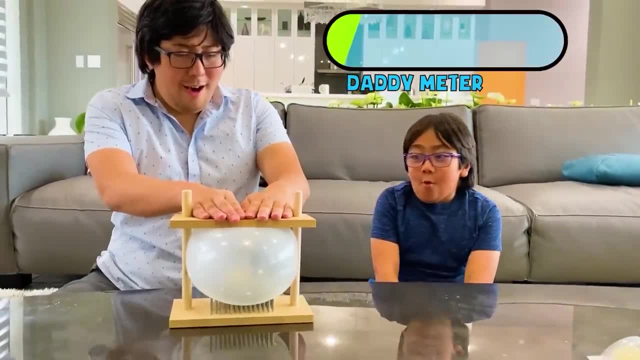 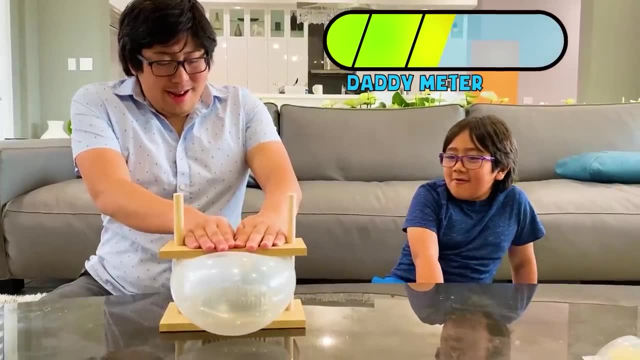 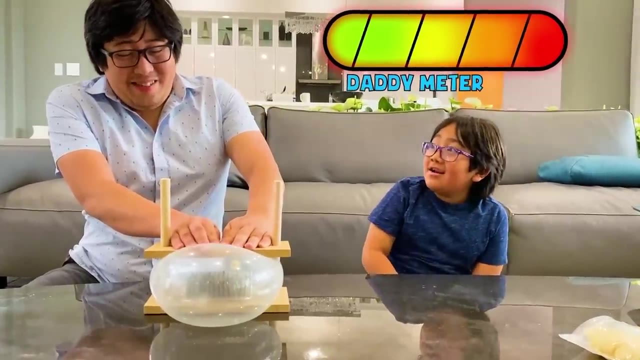 All right, Let's go. Wow, Okay, I'm pressing a lot, Pressing a lot. Do you have to go all the way back down again? I guess Still no. Whoa How? Almost all the way down. 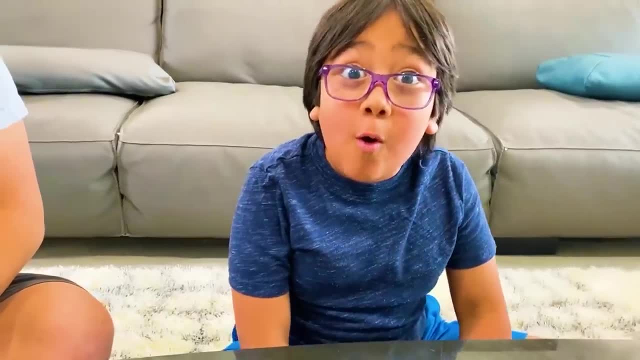 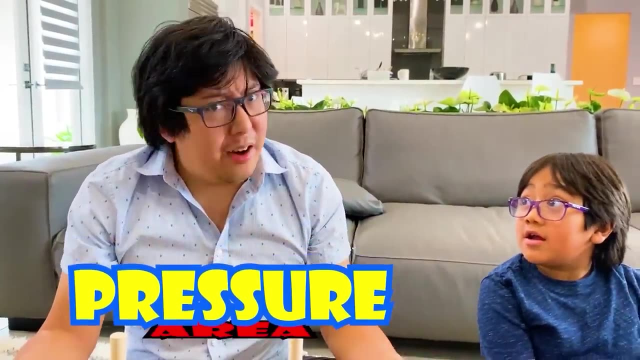 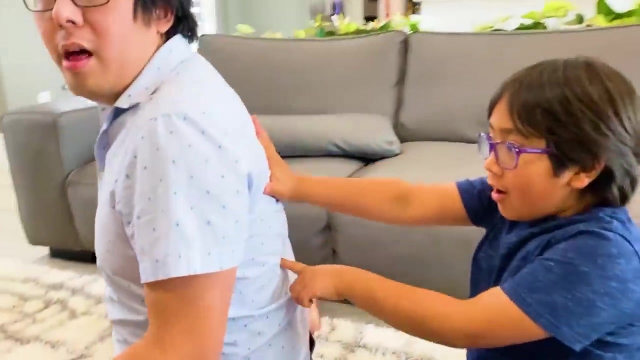 That was so cool. Yeah, The experiment teaches you the concept of pressure. The pressure is the amount of force applied over the area. So the smaller the area is, the higher the pressure. For example, with the same amount of force but applied in a smaller area, it makes the pressure higher. 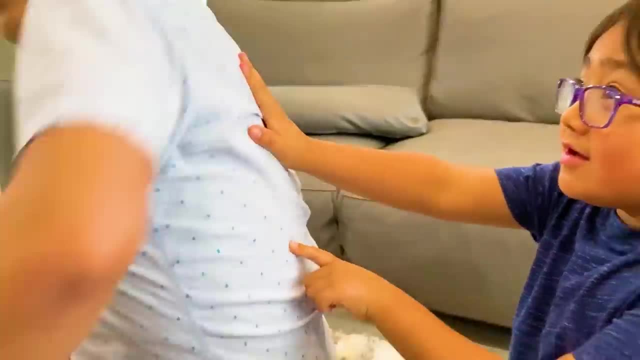 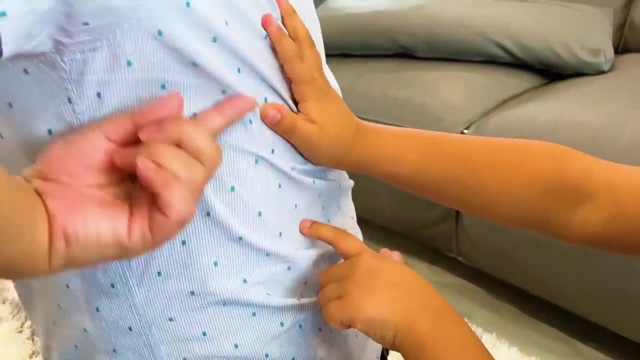 Ow, your finger hurts, Ryan, So same amount of force, but the one you're pressing with your finger is higher pressure than the one you're pressing with your hand. Yeah, Hey guys. Today I'm doing the Free the Animal Challenge. 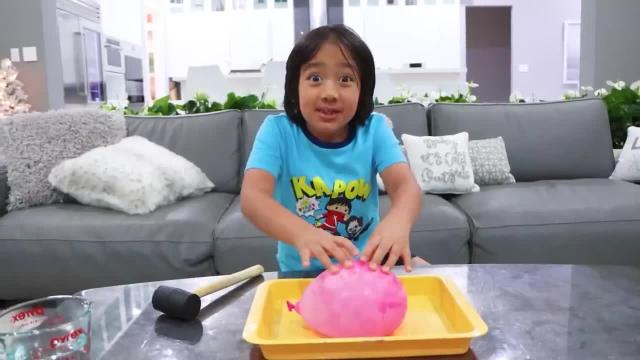 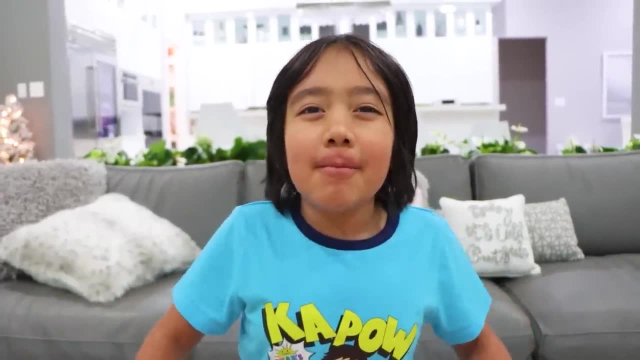 Mommy put a shark inside this balloon And this balloon is filled with ice And I'm going to have to free the shark from the balloon. And first, here's how Mommy did it: First grab a balloon, Then get your favorite toy. 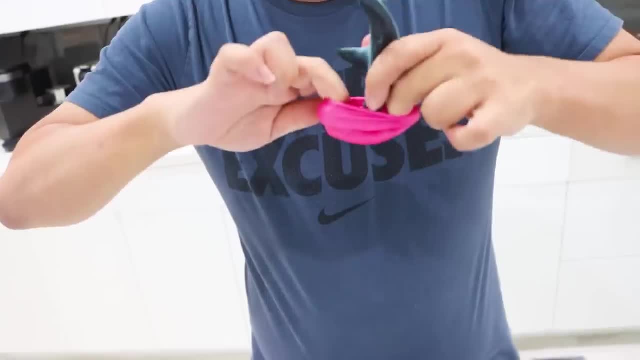 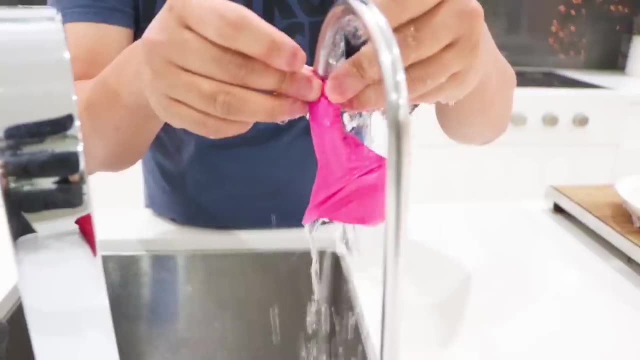 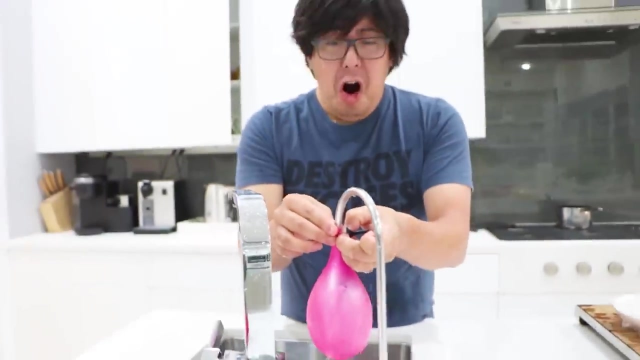 Carefully put the toy inside the balloon, Did I mention carefully, Once the toy is inside, fill the balloon with water. Oopsie, Carefully not to splash water everywhere. The balloon will get bigger and bigger. Then remove it and put it on the tray. 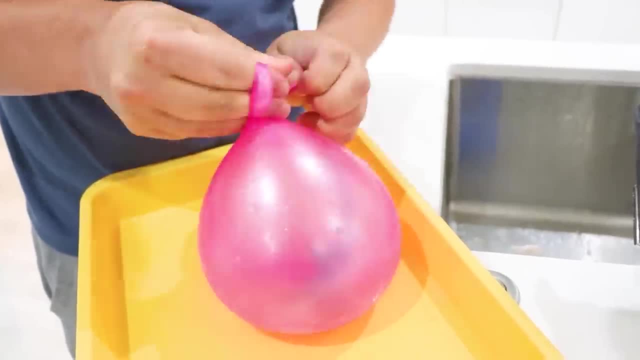 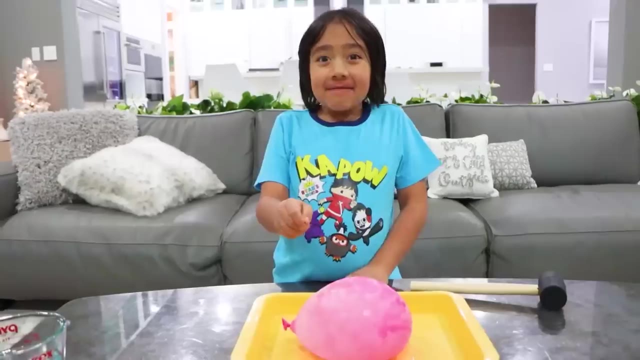 Next, tie the balloon so the water won't spill out everywhere. Next, put the balloon in the freezer until the water inside becomes ice. OK, first I'm going to try to get rid of the balloon, And also, don't forget to ask a grown-up for help. 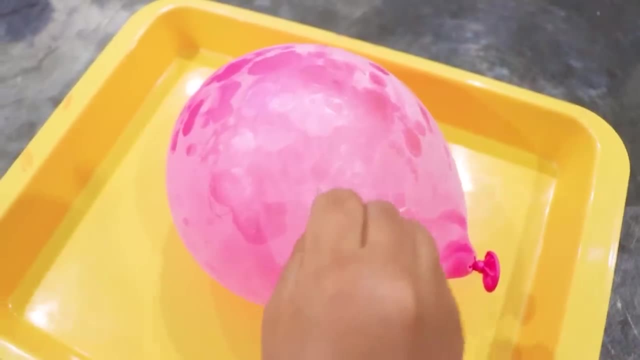 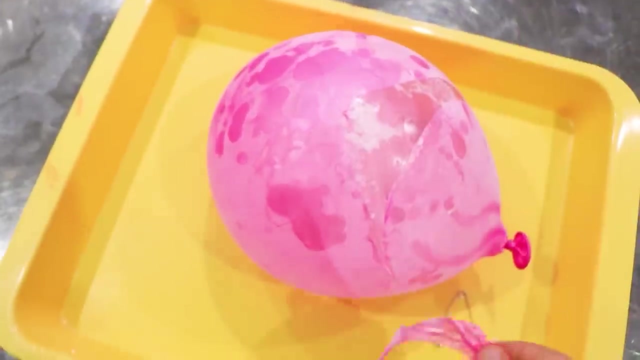 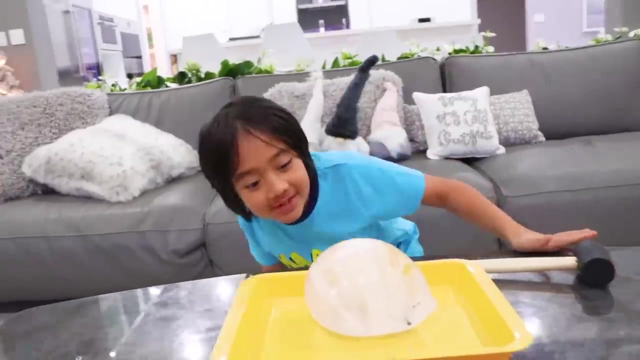 I have Mommy here, Hi. What It's not breaking and it's super strong. What I'm going to take the balloon off and you won't even see a difference. Wait, guys, I think I see the shark inside somewhere in the ice. 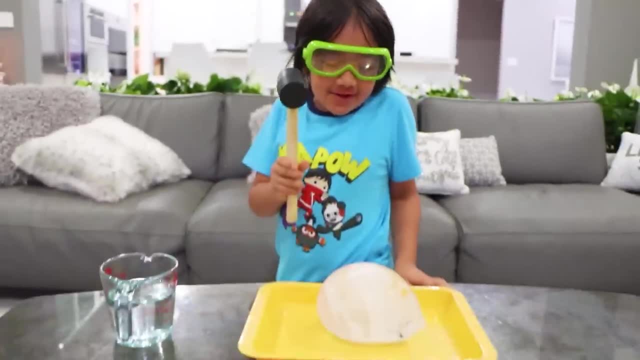 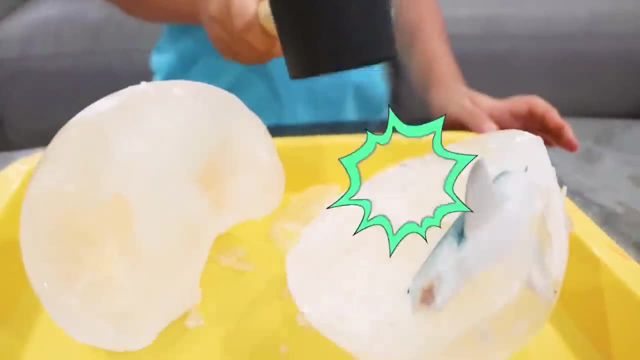 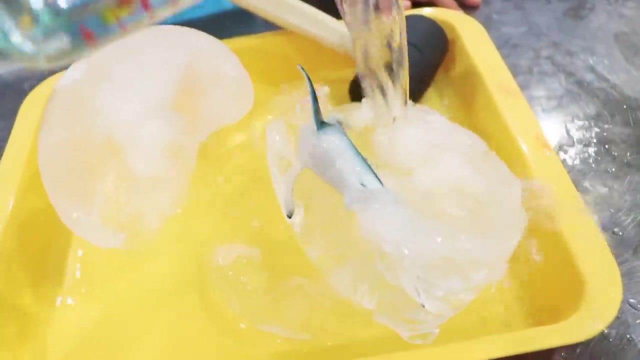 First I have my goggles, just in case. OK, let's get started. Oop, I already cracked it. Ah, I see the shark already ready, but I'm gonna try to use warm water. it's working. it almost got the. 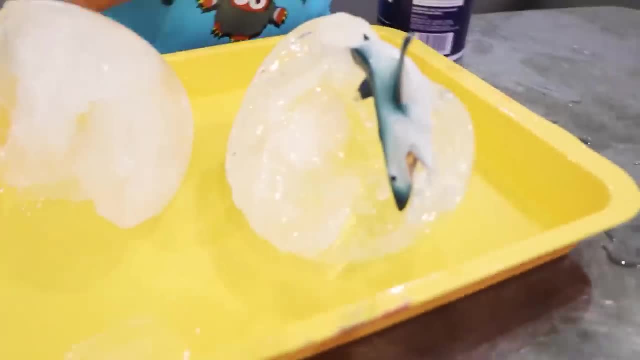 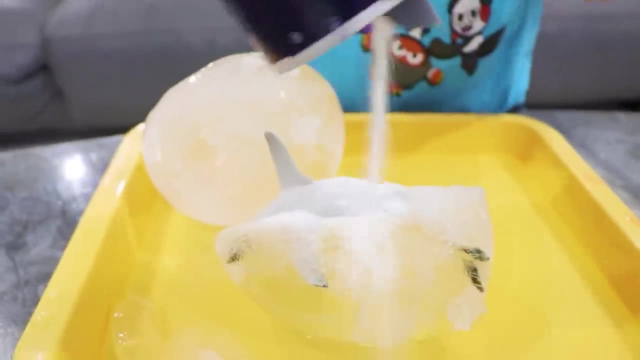 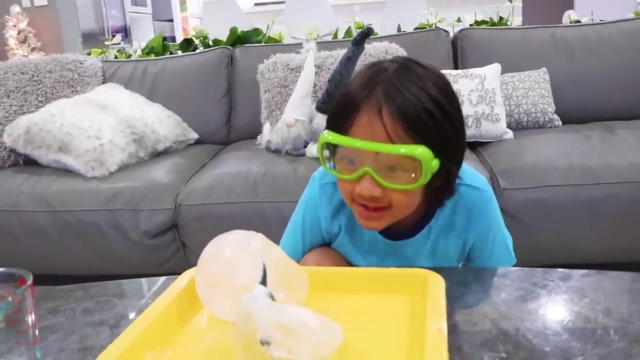 shark out. he's right there, but his fin and his tail is stuck. I think that I can use salt. oh, oh, oh, oh, oh, oh, oh, BAM. so I hear the ice crackling. guys, it's working. I don't want the shark to crackle. I think I have an idea. mr shark, let's. 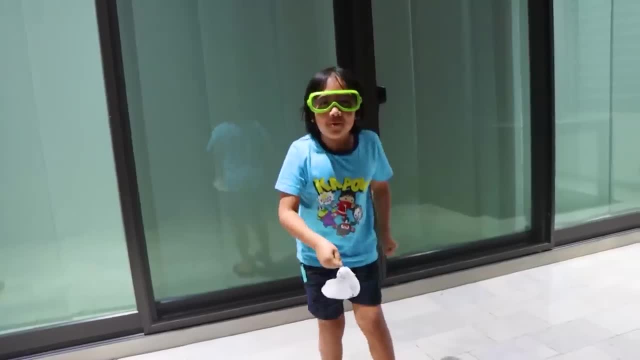 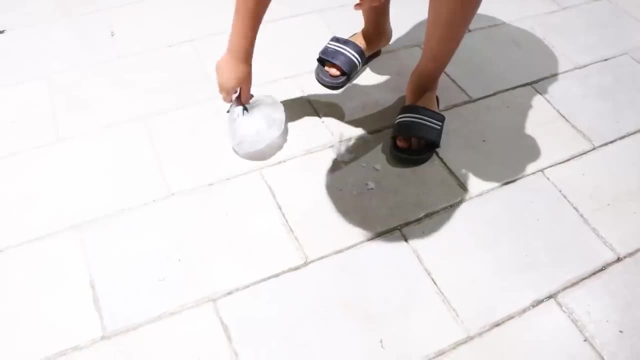 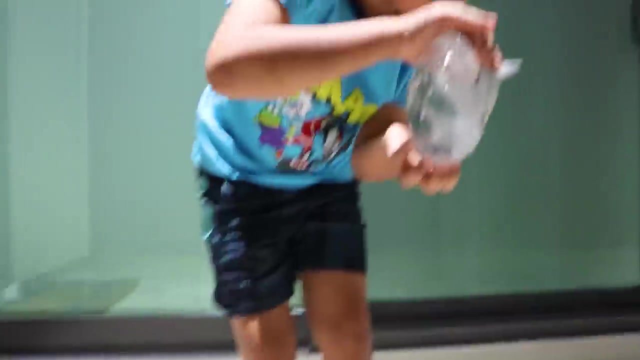 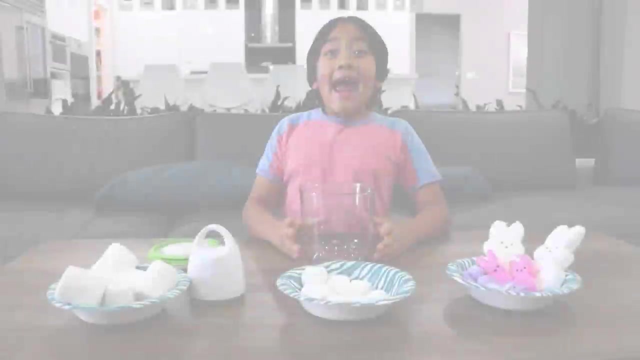 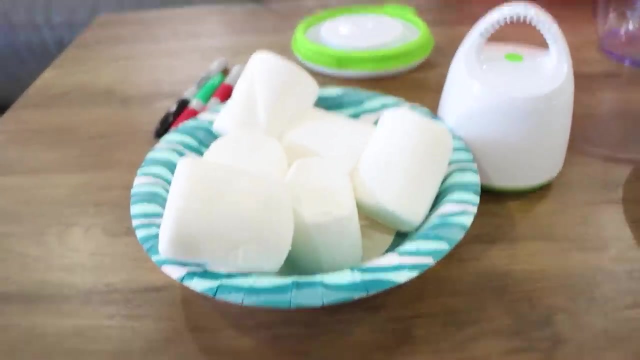 take it outside. remember, I would only do this with adult supervision. three, two, one. I think I'm out. no, not yet. his tail is still stuck. yes, I got the shark. thank you for rescuing mr shark with me. hey guys, today we're doing the marshmallow in a vacuum experiment. that's right, guys. so we have some giant. 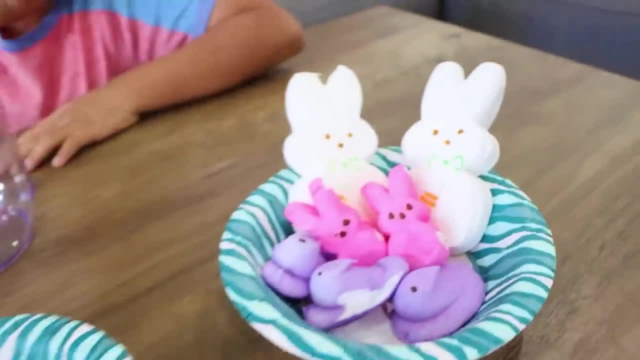 marshmallow, got some regular sized marshmallow, got some funny bunnies and chick marshmallows, and here we just have a container and we put the marshmallow in there, and now we're gonna put the marshmallow in the container and put the marshmallow in the container and put the marshmallow in the. 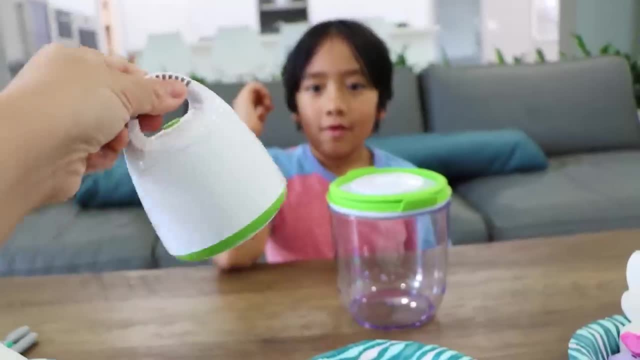 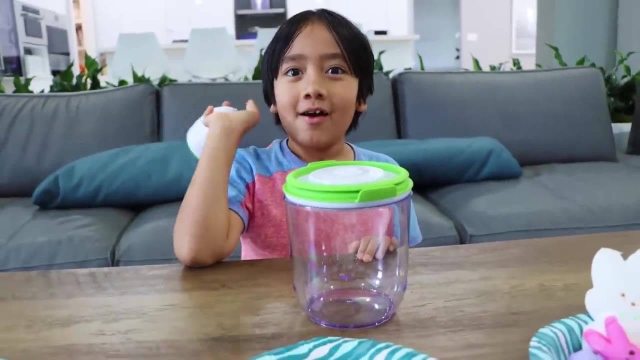 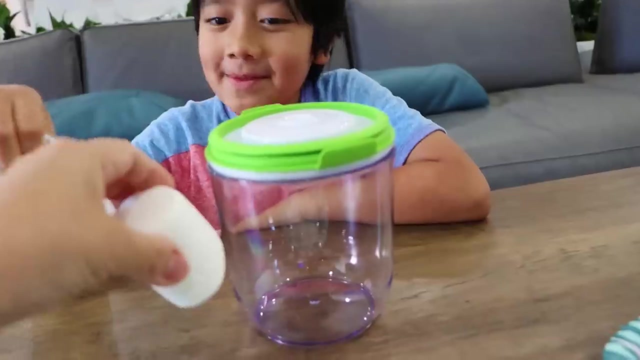 Yeah. so when you put it in here, what's going to happen is you've got this device here and all the air will be sucked out. So then, when you have no more air, it creates a vacuum. So before we begin, I want to ask you guys: what do you think will happen, Ryan, when you put the marshmallow in the container and suck out all the air? 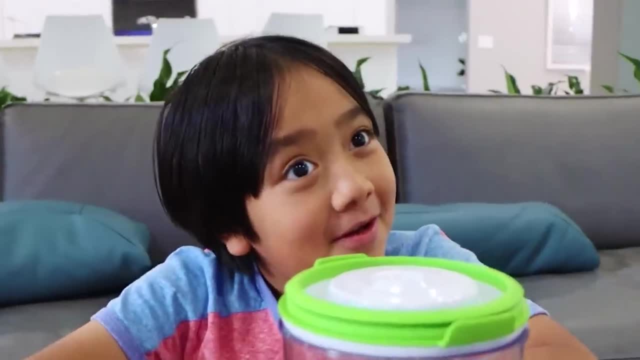 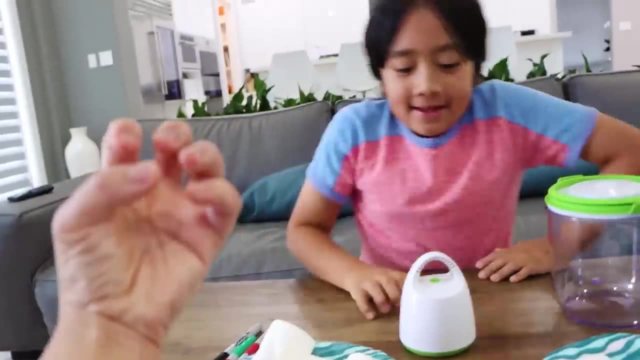 I think the marshmallow will be dried up. Be dried up, Yeah, maybe. Oh, you think so. Maybe you're right. Maybe if there's no air, it'll be all dried up, so it would be smaller or bigger, It'll be squished or expand. 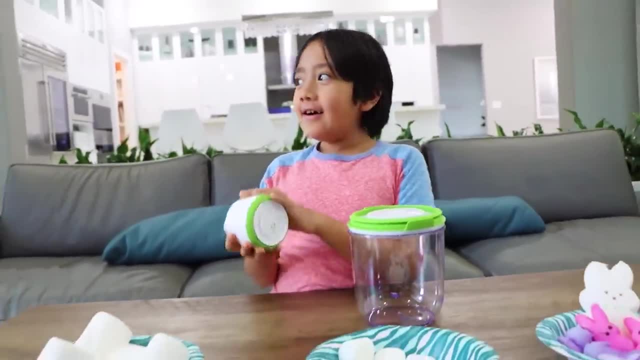 Smaller, Smaller, Yeah, Okay, what do you guys think? Okay, so let's test it out here. First, let's start with regular-sized marshmallow. You want to try that? Yeah, So we're going to open up. 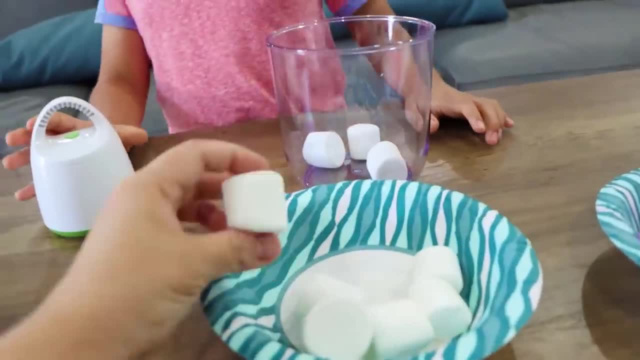 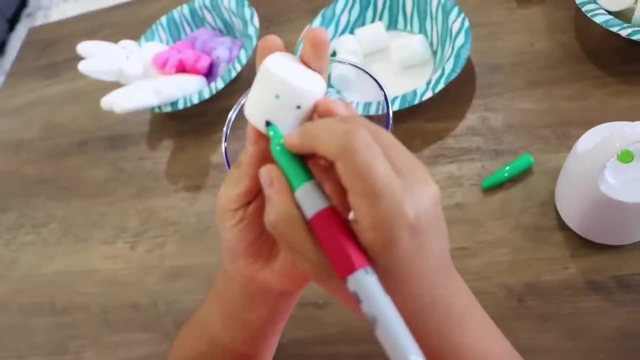 Okay, let's put one tree, Okay, and then you'll be fun. You can also make faces on the marshmallow. So here you do a face and I do a face, Okay, Okay, Just see what happens. 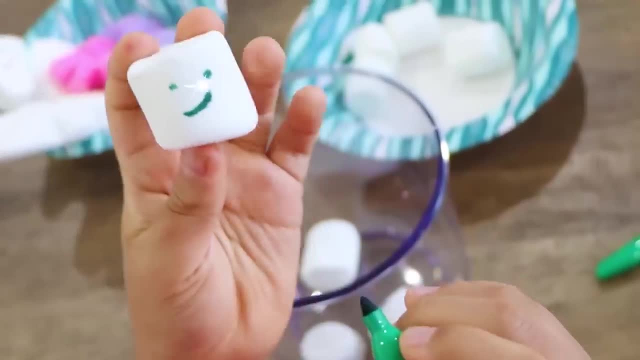 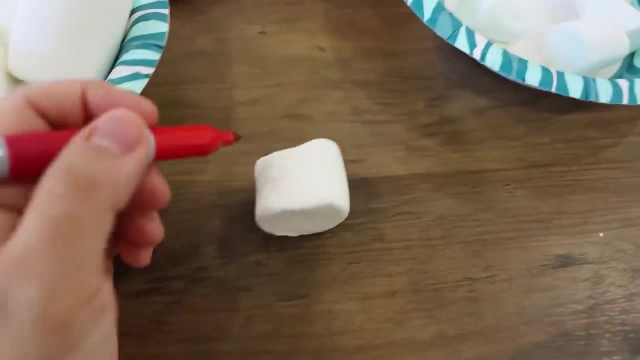 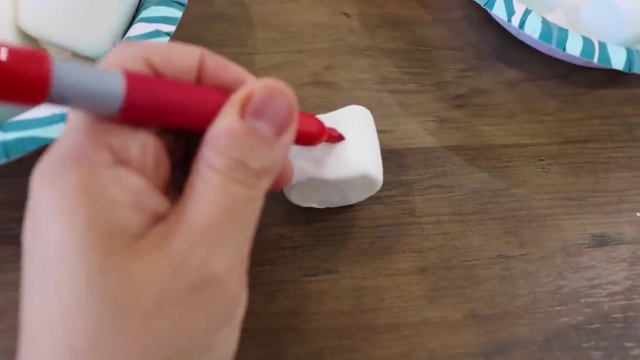 Let's see what happens to it. Bam Eh, half face. Okay, while Ryan's finishing up, I'm going to do mine. What should we draw, guys? You know, I'm not sure how it's going to be in the vacuum, so maybe I'll draw little eyes, little eyes and then maybe a sad face. 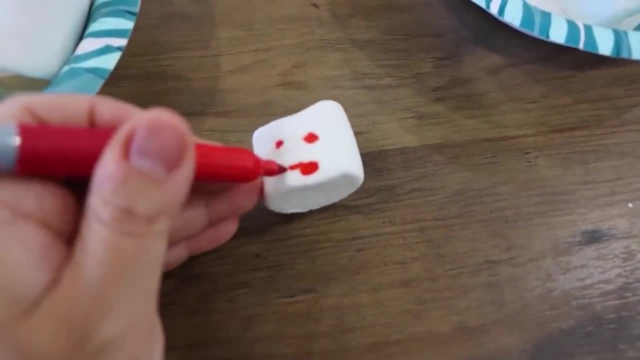 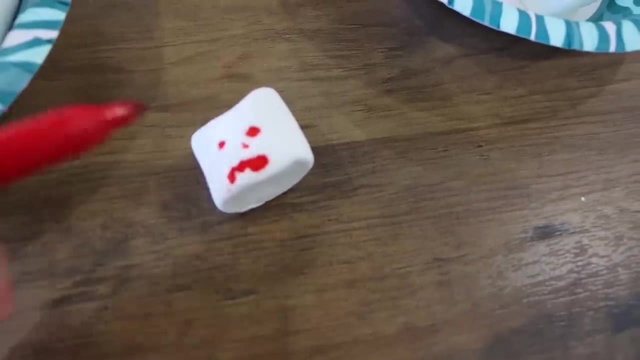 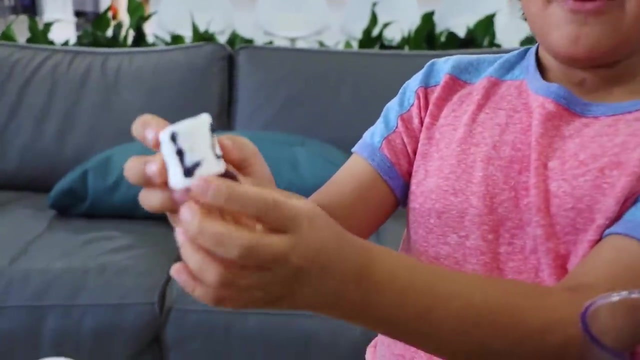 Let's see if I can draw a sad face with one hand. Ah, harder than I thought, guys. There it is Sad Little marshmallow Boop. It has E on the top, Uh-huh, And it has the face, and then it has L O, L and then the face again. 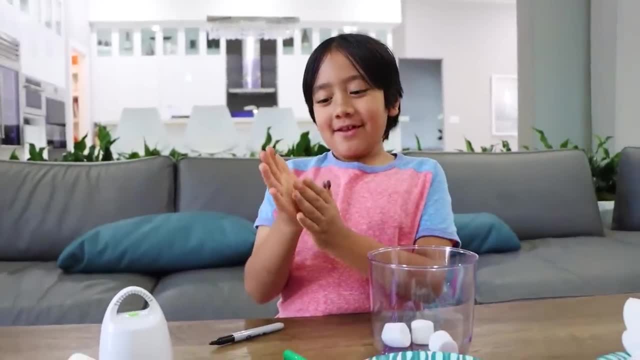 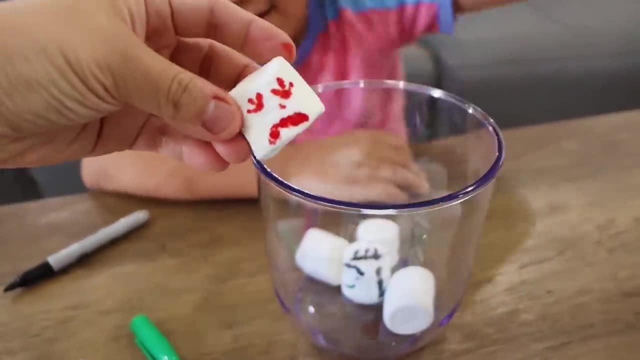 Oh, LOL. What is L for LOL-y, LOL-y? Okay, Okay, guys, I'm going to put mine in. Okay, me too. Sorry about my scary face. Scary face here. It's not Halloween, Mommy, right. 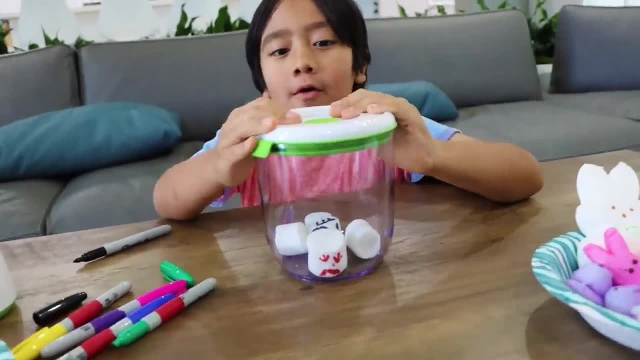 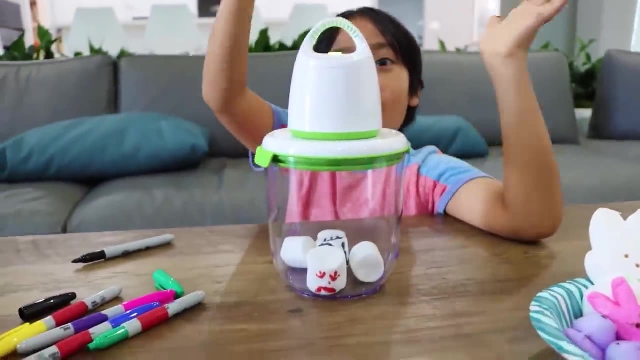 So I'm going to put this on top, Okay, close it up tight, Okay, And this is going to suck out all the air. So you're going to put this and press the button. Press the button. Okay, let's see what happens. 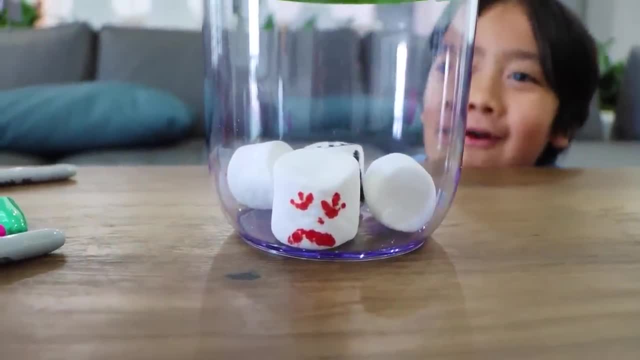 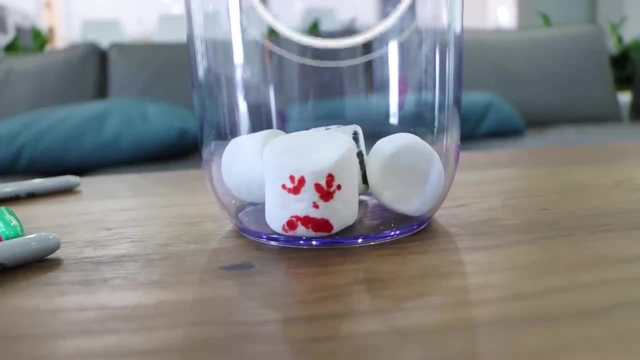 It's going to do it fast. It's taking time. It's probably hard to tell Here. I'm going to go over here so I can see. Do you guys see or not see? Okay, Sucking out all the air as we speak. 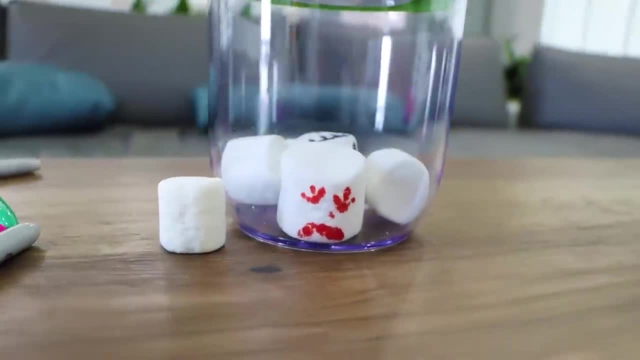 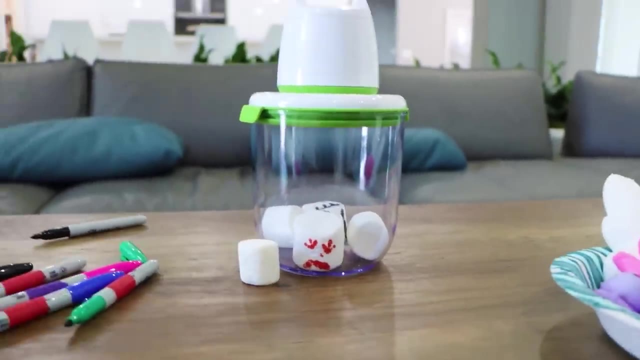 Okay, And then here was the original marshmallow. You guys can't tell. So, Ryan, what did you notice? This was the regular marshmallow, and then here is the one in the vacuum, So Actually it feels like they got bigger. 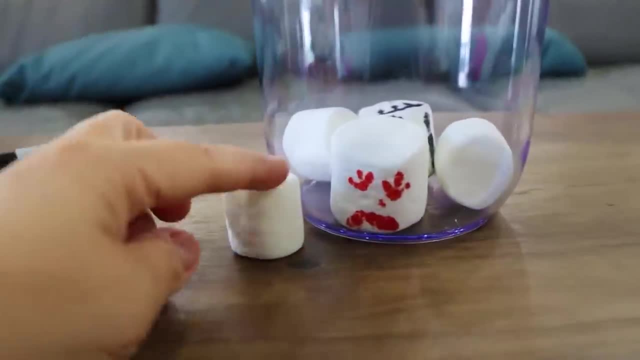 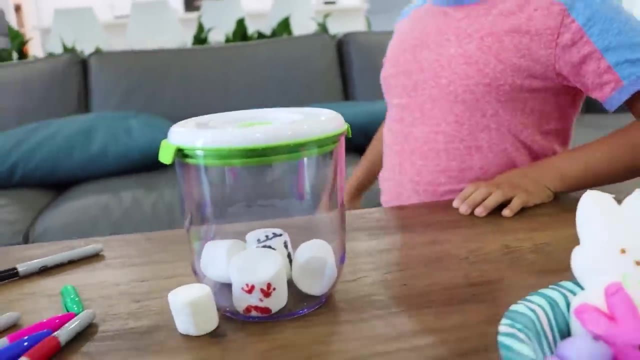 It got bigger. It expanded, Yeah, Yeah. So there it is. It actually got bigger. So here's what's going to happen when you unsuck the air. Are you ready? Okay, I'm going to open this. Okay, If you press this button, all the air will go back. 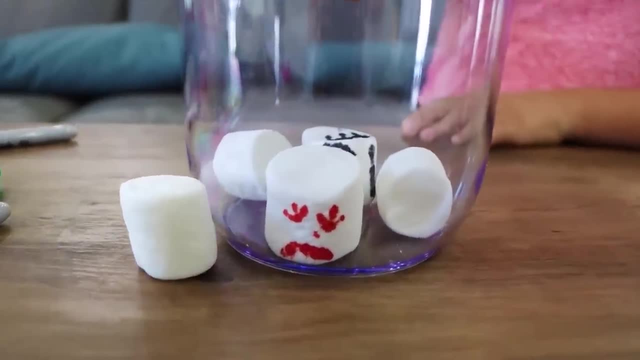 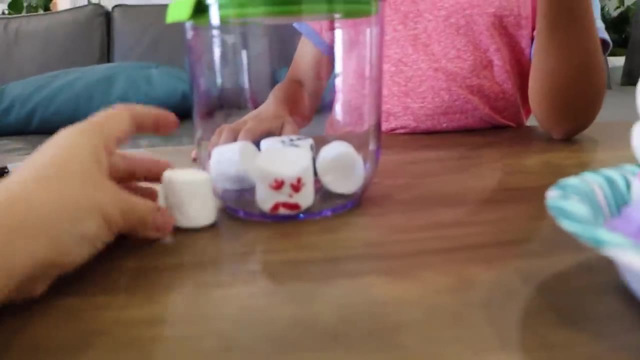 Oh, okay, Mm-hmm, What It became so much smaller. Yeah, Let's try that again. Okay, All right. So you guys notice here it's kind of it's the same size. Okay, All right, Go ahead. 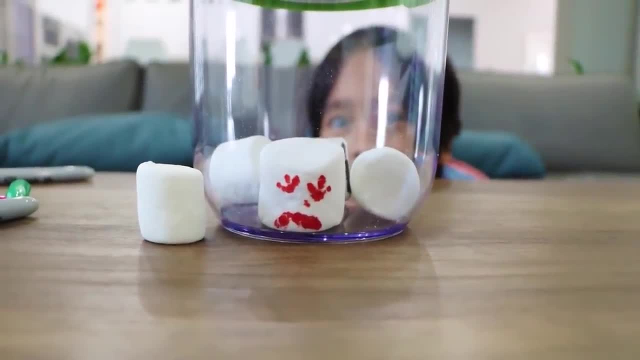 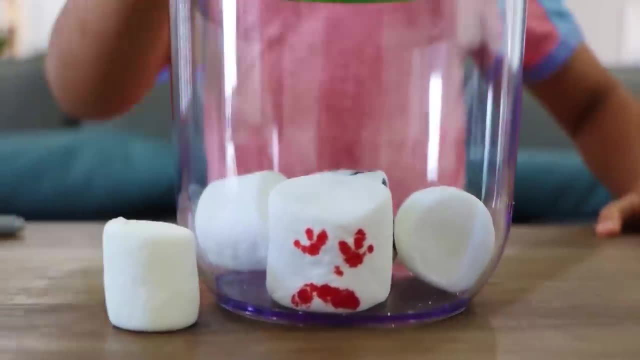 Vacuuming itself, Vacuuming. Oh boy, Oh, Do you guys notice it got bigger? Oh yeah, You just put yourself in the same spot. Yeah, Okay, Ryan's going to press the button again In three, two, one. 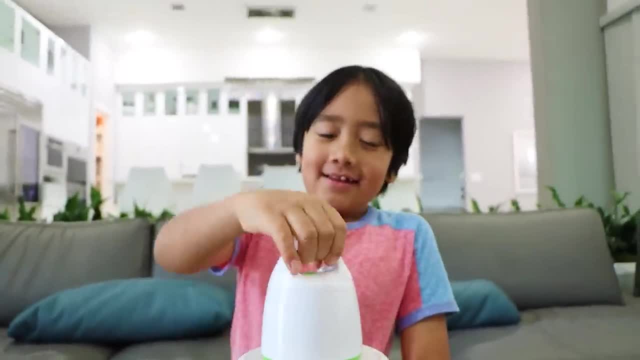 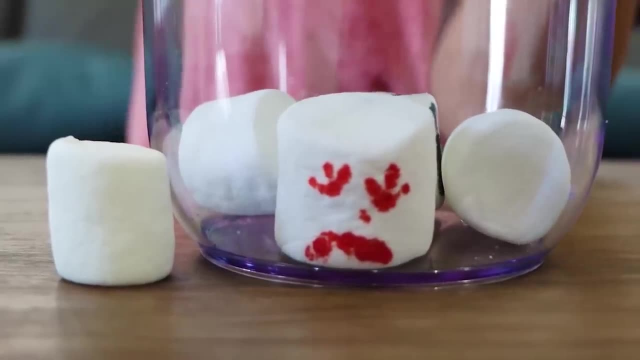 Whoa, Whoa, It got smaller again. So what actually happened with the marshmallow in the vacuum? That it became bigger? Oh, but do you know why? Why has it got bigger? Why, If you're sucking out all the air, why does it become bigger? 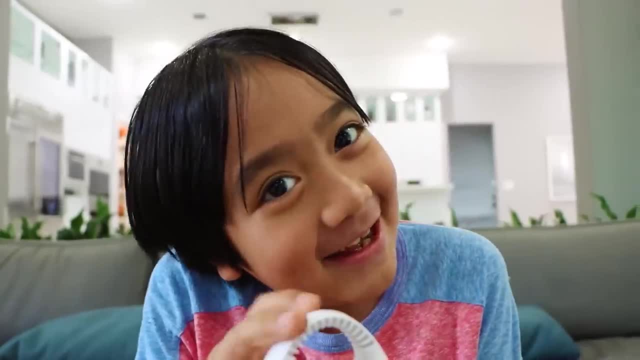 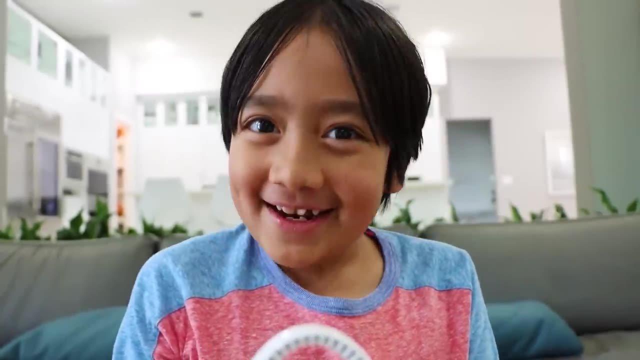 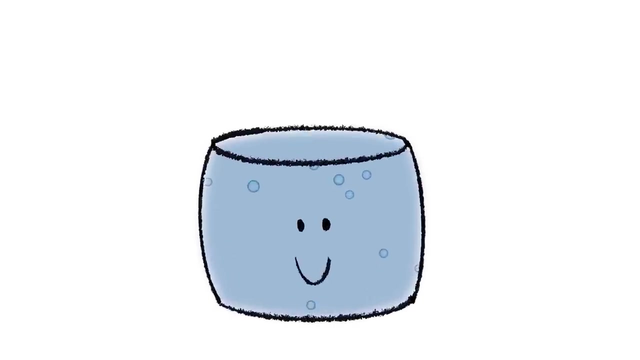 Any hypothesis, Any theory, Because the air is gone, That the air is gone Because the air is gone, Yeah, Okay, guys. So here's what's actually going on. Did you know that there are air bubbles inside the marshmallows? 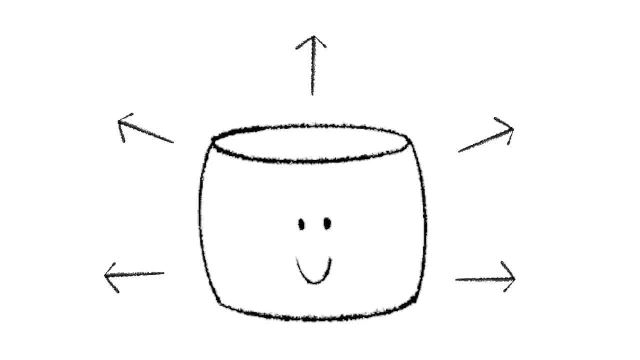 that moves around and push air Out onto the marshmallow. There are also air pressure from the atmosphere outside pushing in to the marshmallow. So the air from inside the marshmallow pushing out versus the air from the outside pushing in. This battle of the air keeps the marshmallow at the same constant size. you see now. 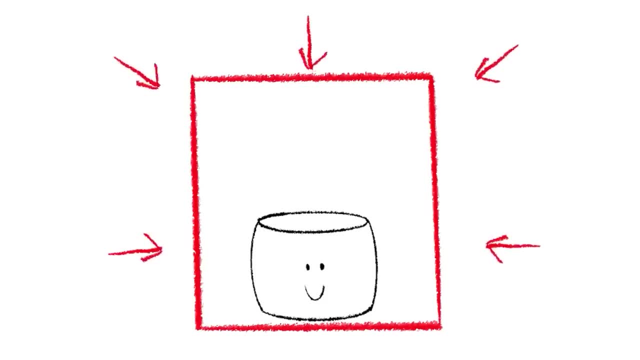 However, when you take out all the air outside, all the air inside of the marshmallow away, then the air inside of the marshmallow that's pushing out wins. That means the marshmallow will expand and become bigger. However, when you let the air back inside, 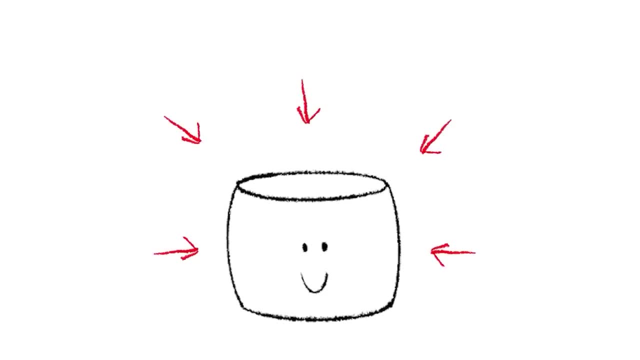 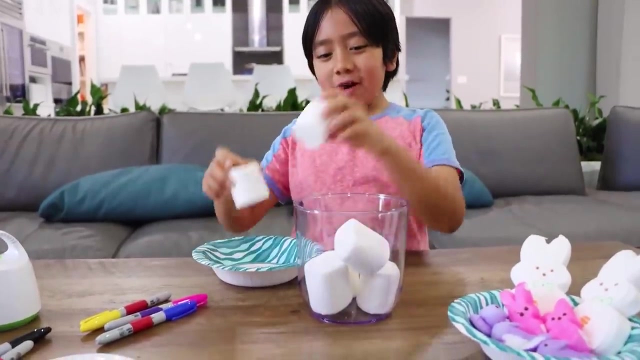 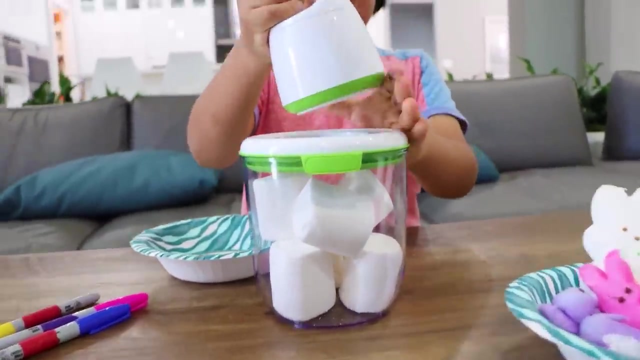 now the outside air will push back onto the marshmallow again, So it becomes normal size. Okay, so now we're going to try with giant size marshmallow- Giant size marshmallows. Okay, here's the cap. Okay so. 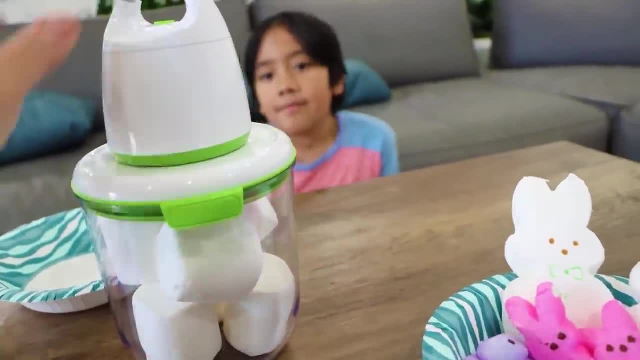 Oh wait, Can we take one out? That way we can see the original size. I think, Okay, so we're actually going to keep one out so you can see the size. See Same size right now. Three, two, one. 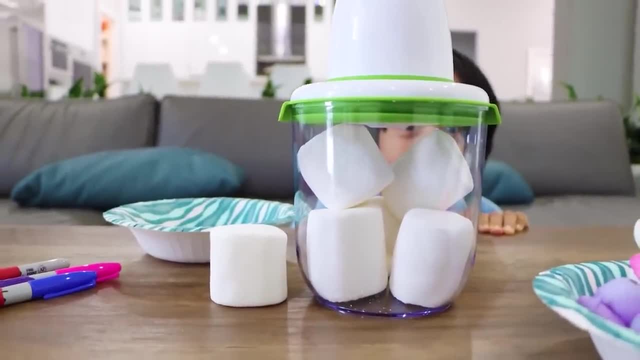 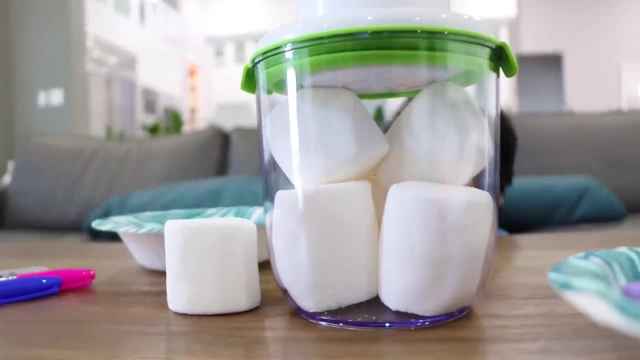 Oh, it's getting bigger. Oh, one of them is going to reach the top. Oh, it reached the top. Oh yeah, there's some space up there. Oh, do you guys see It's getting so much bigger, Do you see? 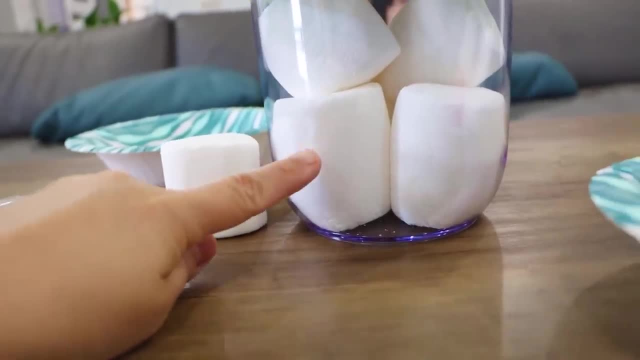 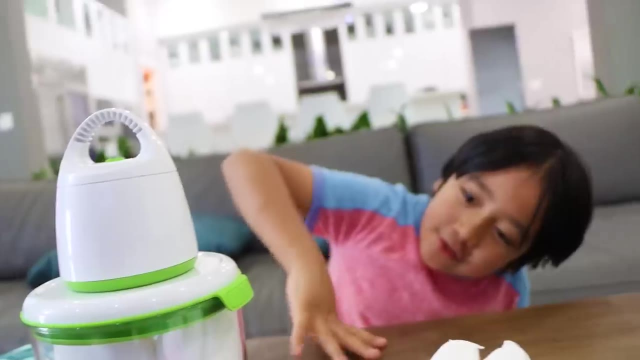 That's crazy. Look, That's the original jumbo size and that's the super jumbo size. Wait, when we make it bigger, one of them, or two of them, is up against the roof. so it's like: ooh, so it's going to stay like that when we put it back. 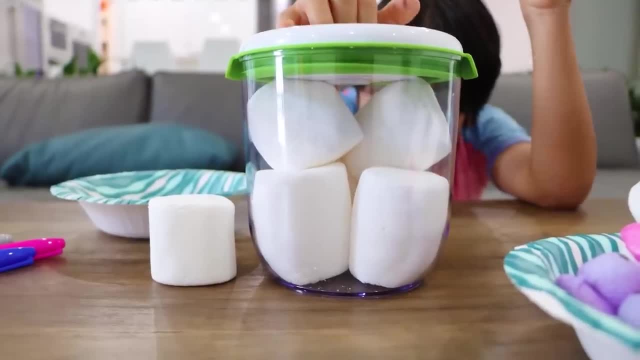 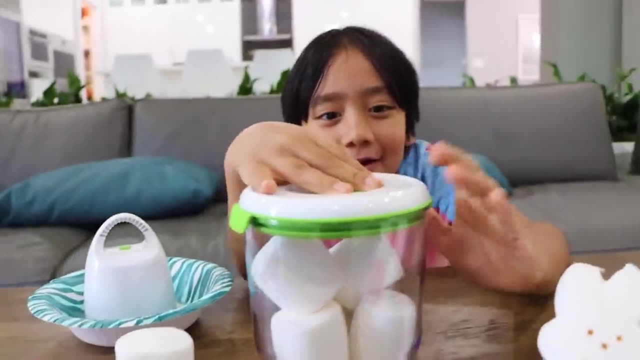 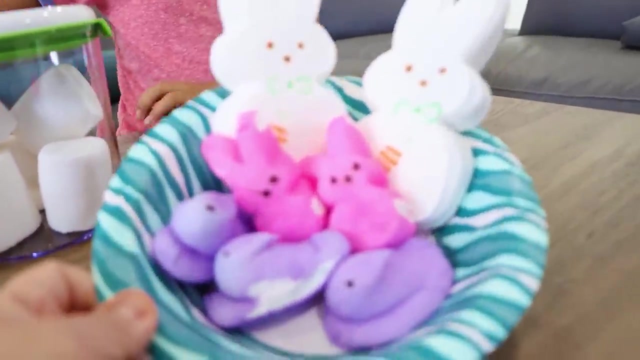 Let's see what happens. Okay, let's see Three, two, one Small mode: Whoa, Did you see that? Yeah, That was really cool. Yeah, that was so cool. Okay now bunnies, Are you guys ready to be jumbo size? 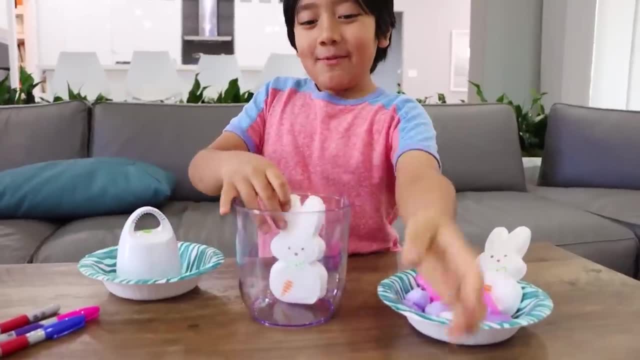 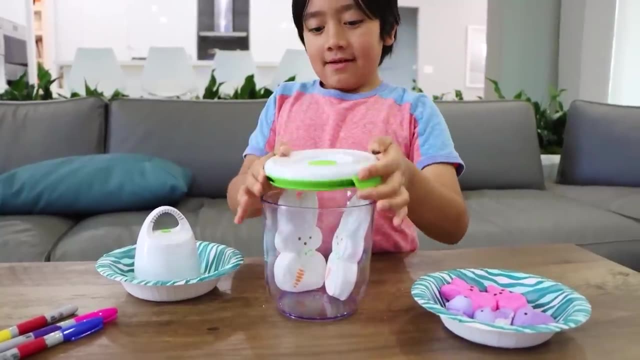 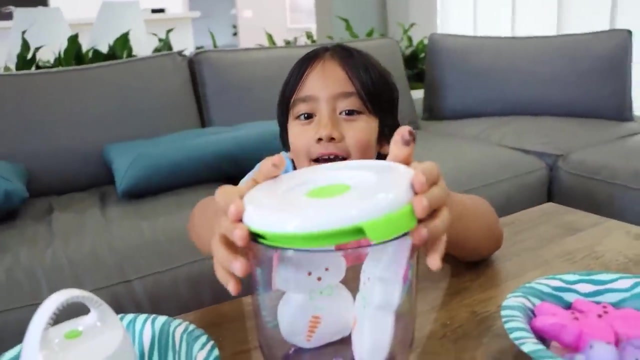 And then small-o size. Okay, we're going to try one big bunny. Do I need two big bunnies? Okay, Wait, this might. What will happen? There's no space on top. Yeah, there's no space on top already. 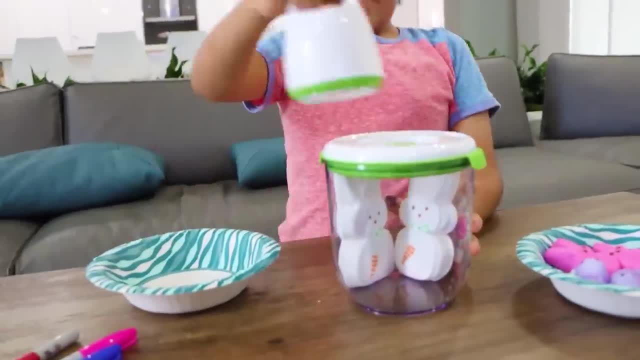 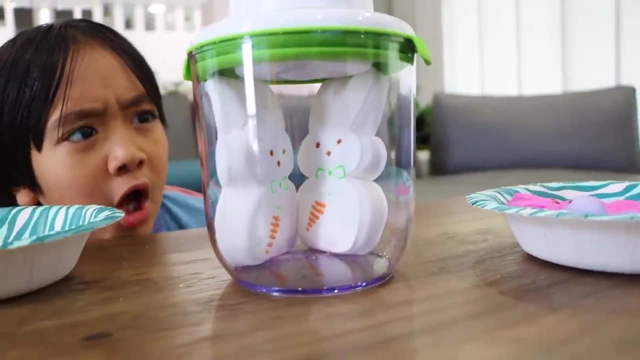 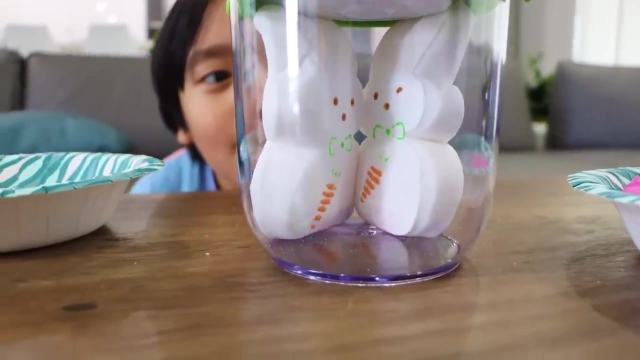 That's the fun of the experiment. Get to see what happens. Okay, three, two, one. Okay, Can it become bigger? It's getting bigger. Do you guys see it's becoming bigger? Oh yeah, it is. Look they're getting closer together. 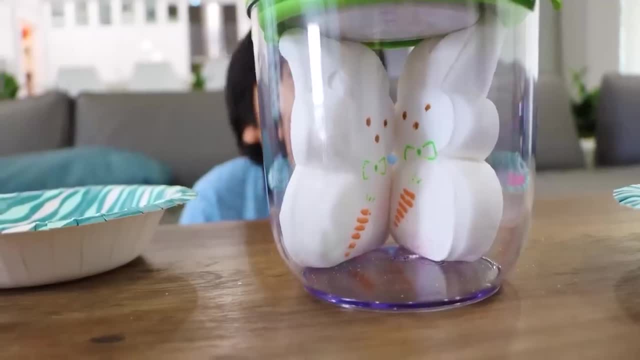 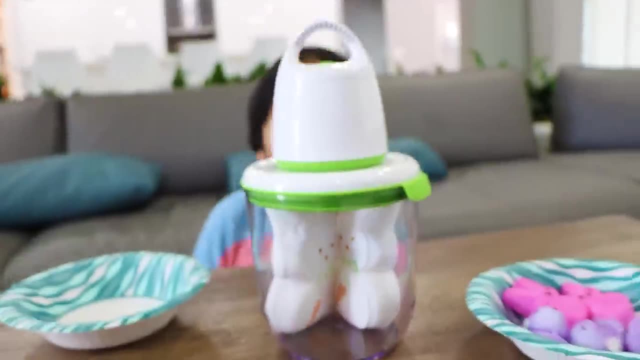 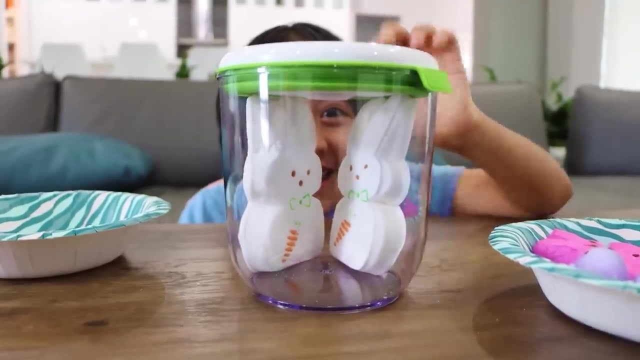 Bam, they're touching now. I know they're touching now. They're friends now. Hi Hi. Okay, Ryan, you ready to let the air back in? You can't see me through this Now you can. Whoa, you guys see that. 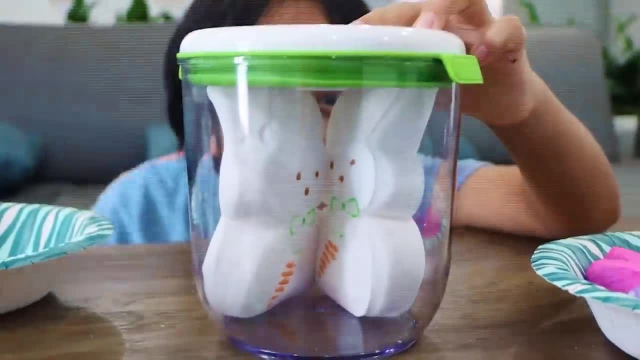 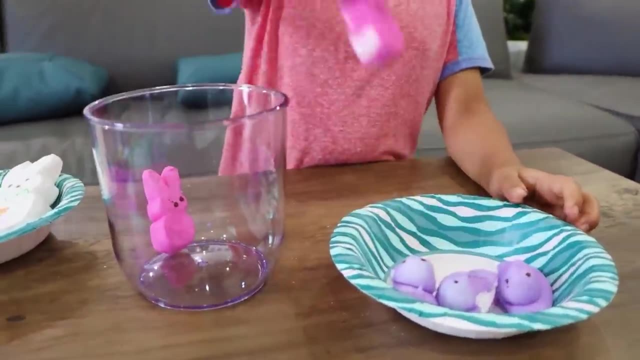 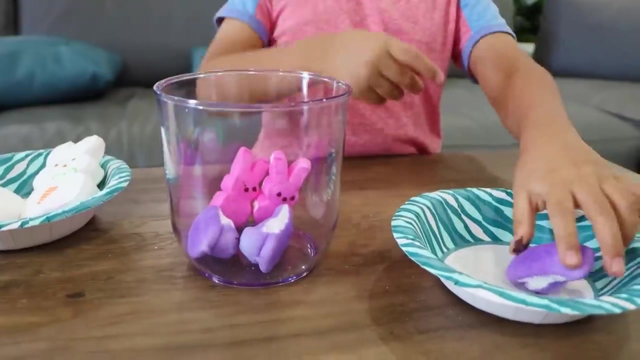 Alright, guys, instant replay. Now you see, Now you also see. Okay, we're going to put these all together. Oh, oh, oh, Baby bunnies And some baby chicky chicks, Bam-a-bam, Bam-a-bam. 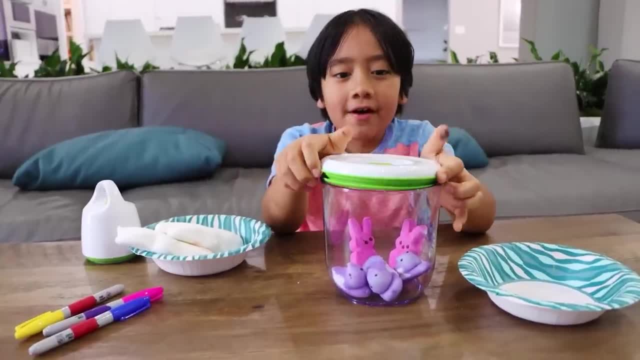 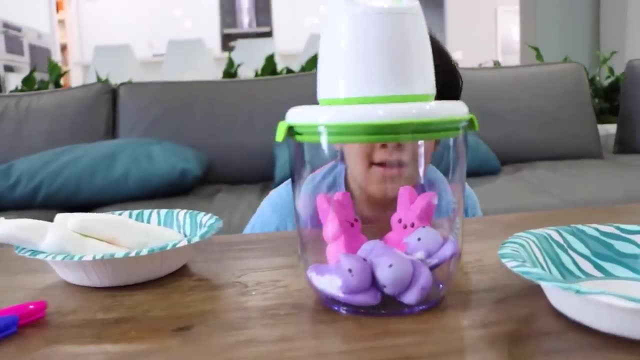 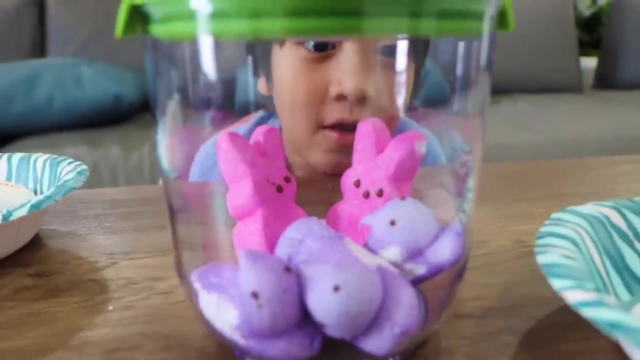 And bam-a-bam. Okay, guys, we're going to put it on Bam And then we put no air Vacuum. Vacuum the air out, Air the vacuum out. Oop, Did you guys see it got bigger? Is it getting bigger? 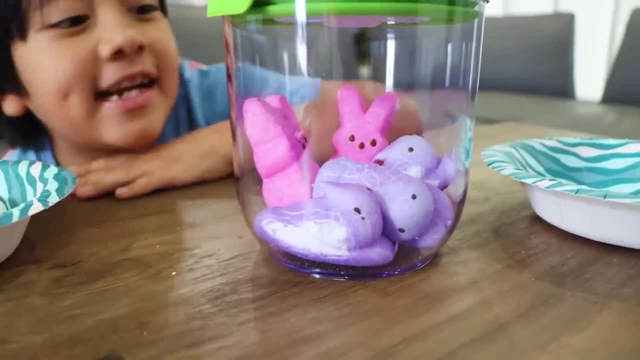 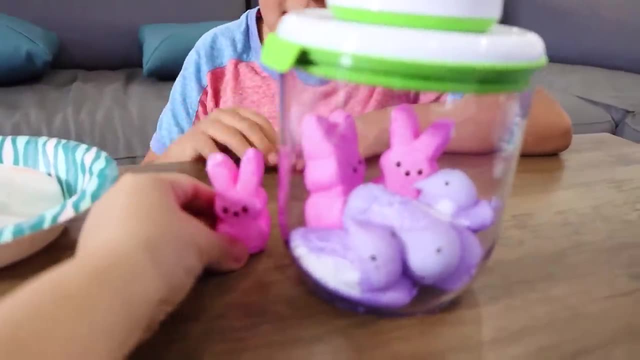 Yeah, it's getting a little bit bigger. Yeah, it's getting a little bit bigger. Yeah, it's getting a little bit bigger. Here's the original bunny. Did it get bigger? Oh, yeah, it got a lot bigger. Yeah, it got a lot bigger. 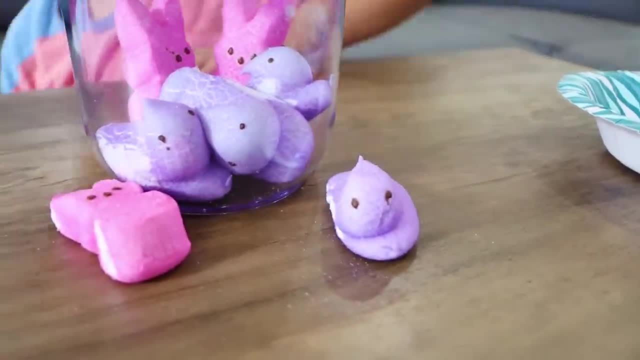 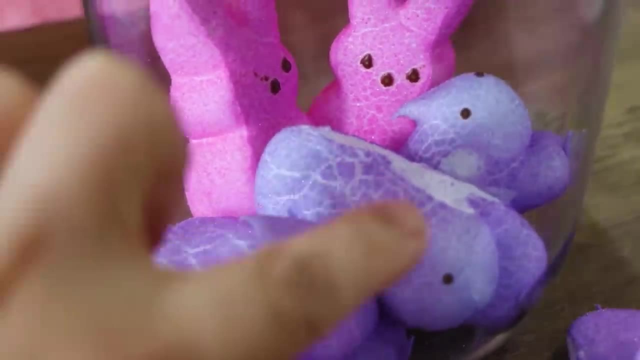 Here's the original chick here. It got a lot bigger too, because when you see it expand, do you see the little holes and cracks? Yeah, See, when it's trying to expand, you guys see the little cracks that it makes. Should we put the air back? 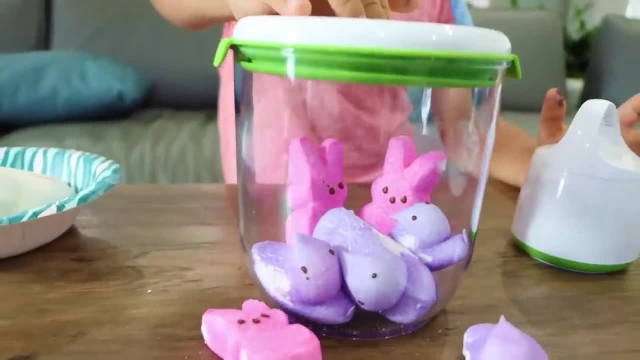 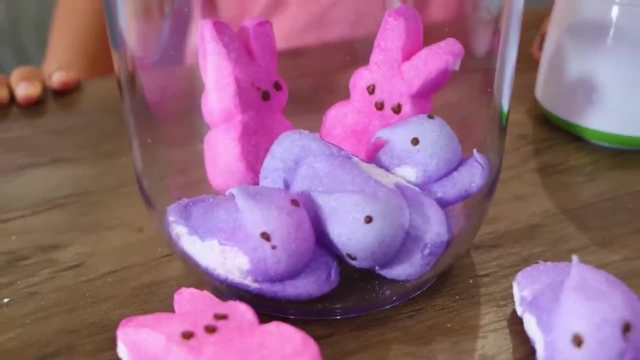 Yeah, let's put it back. Let's see how small it gets. Wait, the cracks are all gone. What really? Yeah, Let's see. Oh, yeah, that's crazy. Okay, I'm going to try it one more time, You ready. 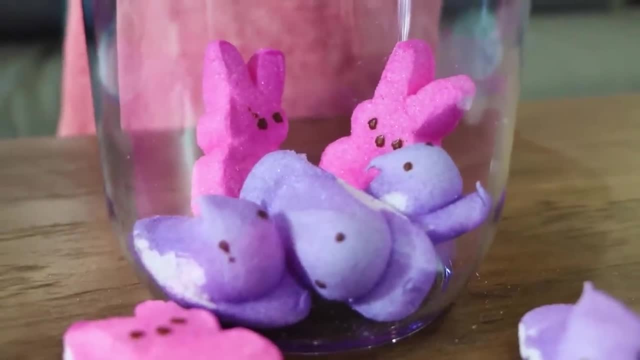 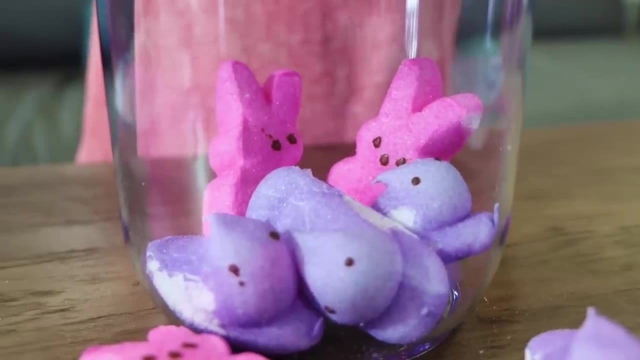 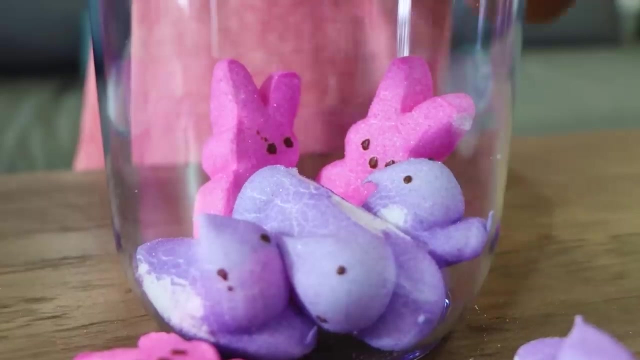 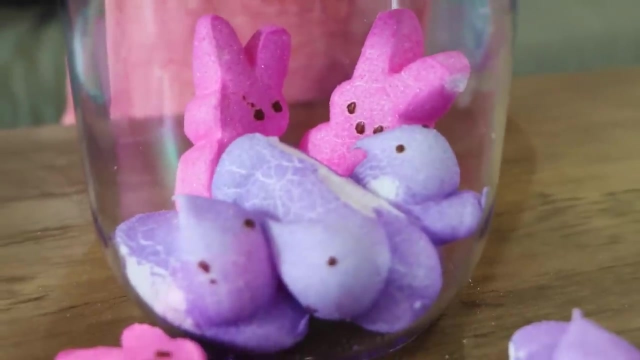 Okay, I'm going to do it super still. Okay, go ahead, Press it for me. Whoa, Do you guys see it expand? Look, it's starting to get some cracks. Oh yeah, see the cracks guys. Okay, undo it whenever you're ready. 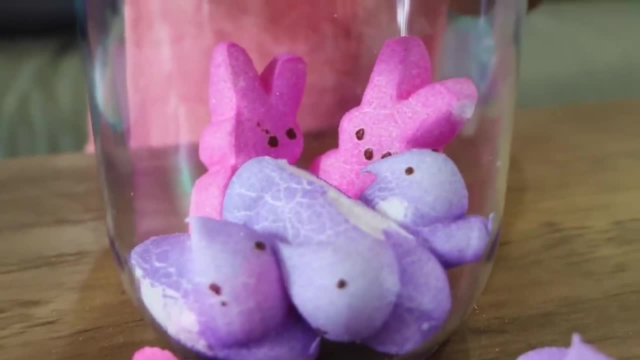 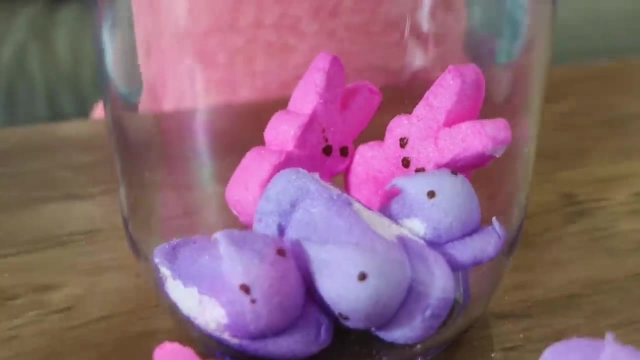 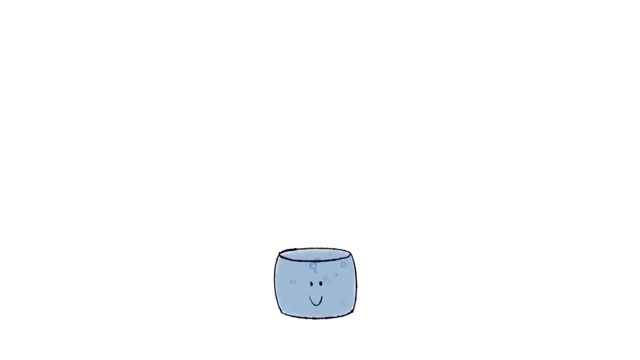 Okay, right after this one. Okay, And cracks, No cracks. Whoa, that was so cool. Yeah, And here's a recap of why it happened. Row the clip: Did you know that there are air bubbles inside the marshmallows that moves? 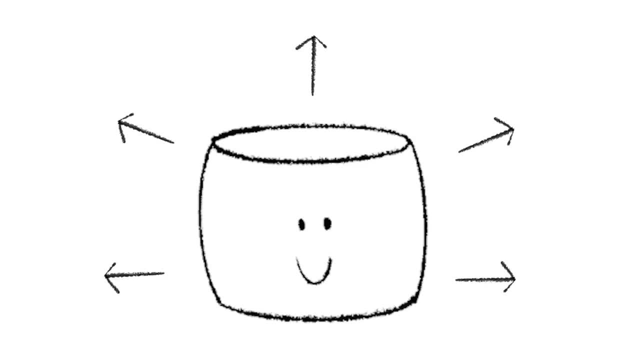 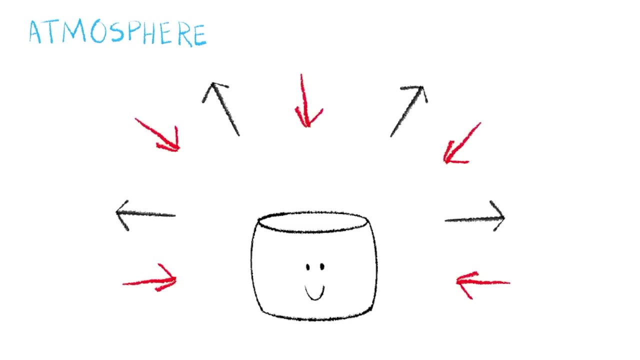 around and push out onto the marshmallow. There are also air pressure from the atmosphere outside pushing into the marshmallow. So the air from inside the marshmallow pushing out versus the air from the outside pushing in. This battle of the air keeps the marshmallow at the same. 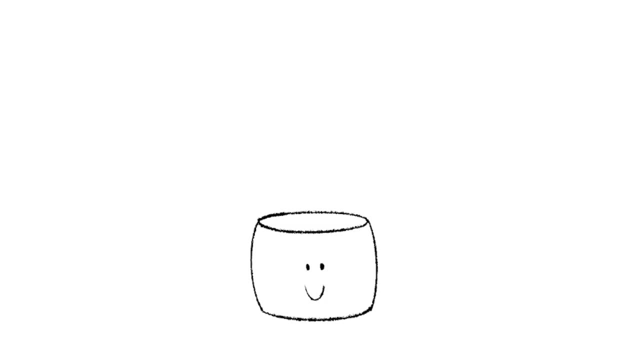 constant size. you see now, However, when you take out all the air outside of the marshmallow away, then the air inside of the marshmallow that's pushing out wins. That means the marshmallow will expand and become bigger. However, when you let the air back, 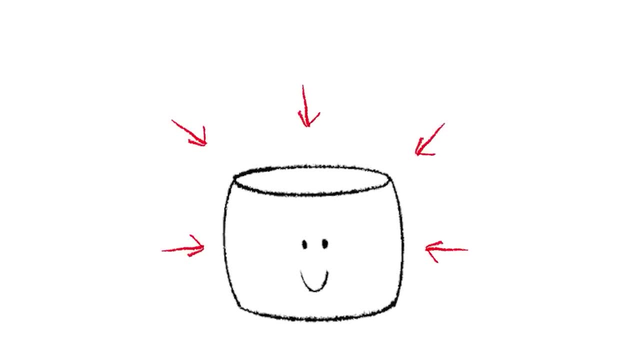 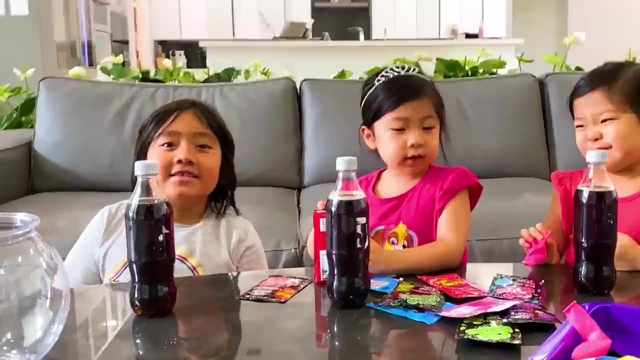 inside. now the outside air will push back onto the marshmallow again, So it becomes normal-sized marshmallow again. Thank you for watching my marshmallow in a vacuum experiment. Hi guys, Today we're going to blow out balloons with rock, candy and coke. 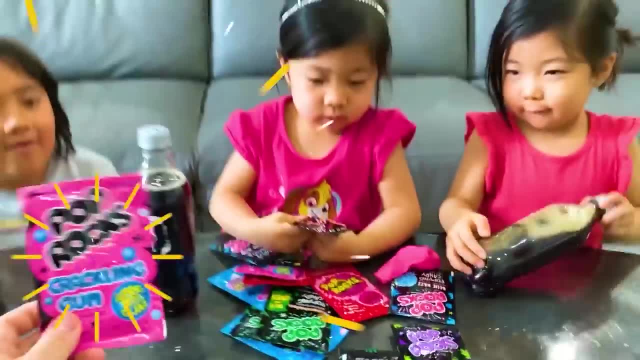 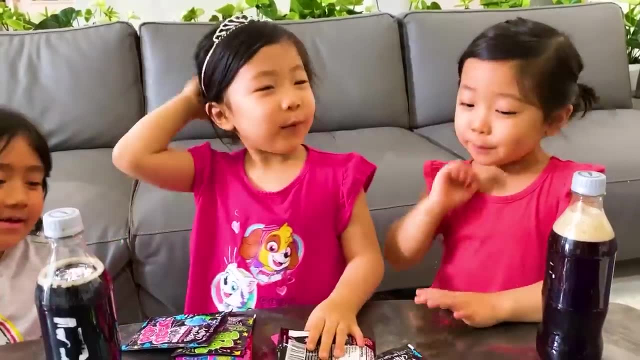 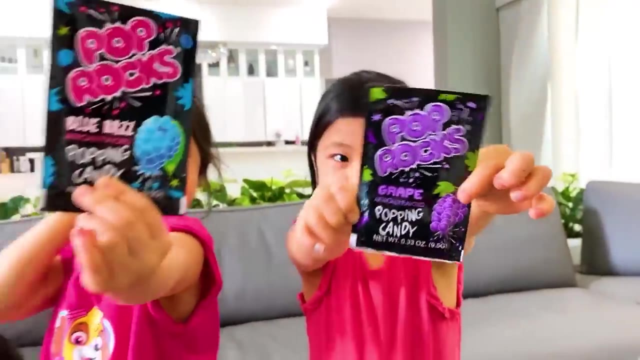 So we got a whole bunch of rock candy here. Have you guys ever tried rock candy before? No, You have. No, Do you want to try it? Yeah, Okay. so which flavor do you want to try? I want this one. 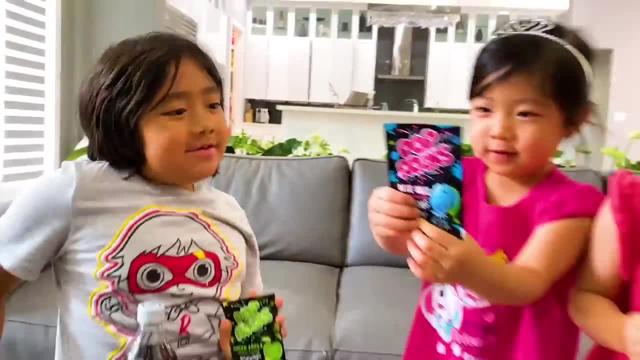 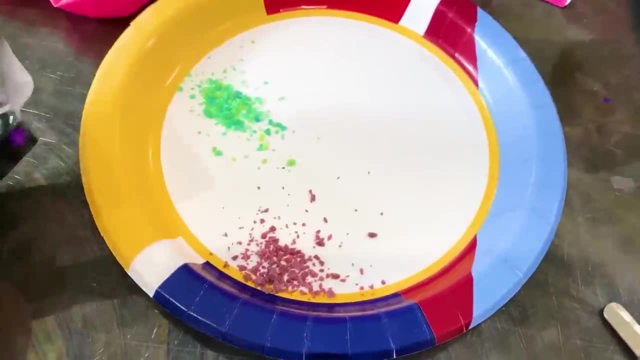 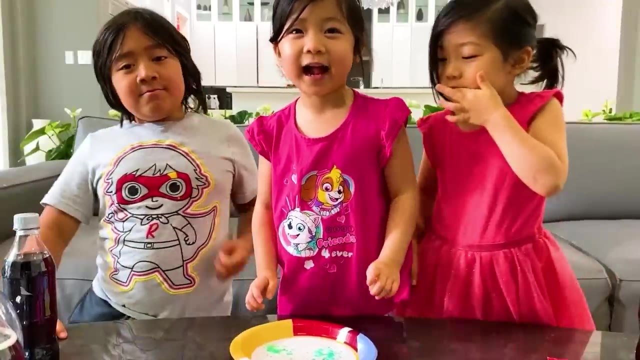 Okay. so Emma wants to try blue, Kate wants to try grape And Ryan Green apple. Okay, some green apple there, Some grape Green And some blue Blue. Can I try, Ryan, And you don't have to chew? 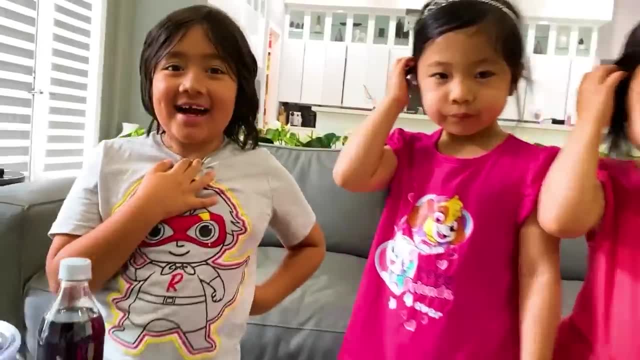 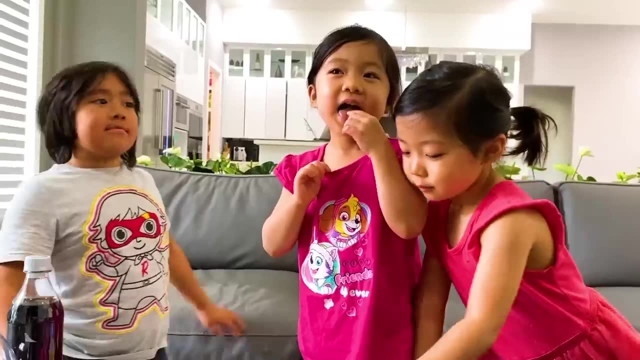 Just put it in your tongue and it's supposed to pop. Tell me if you feel the pop, Do you? I hear it too. Do you feel the pop? Yeah, just put it in your tongue and just keep it there And close it. Close your mouth. 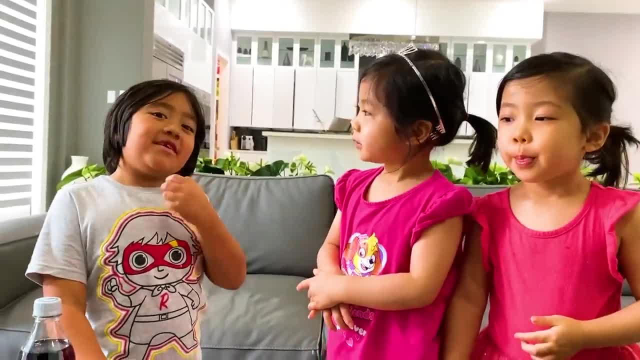 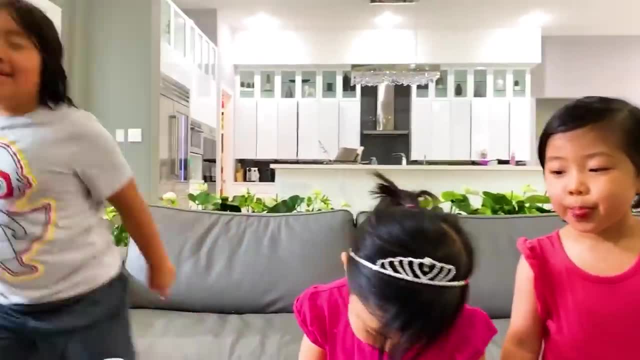 Whenever I eat it- and I do this- I hear a lot of pop. I know Well, what do you guys think? Do you guys like it? Don't like it. Weird, You like it. I don't feel the pop. 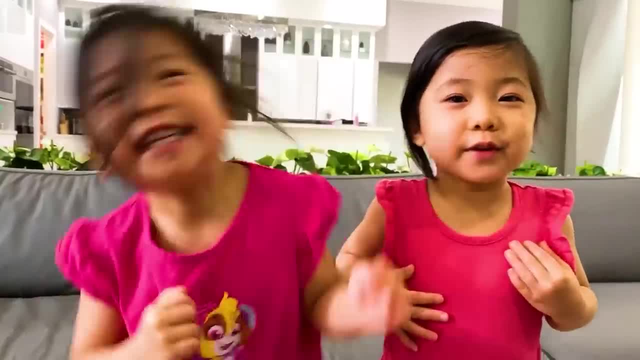 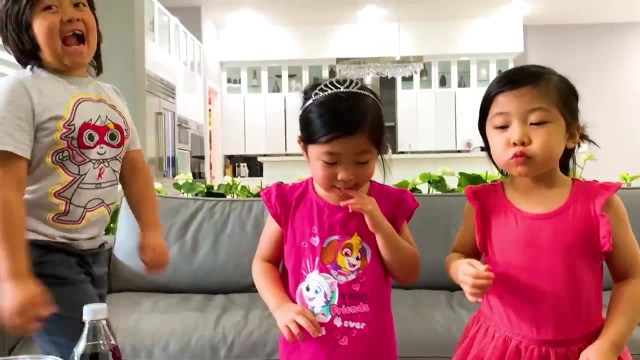 I don't feel the pop. You don't feel the pop. What about you, Emma? Yes, Okay, you guys ready to blow up some balloons? Yeah, Okay, actually, before we try to pop a balloon, we're going to see what it looks like with the Coke. 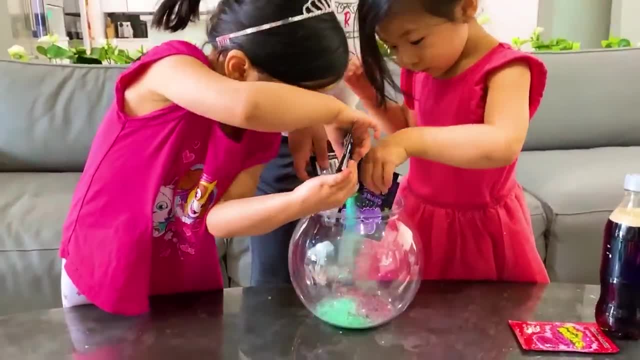 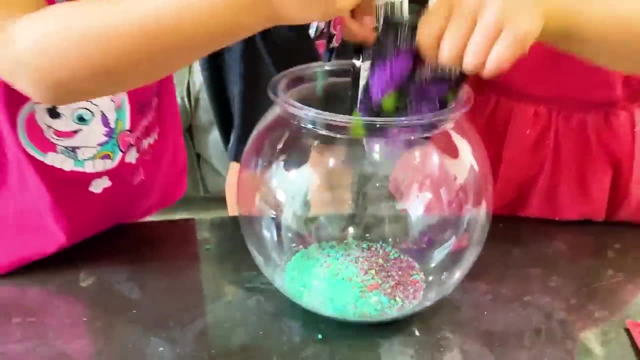 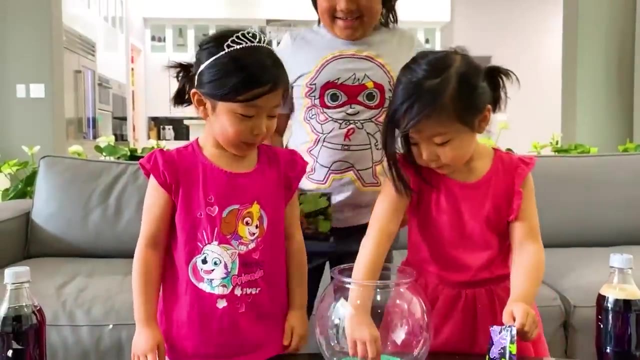 Okay, so everybody pour in their rock candy. Whoa, All of them. Yeah, all of them, All of them. There you go. There's a lot of green, I know, Emma, Stop, Okay, so now we're going to try the Diet Coke in there. 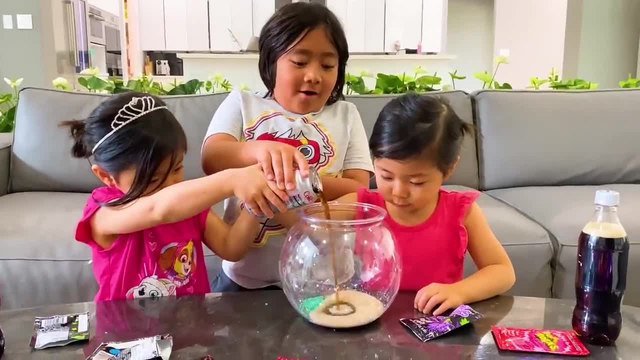 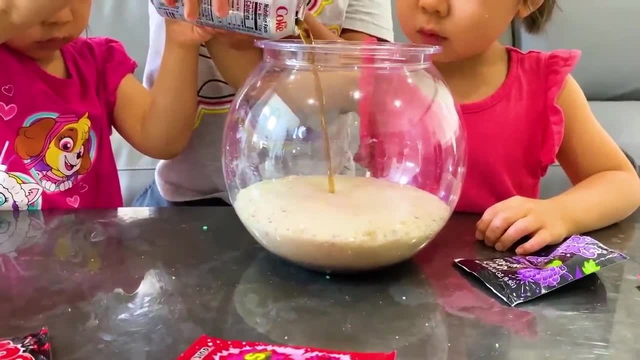 and see what it looks like. Whoa, Whoa, that's a lot. We're going to eat it. I know we have a lot more. I don't know if we need that much. Okay, Wait, it's kind of changing. 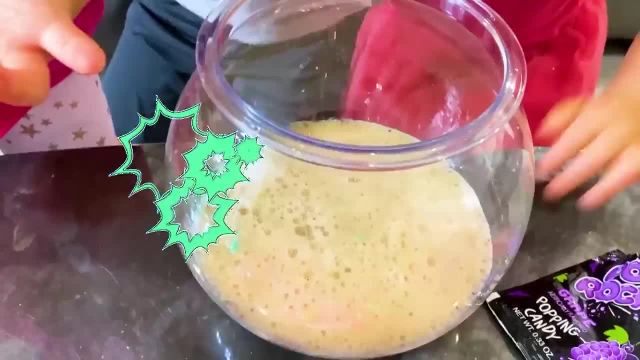 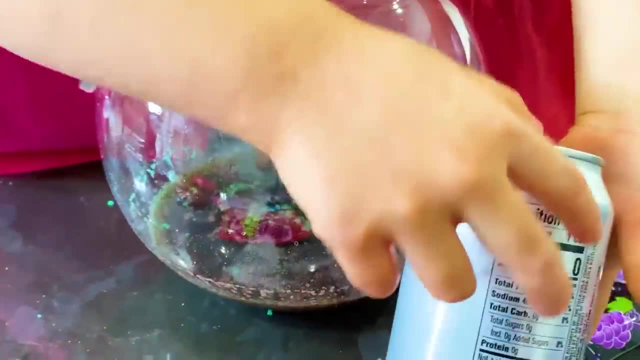 different colors. the Diet Coke: Do you see the pop in there? That's too much Diet Coke, Not too much you guys. Do you guys hear the popping sound? Yeah, Whoa, it's popping. I want to put up more. 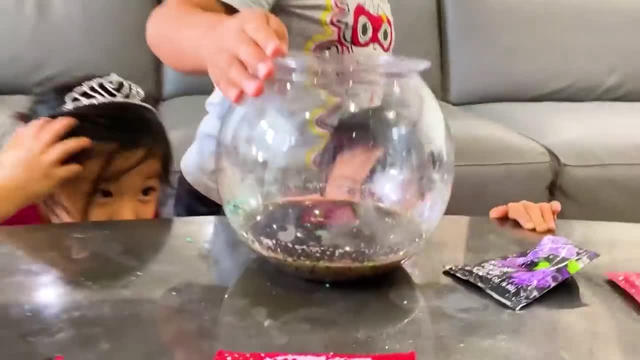 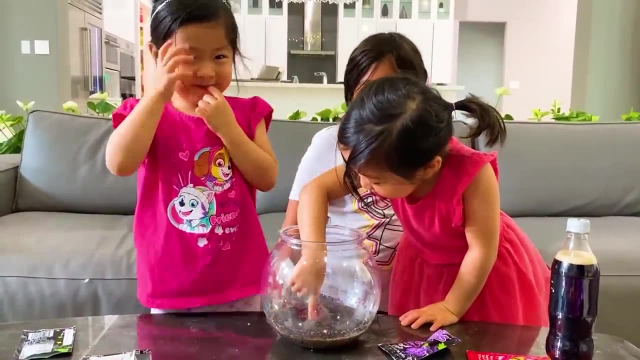 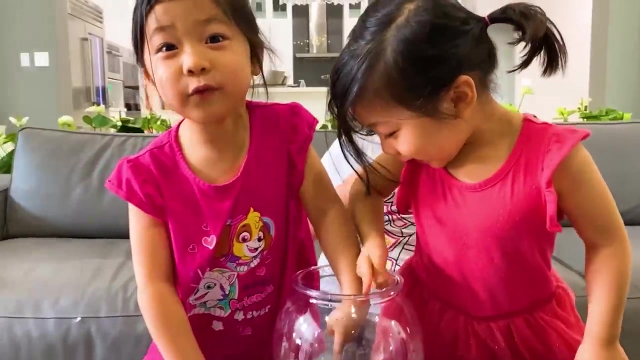 Do you see the popping? Thank you, Melanie. How does it taste? How does it taste? It tastes good, Does it? Yeah, Okay, just one little taste, Thumbs up, Thumbs up. It kind of tastes like 1% of the taste of Sour Cots. 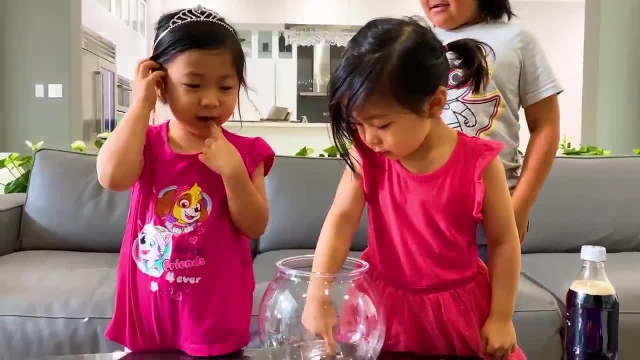 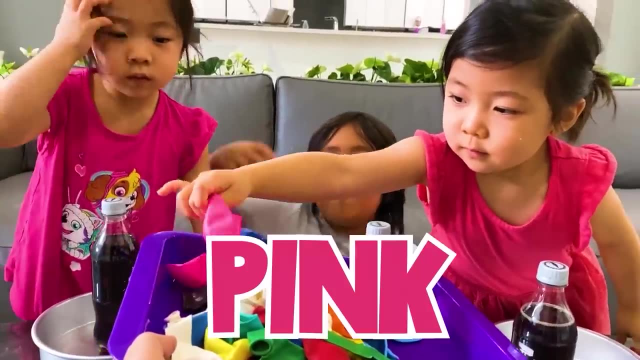 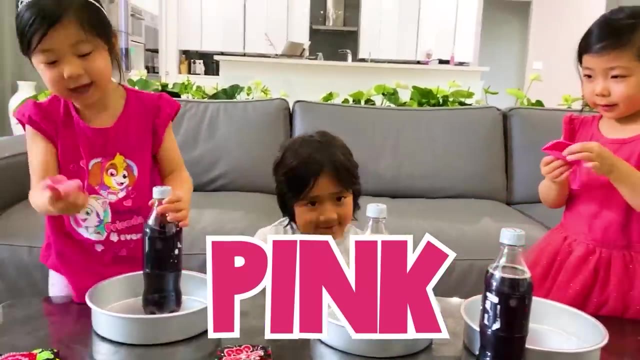 Really, Yeah, Sour, Interesting, Okay. so now we're really going to do this experiment. Okay, first you're going to pick your balloons Pink, blue and pink. Okay, change your mind. Okay, I like this pink. 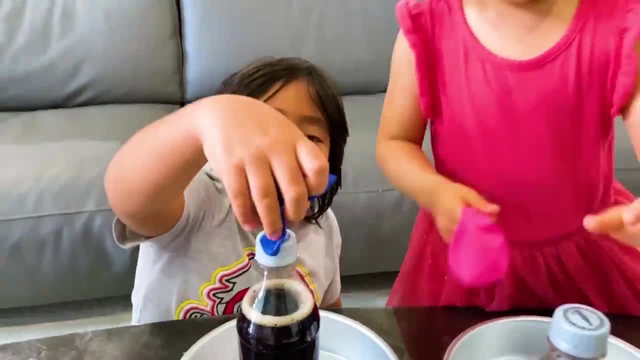 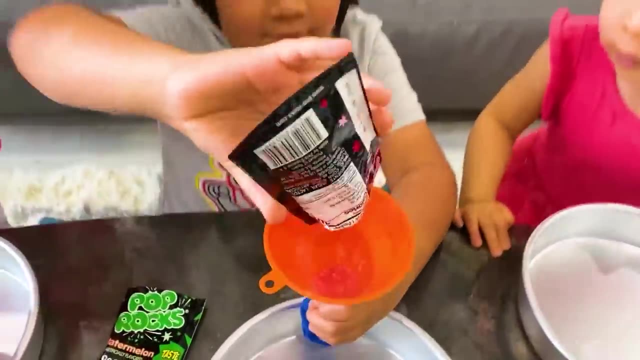 Got it. So first, that's right. Good job, Ryan. Yeah, Alright, we have a funnel to the balloon and Ryan's going to put the rock candy inside, like that. Okay, We're going to use both because we are courageous. 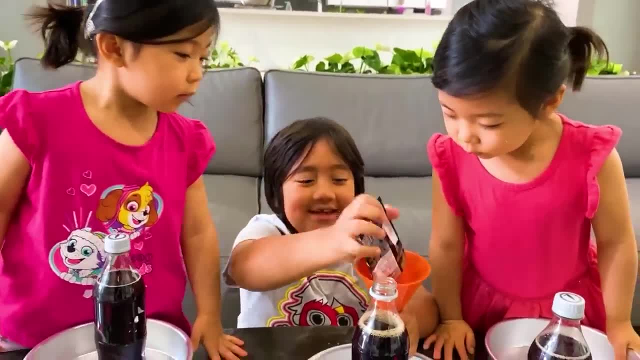 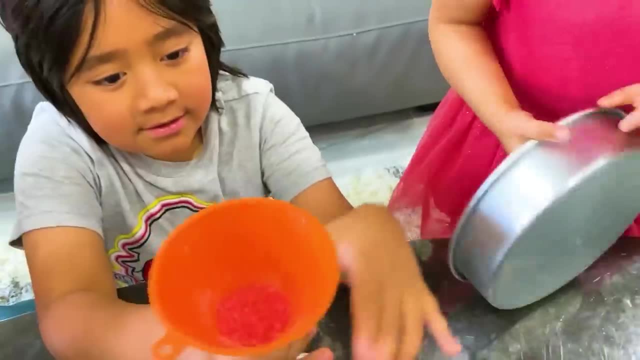 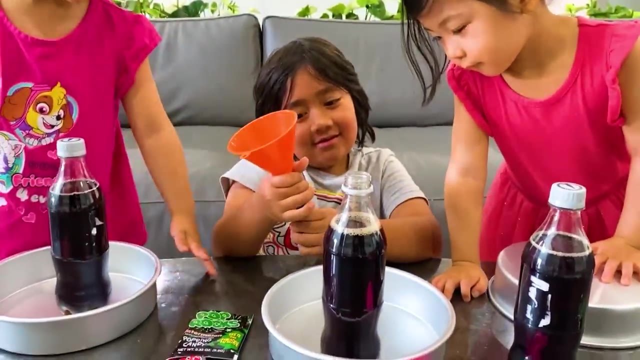 Yeah, Go big, or go home, right, Yeah, Go big, Go bigger. Oh, it's a lot Shake it, Shake, shake, shake. Okay, Ryan, here's for the hard part. Can you put your balloon over? 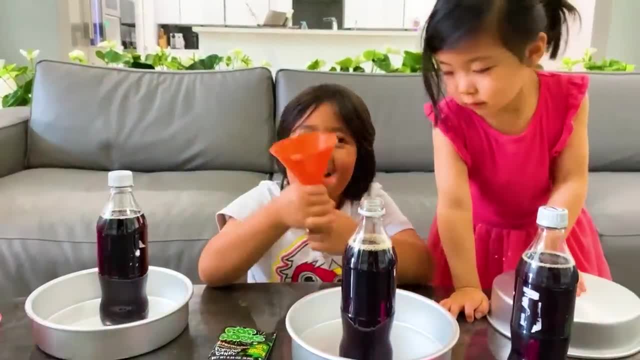 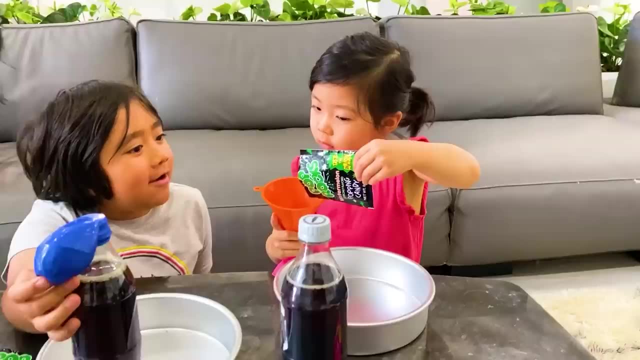 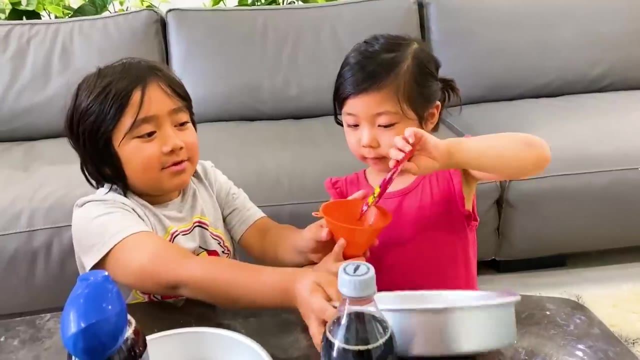 this without it going in. Yeah, Okay, You got it. Got it, Alright, Kate's turn. Oh, Good job, Kate. There you go, My turn. Yes, Emma, your turn. Yes, your turn Emma. 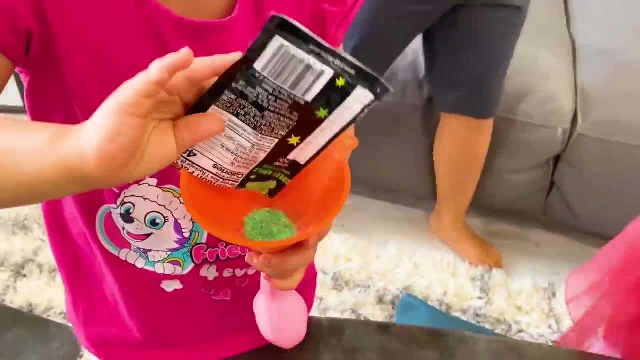 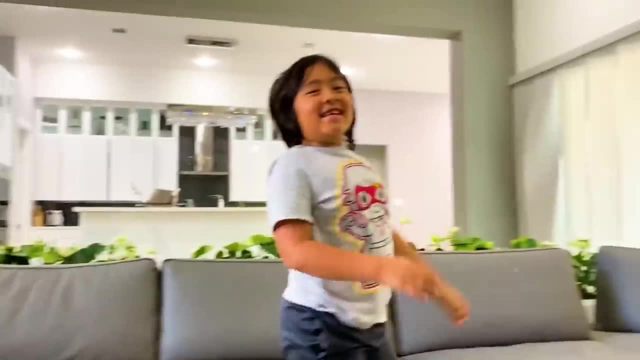 Okay, now Emma's turn, of course, But this time we need two. Yep, we're going to try two. Probably works with one, But maybe we can get a bigger balloon. Right Now we're going to put it down. 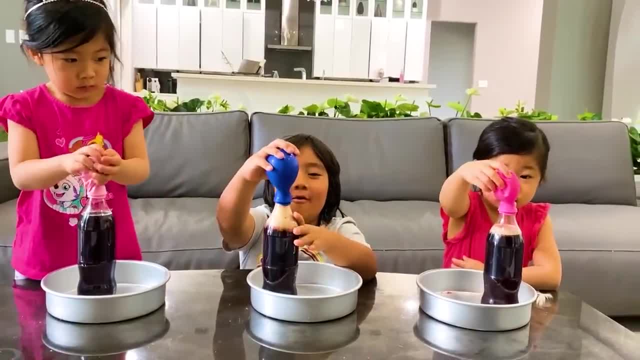 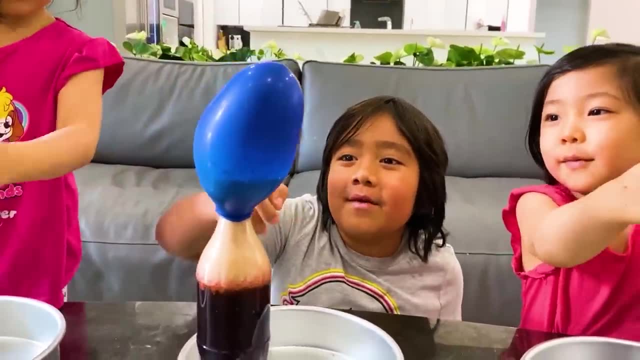 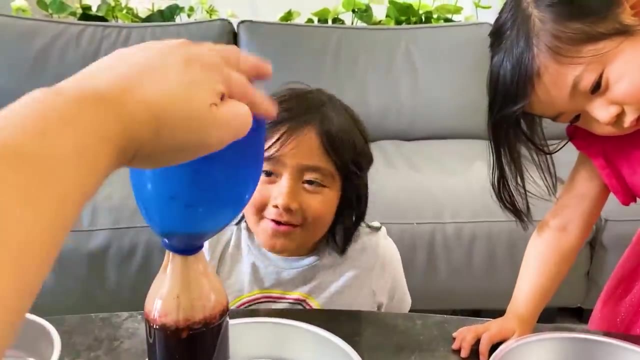 Three, two, one, Go. Whoa, whoa, The balloon is getting bigger. It's so big, Mine's bigger, Mine's more bigger, Mine is more bigger. Yours has a weird shape, Ryan. Emma, yours is working now. 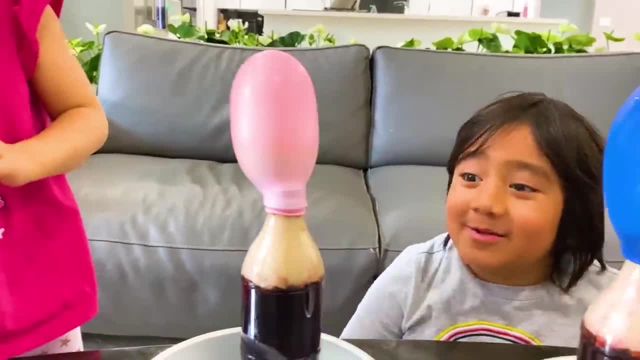 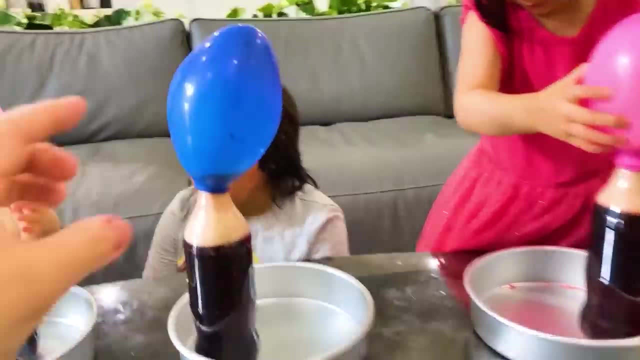 It's going down, Oh no, it's going down. It's going down here And these are going down here. Yeah, Oh, oh, I'm going to spill it. Oh, it's spilling. That's why we have a tray. 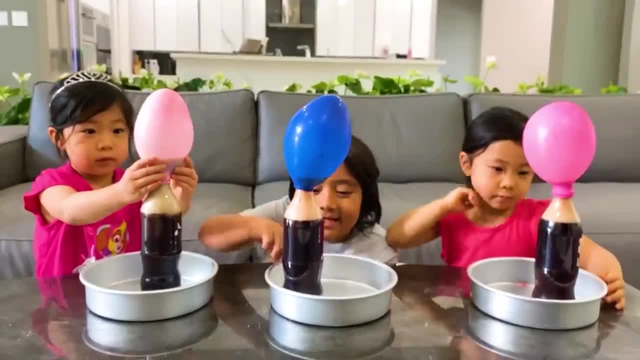 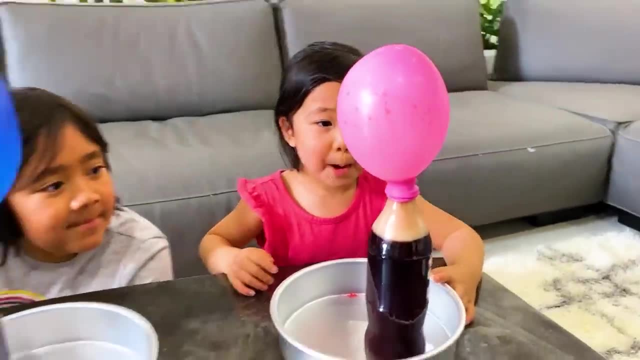 It's spilling a little bit, but it's okay. That's why we have a tray, you guys. I want to taste it, I want to taste it. I want to taste something else. Okay, when we're done, we can open it. 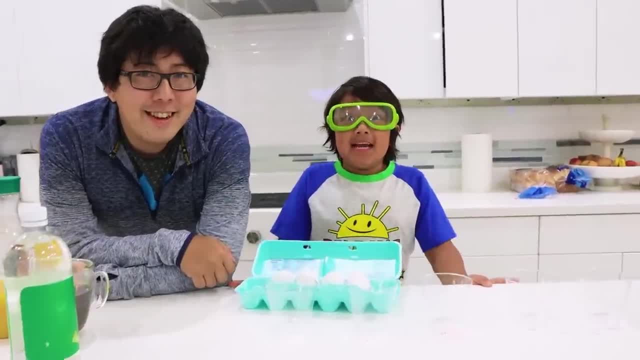 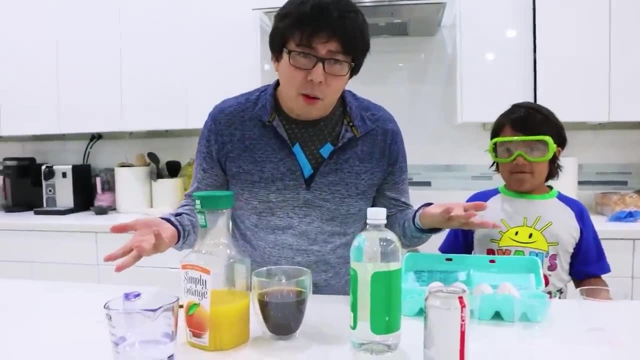 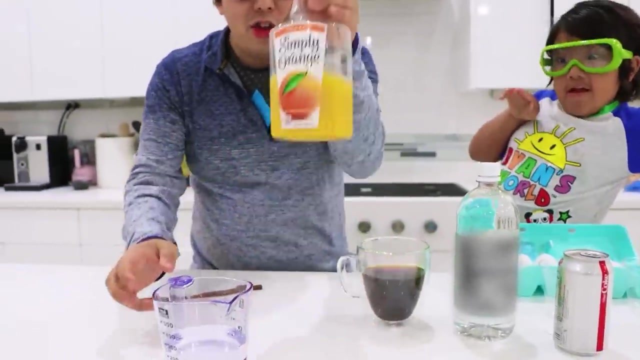 and you can taste it. Hey guys, today we're going to do a science experiment and see what happens to these eggs in liquids. We prepared so many different kinds of liquids. We got Diet Coke, vinegar, coffee juice, orange juice. 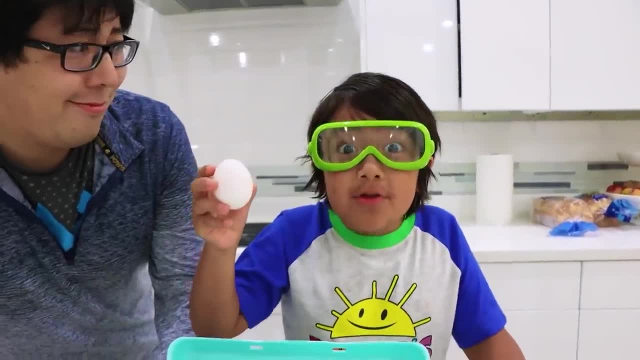 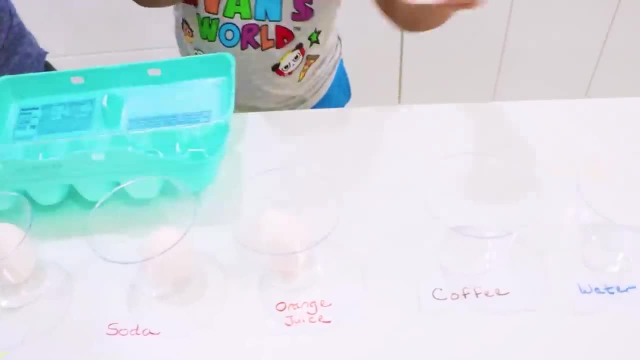 and water. Eggs are made up of a similar material as your teeth. We're going to put the eggs in each cup with the different liquids so we can test out and see what happens to the teeth if you don't brush it. This one says vinegar. We're going to pour vinegar. 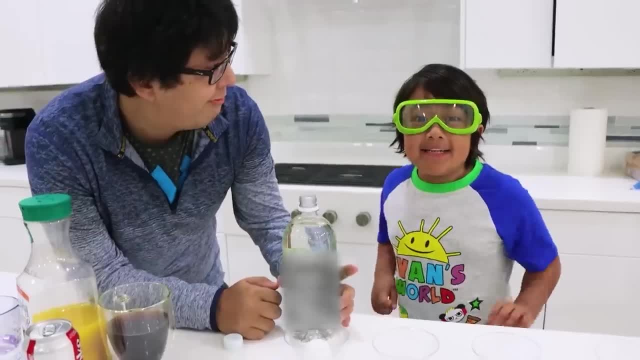 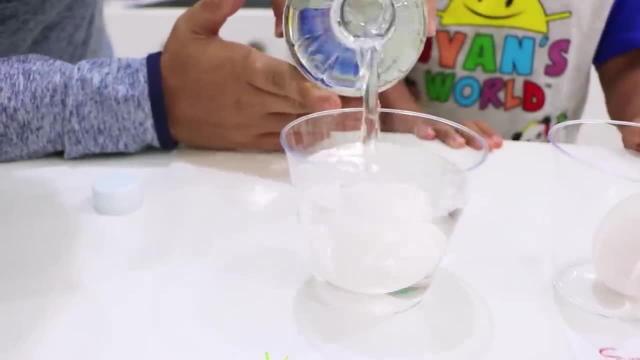 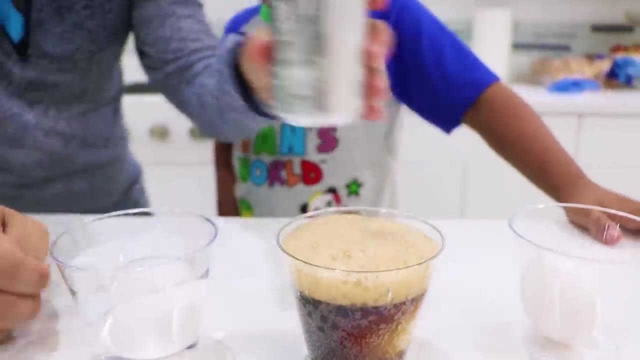 Alright, here we go. Daddy's going to pour vinegar. Let's see, Oh yeah, it does smell like vinegar. Alright, perfect. Next is Coke. Pour this into bubbly, Okay, all in. Next is orange juice. Oh, I smell it. 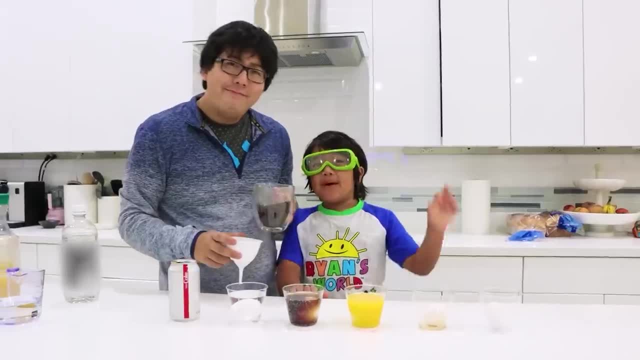 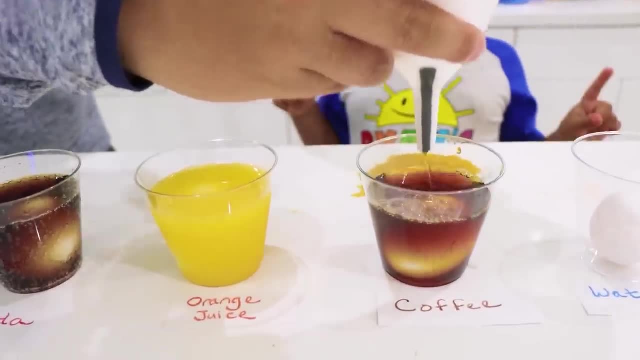 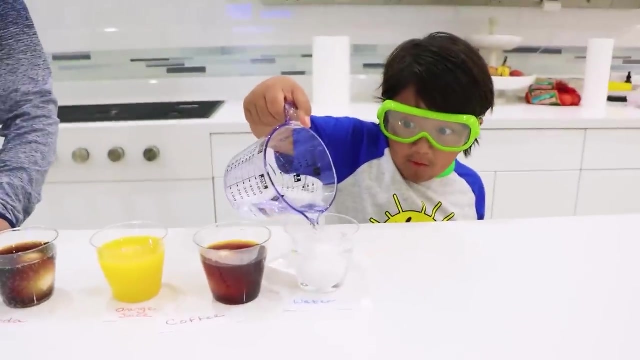 And the next one is coffee. Next one is coffee. Alright, here we go. Ooh, Coffee, Alright. Last is water Out of the way And good job, Boom. Now we're going to wait one day, See you soon. 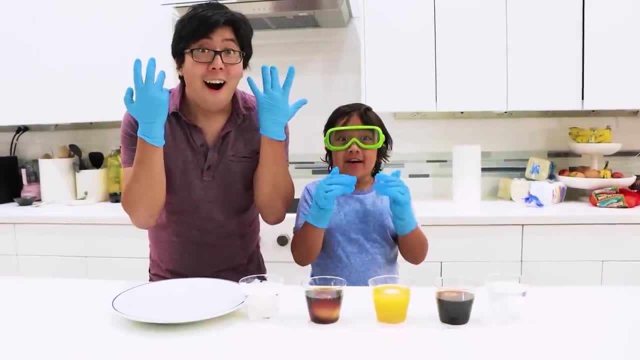 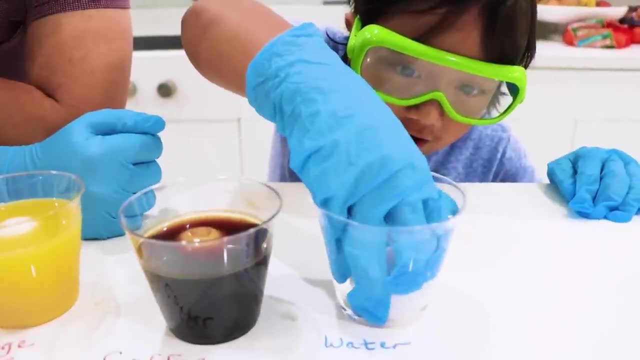 It's been one day now, And now we're going to check what happened to the eggs. Now we're going to start out with water, Carefully touch it, Ooh, Oh, it's the same. So the exact same. Yeah, nothing different. 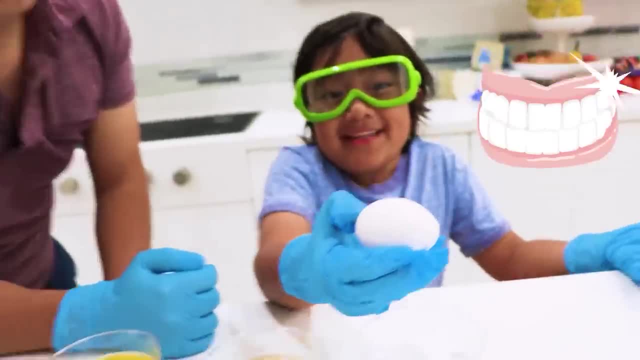 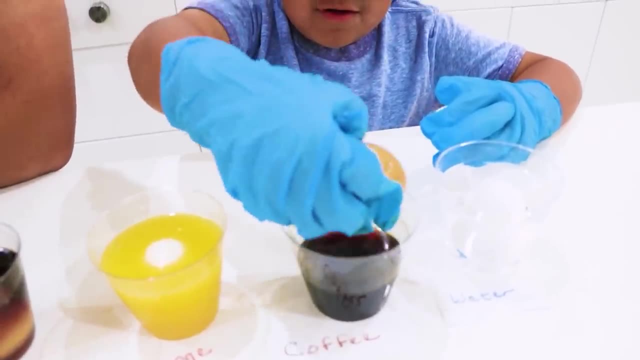 So if you put your teeth in water for a day, nothing happens, So water's good for you. Next, let's look at the egg in coffee. Oh yeah, I drink coffee all the time, So this is my teeth. I thought I'd brush my teeth. Look at it. 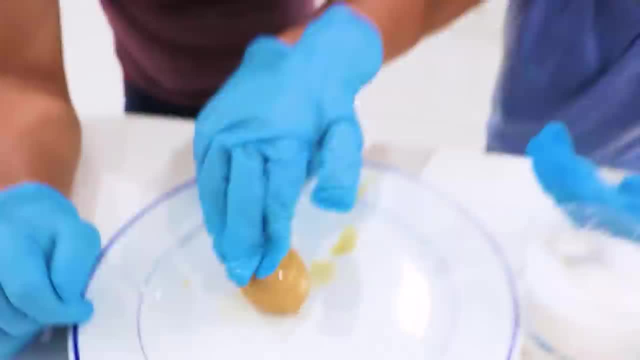 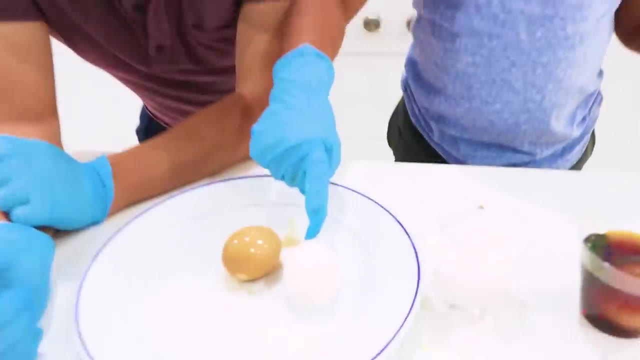 What happened to the egg, Ryan? It's brown. It changed the color. Look at it. So what happens if you don't brush your teeth after you drink coffee? It's going to turn brown- I know No more white. This is what a normal egg looks like. 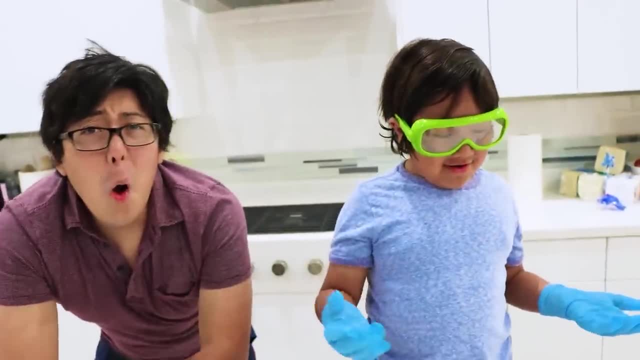 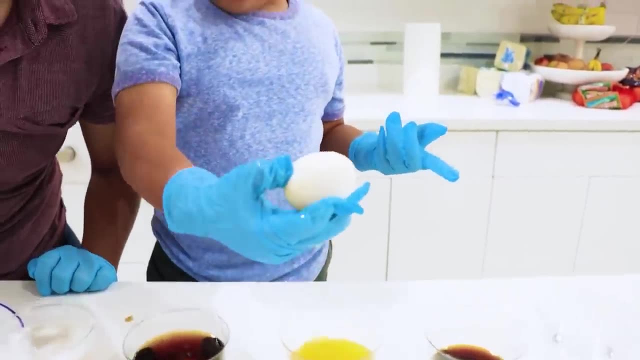 And this is what an egg in coffee looks like. Ew, No, Now let's try orange juice. Can't be orange, right Color? Let me see What. Oh, you see the bubbles that are on it, Yeah, but besides that, it's the same right. 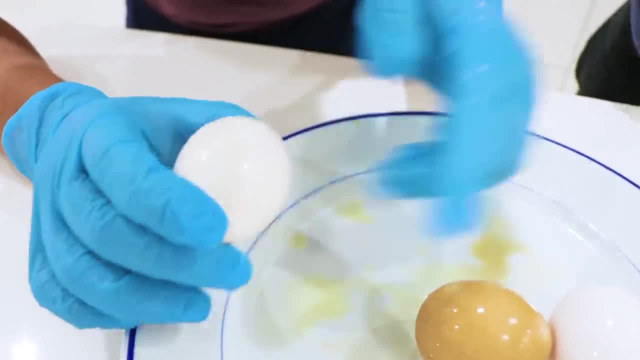 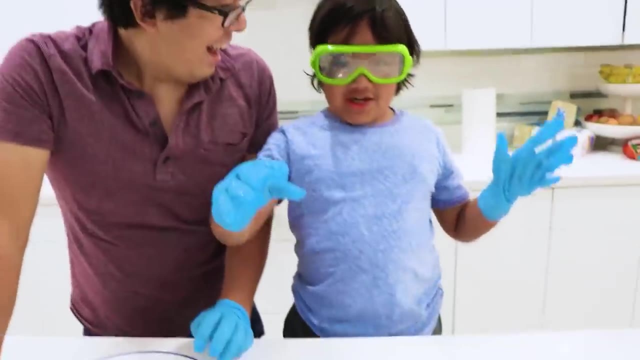 Don't forget, there's sugar on there too, So if you leave it for a while, it might attract bacteria and germs. Stop touching that. No, Now we're going to try soda or Coke. Oh yeah, We hear all the stories about soda. 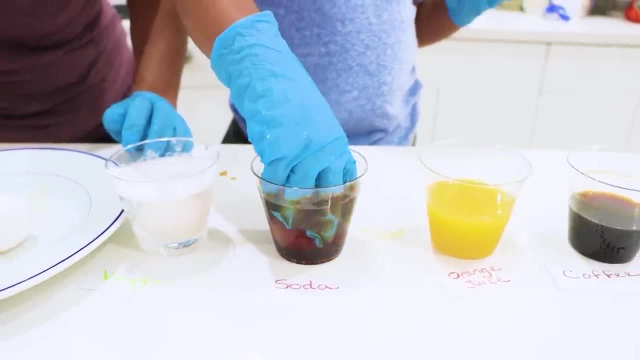 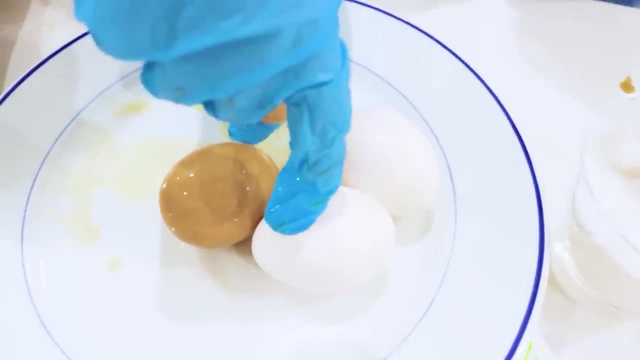 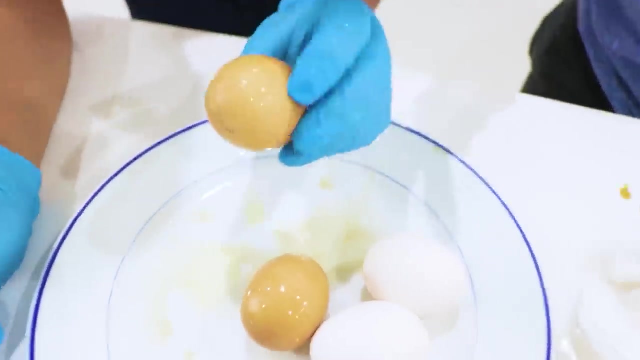 Let's see what happens. And soda also has lots and lots of sugar. Oh no, It also stains the egg, Wow. So this is like a super good version. This is a second best version. This is the worst version. No more white teeth, right? 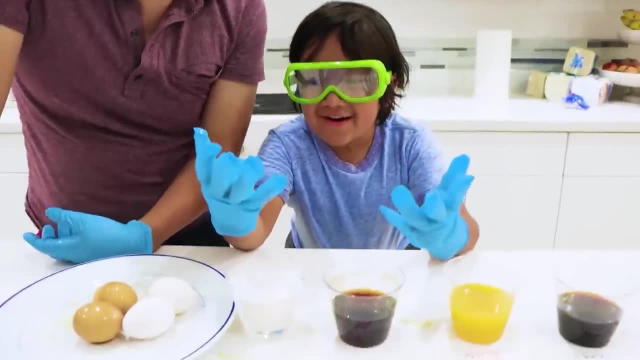 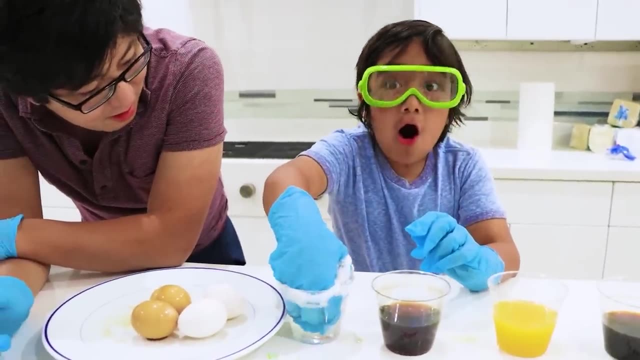 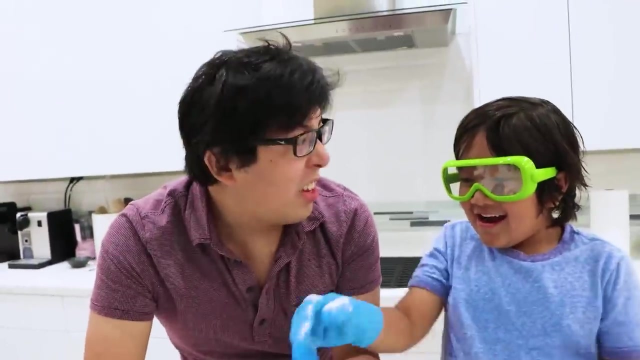 Yikes, This is the most exciting one, Vinegar. Alright, let's see, Take it out, Ryan, Take it away. What? What You got to be gentle? What happened? Feel it. Feel it, It's soft. What? What happened to the shell? 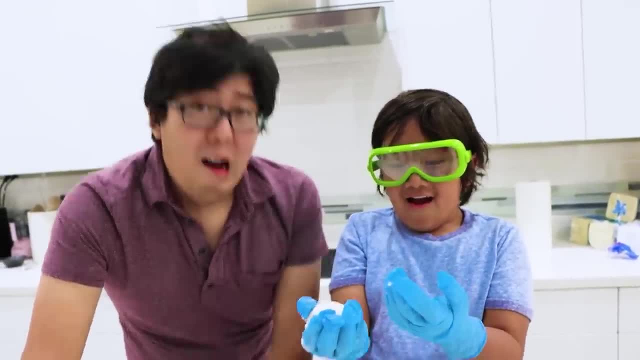 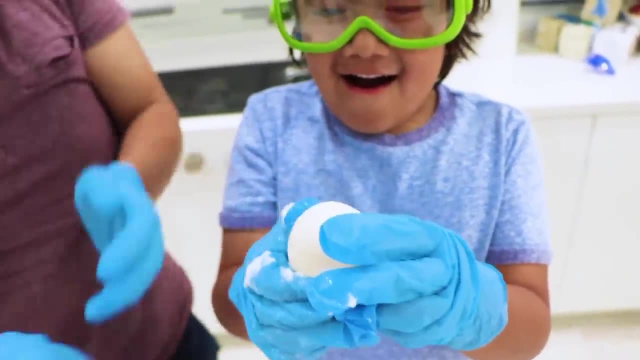 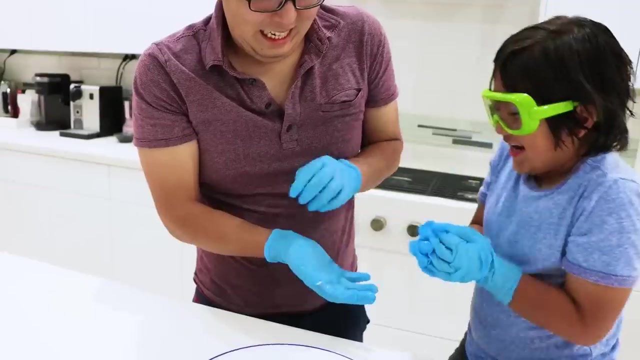 Vinegar is very acidic, so it actually dissolves the shell. The shell is gone, Ryan. I knew it. It's all you left. Don't squeeze it, It's going to explode. It's like a bouncy egg. Are you scared to bounce? 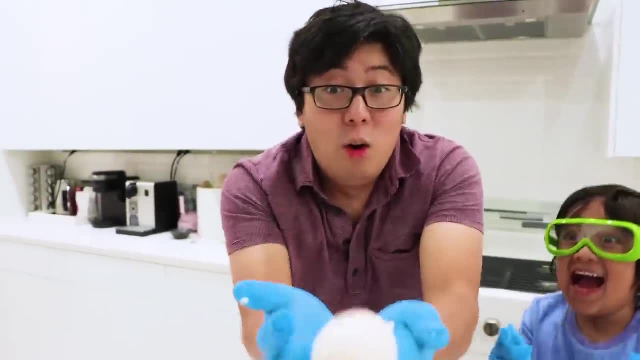 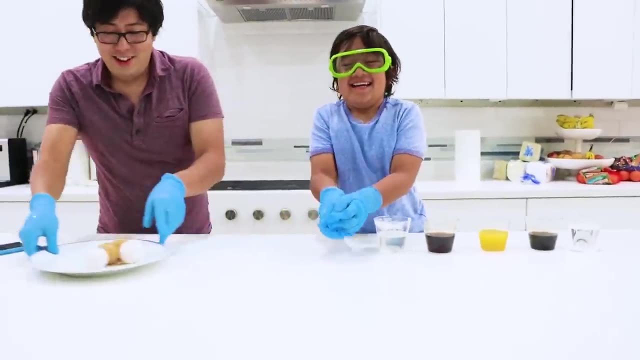 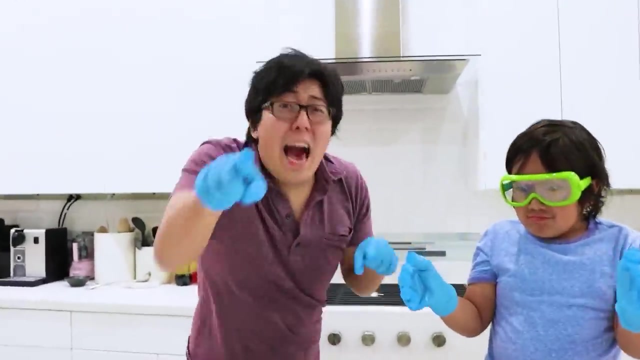 Yeah, It's actually pretty bouncy, you guys, You can bounce it. No, I'm scared It doesn't burst out. Burp, Mommy, you lied, So maybe we should have kept it in there a little bit longer. It would have been a day. 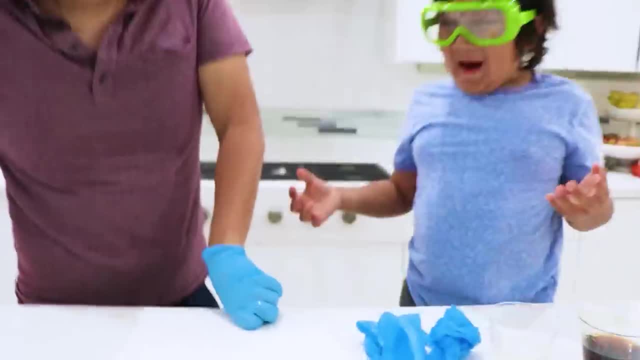 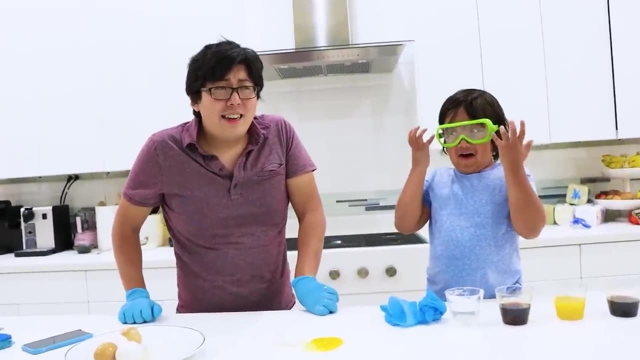 so maybe you need two days. So there it is, the shell there. Now it's a little bit too much, but if you leave it in for two days it's actually more bouncy. Wow. So now you know what happens to vinegar. 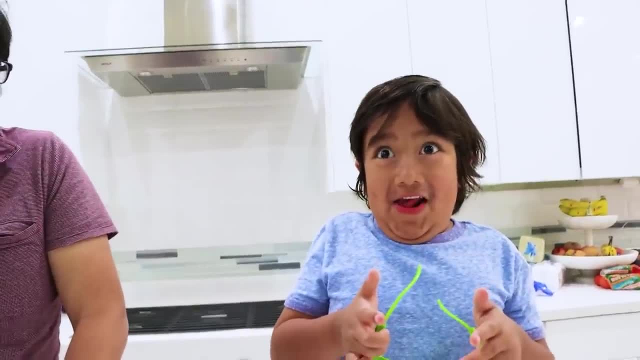 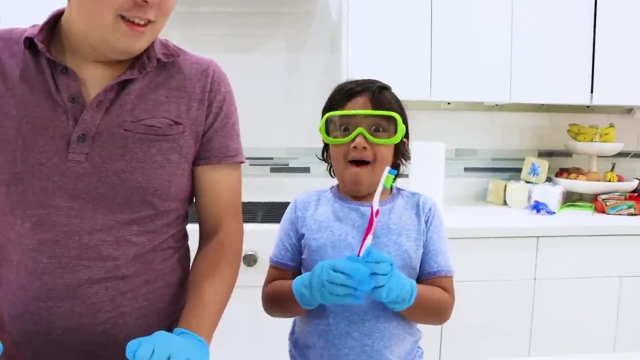 What does it do? It dissolves. It dissolves. All right, guys, Clean up time. We're back. We cleaned up, We got new gloves, right. And then Ryan learned not to touch raw eggs, right? Yeah, Ryan also go wash his hand already. 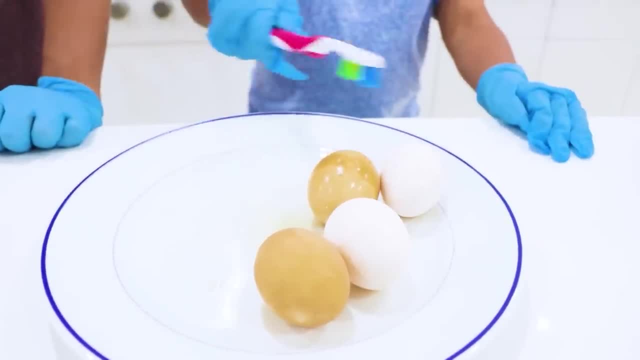 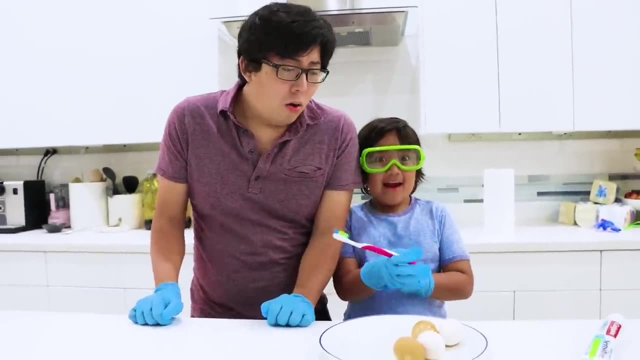 So now do you see how the eggs that was in coffee and soda was brown? Ugh, We're going to test it out, to brush it, yeah, to see if it has any effect. Okay, Yeah, Yeah, make sure you put. 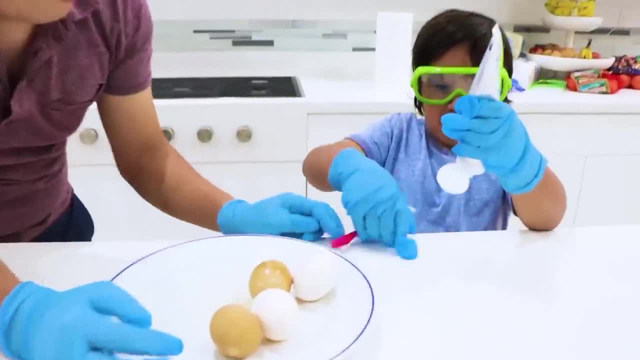 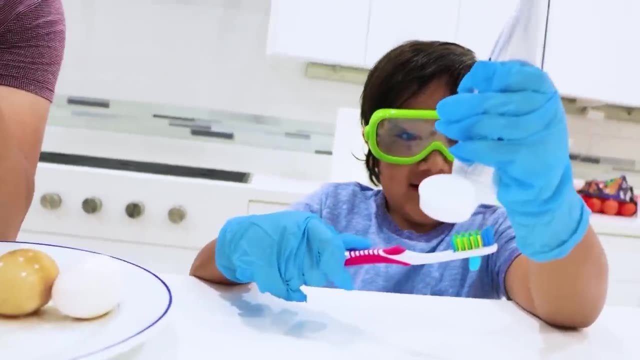 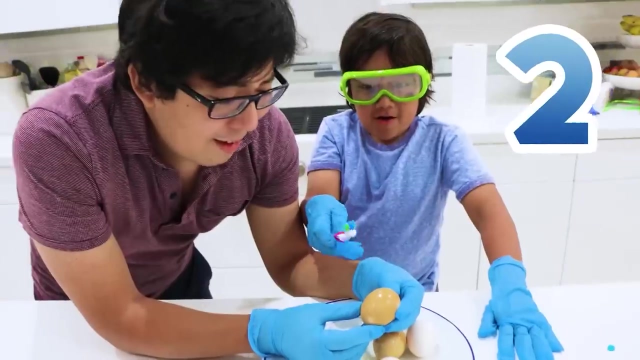 the toothpaste on. Oh, Teamwork. Ugh, Cannot be my toothbrush. Okay, Ryan's holding gloves, so maybe that's why it's a little bit hard. Yeah, that's good, Here we go. Three, two. 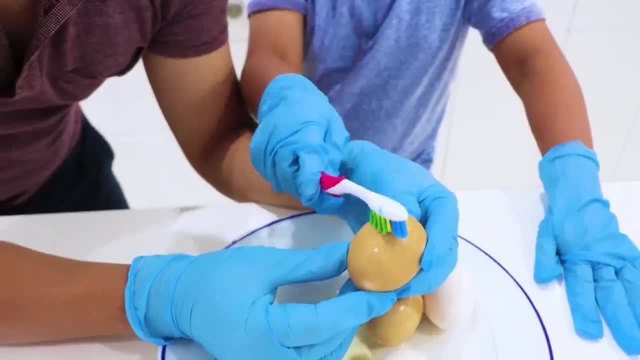 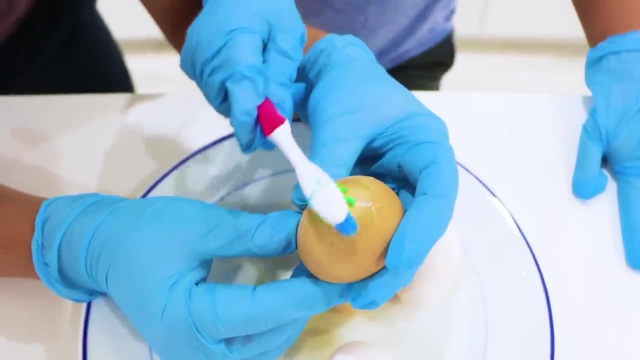 one Brushy, brushy, brushy, Brushy, brushy, brushy. Ten hours later, No, We're seeing if it works. Whoa, whoa, I can tell already: Does brushing help make your teeth whiter? 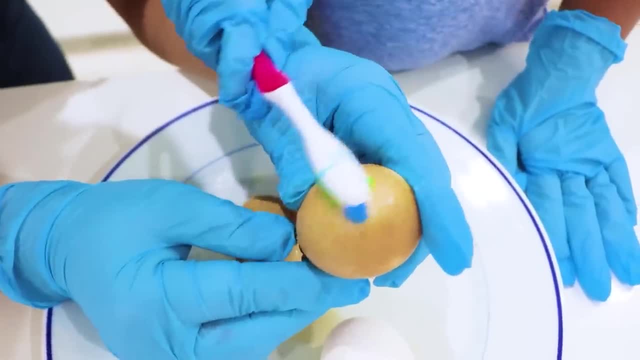 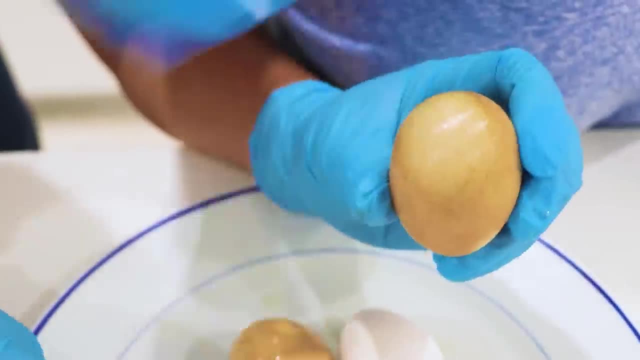 So, Oh, yeah, I see it, Look, Yeah, Yeah, Ryan, look, It's already getting less brown on the spot that you're brushing. You guys see, Oh, look at it, Oh, it's already the difference This is. 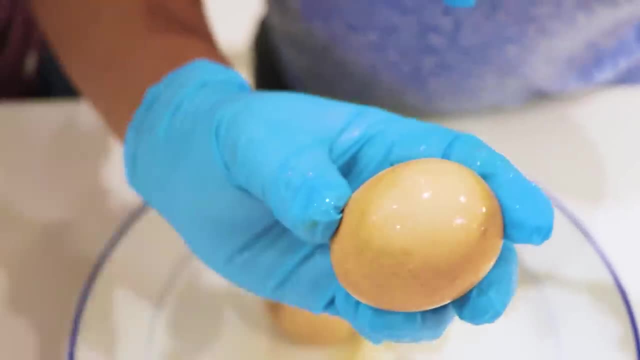 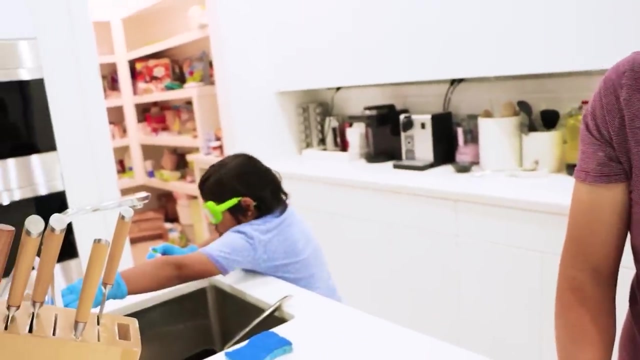 the regular spot and this is where we brushed it. Oh yeah, Look at how, yeah, Wow, the importance of brushing your teeth. right, Ryan's brushing the toothbrush. Oh, Oh, Okay, Ryan's brushing more to see. 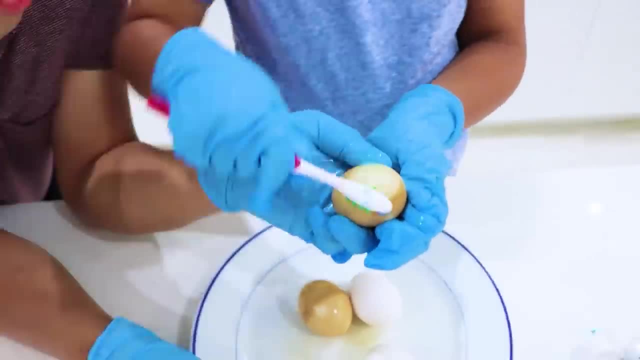 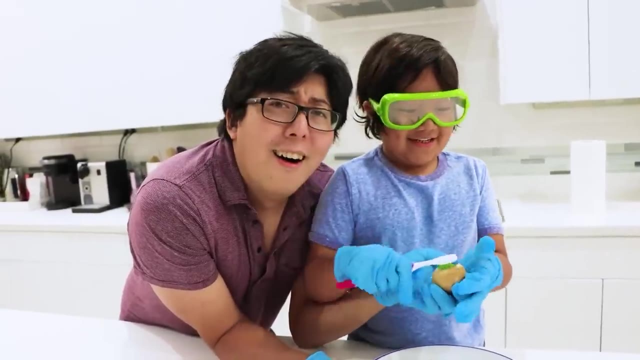 Whoa, Oh, yeah, I can tell the difference. Good job, Ryan. Whoa, You see the difference. Yeah, I can tell Nice Big difference. So what did you learn, Ryan? That brushing your teeth helps a lot. 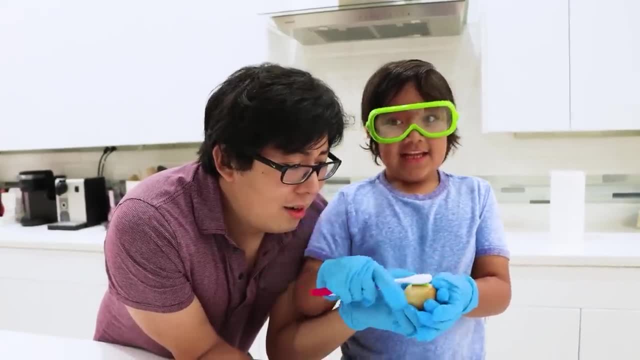 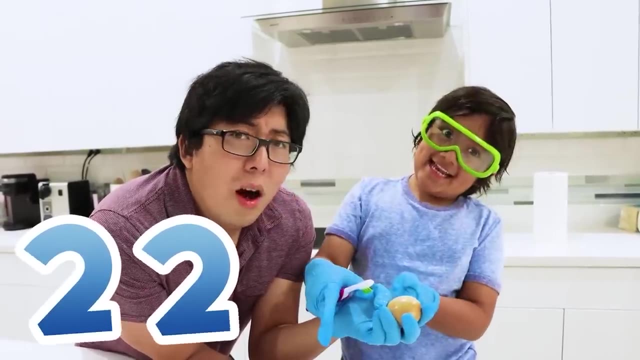 Yeah, it does. And how many times a day you're supposed to brush your teeth? at least Two, Two times a day. Good, For how long Do you know? Two minutes, Two minutes- Yeah, Easy to remember. Okay, guys. so today we're going to be using 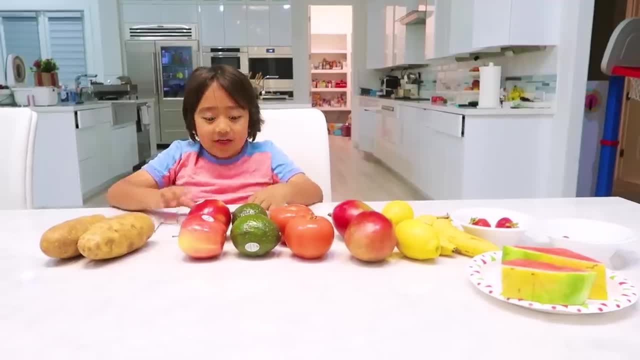 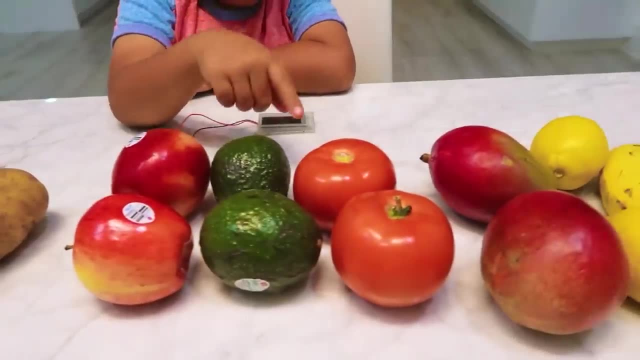 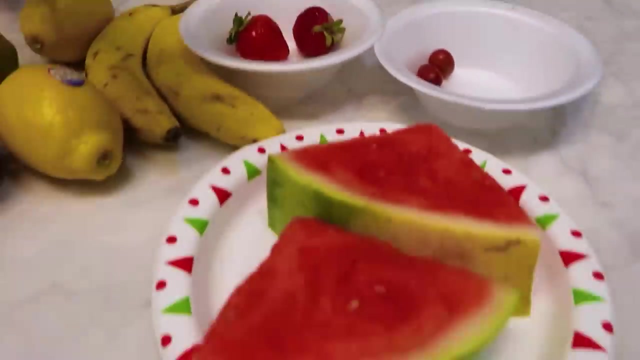 ten different vegetables or fruits and we're going to see if they can power this alarm clock. So we have potatoes, apples, avocados, tomatoes, mangoes, lemons, bananas, strawberries, grapes and watermelons. First we're going to. 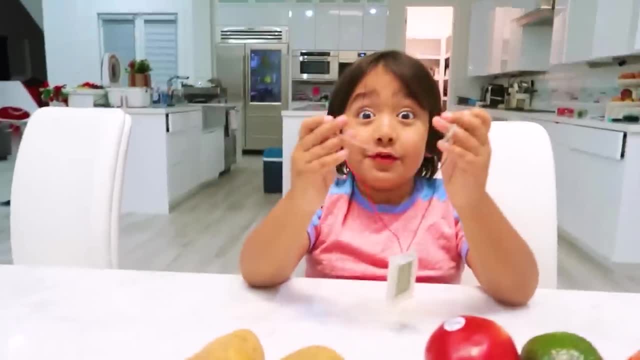 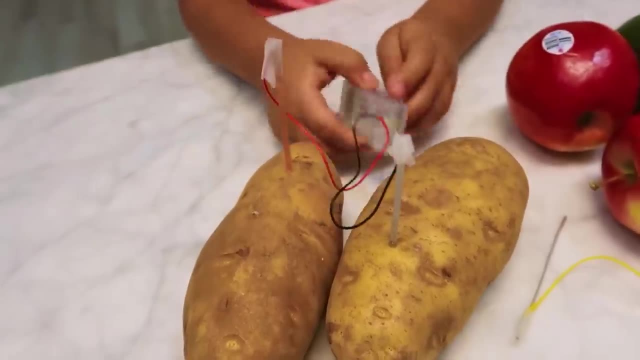 try the classic potato. It was made for potatoes, so I think it's going to work. Three, two, one, Oh. So if you notice here, look at the alarm clock. Is it working yet? Not yet. We got this kit online, So it. 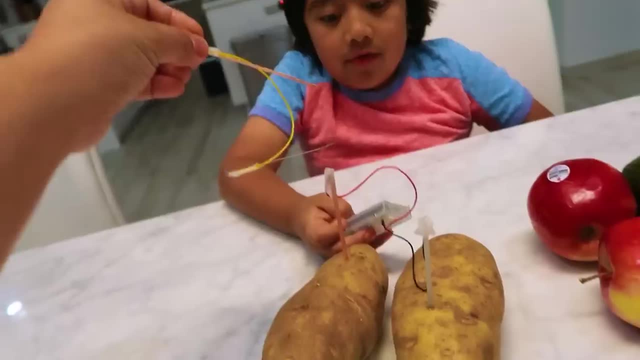 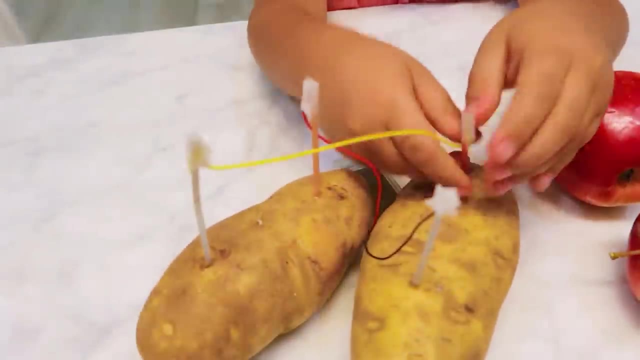 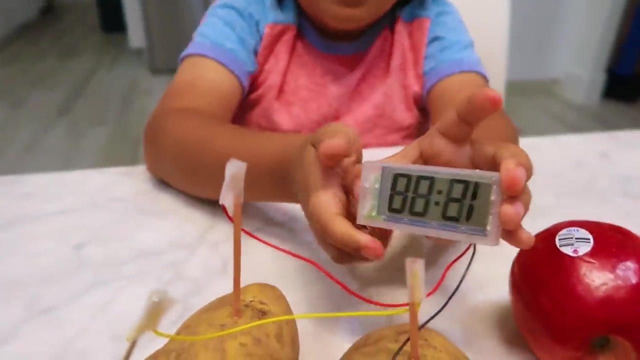 comes with a magnesium wire and a copper wire. You have to connect this two. This Uh-huh High, Yeah, And here. Alright, You tell me, is the alarm clock working? Look it's working. Yeah, it turns on. It's got enough energy. 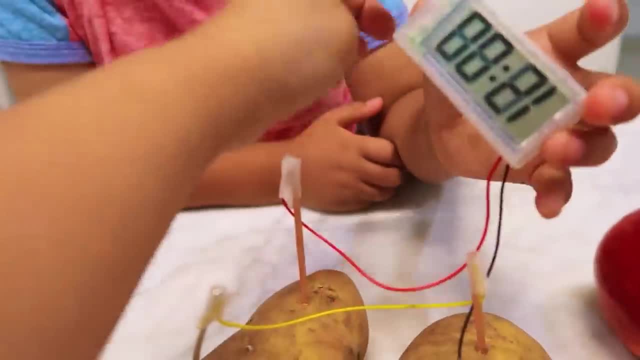 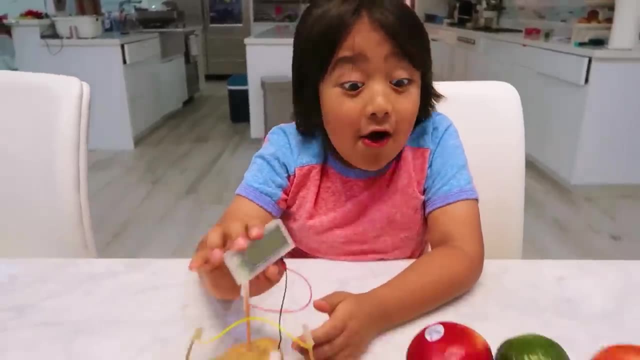 Yeah, so we have to manually set it. but you know, there it is, A potato works. I'm going to use a potato for my alarm clock tonight. Okay, now let's try the next one. Next, I'm going to test. 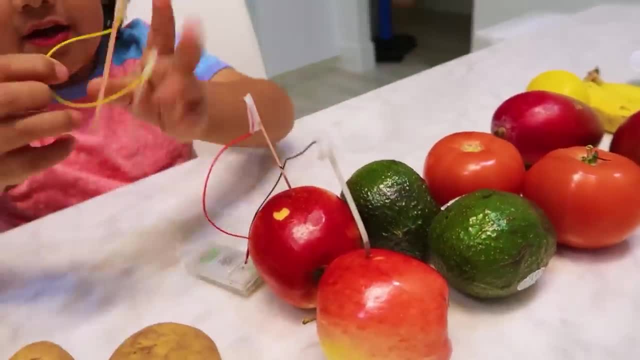 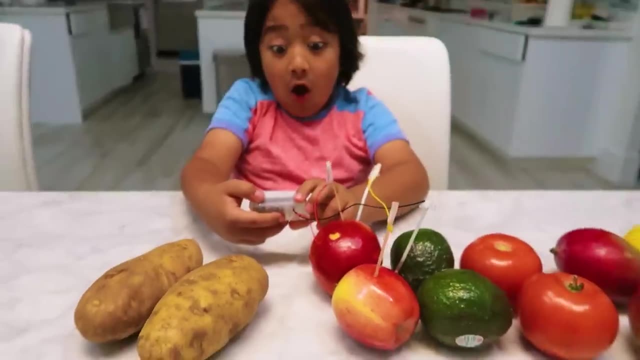 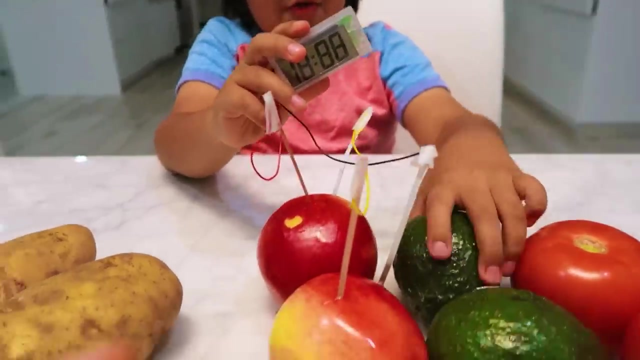 out the apple And do the opposite on the other one. Yes, like over here. There you go, Moment of truth. Does it work? It works, Yay, So an apple can also power it on. You know it's true because 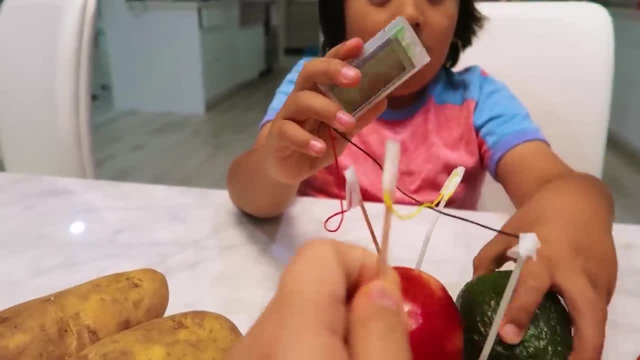 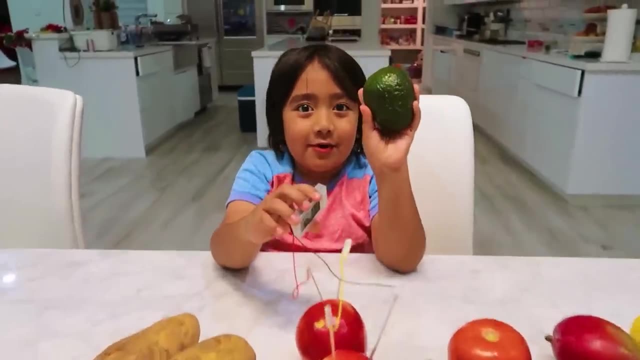 look what happened when I take out one. Okay, if I take out one, it stopped working, But if I plug it back in, it works. I'm really interested for this one, The avocado. Yeah, Guys, let us know if you think avocado. 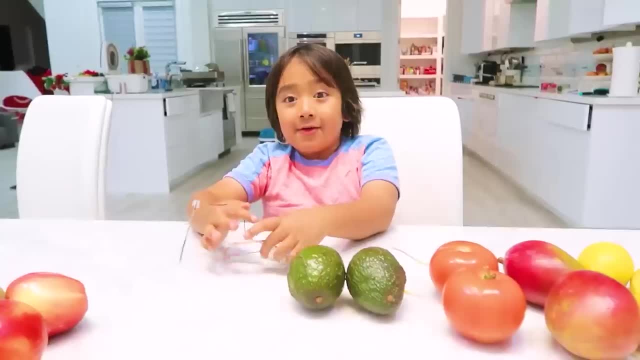 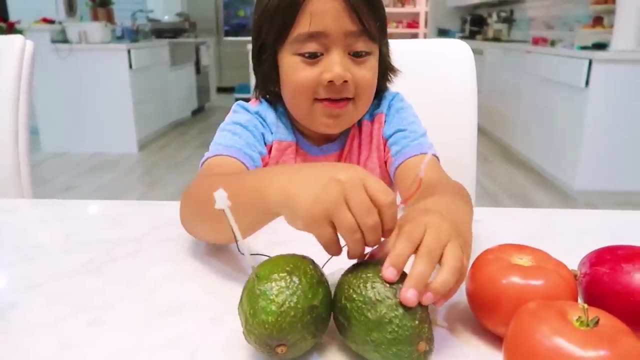 can power on the alarm clock. Now we're going to try the avocado. Oh, I think it's going to work. You think so? Yeah, You guys notice right now nothing's on right, So it doesn't work right now. So Ryan's going to put it in. 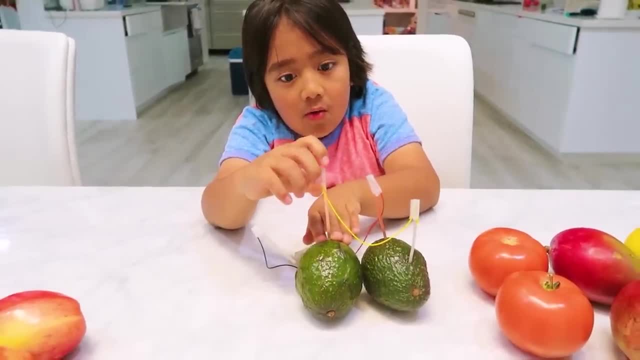 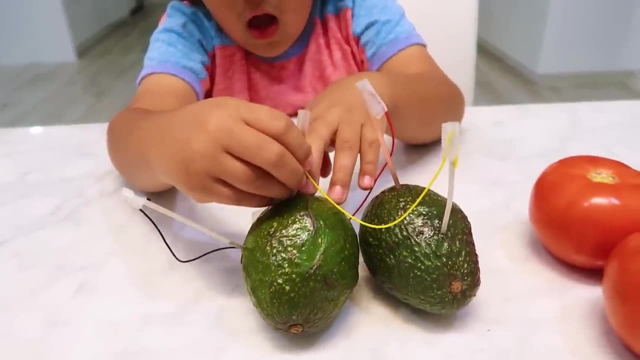 Can you use an avocado alarm clock tonight? Wait, did it mess up? I don't know. No, that's right. Yeah, it's supposed to be opposite. You need that to complete a circuit. Does it work? Avocado work. 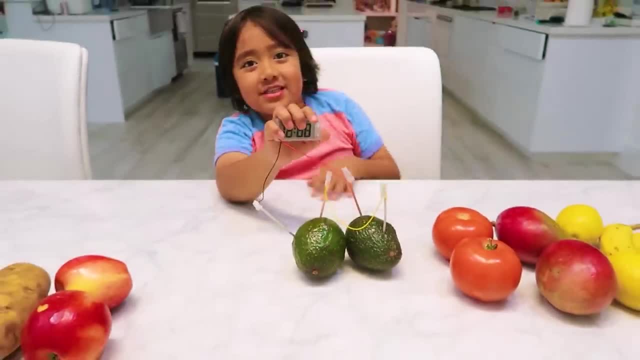 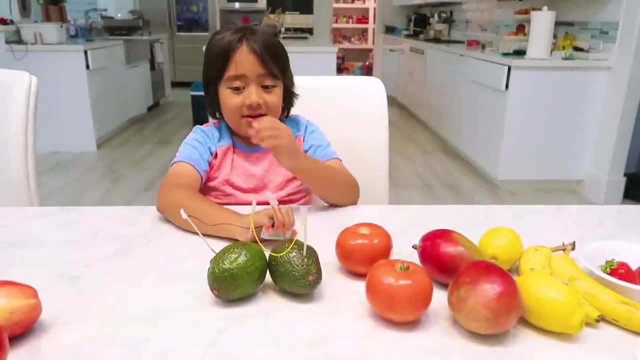 Whoa. Now the most interesting one is one, That's true, That one we're not sure. I think tomato, Wait. no, I think tomato will work, Tomato will work. Okay, let's see. Now we're going to try tomatoes. They're really messy. 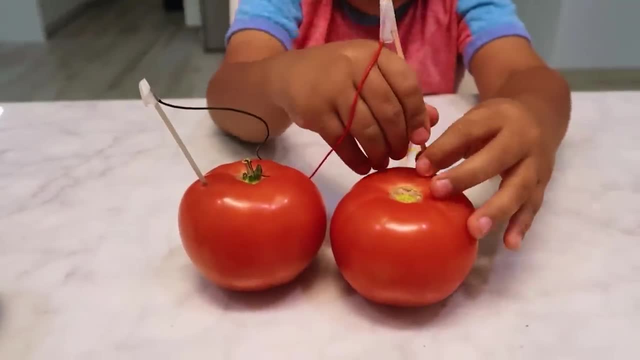 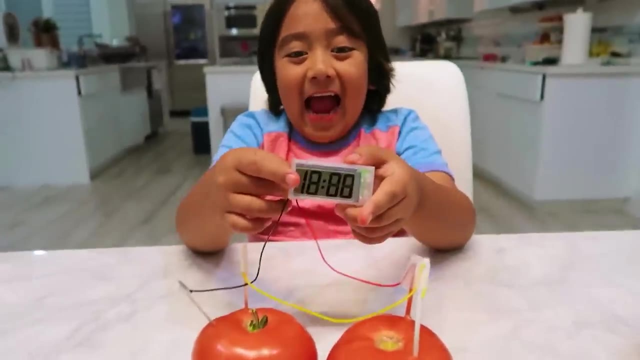 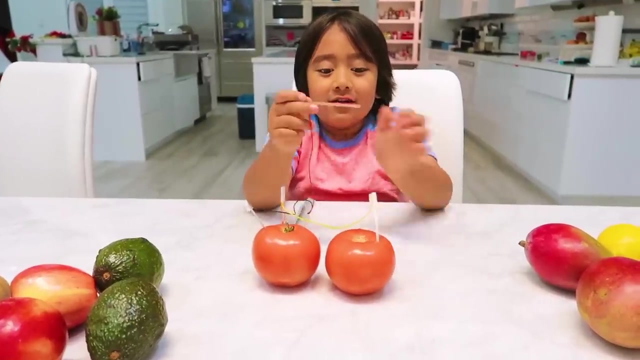 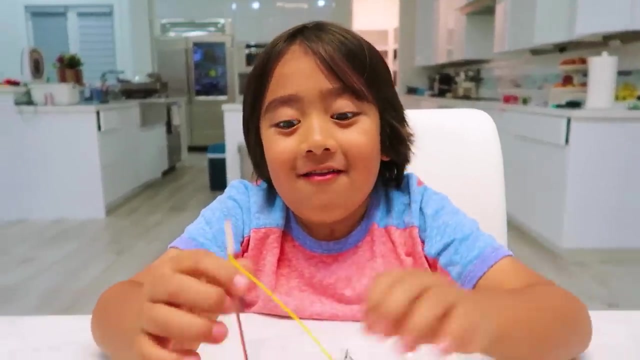 Don't poke it too hard. Pop Like this: Does it work? It works, It does work. Wow, Maybe we do need just fruits and vegetables In our alarm clocks. You think fruits and vegetables can power on your iPad? That's a fun experiment to do later. 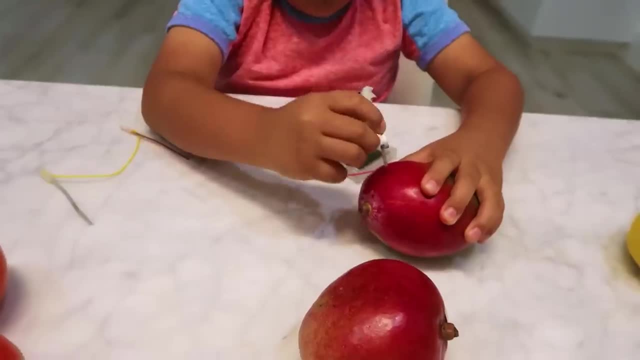 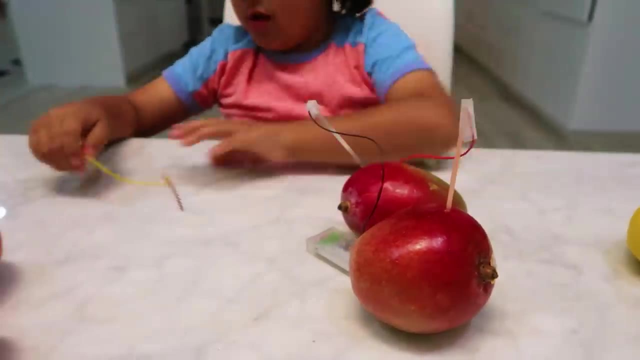 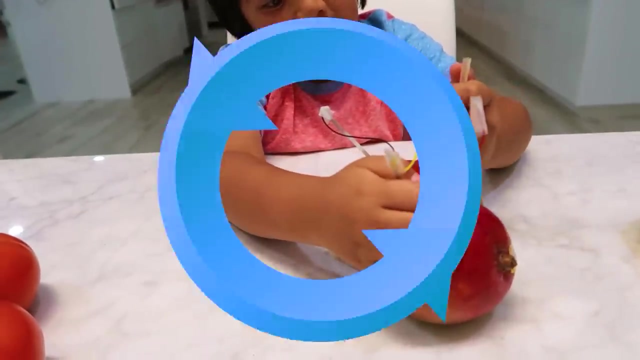 Okay, now let's try mango. Oops, It's bending the wire Here And then one. So you need the other part to make like a circle, You know, to complete the circuit. That's why you need it. Actually, the potato clock works. 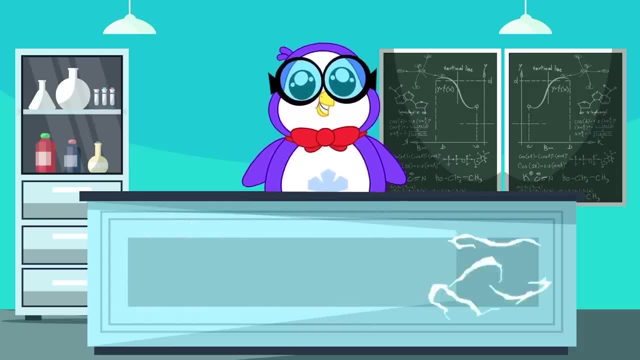 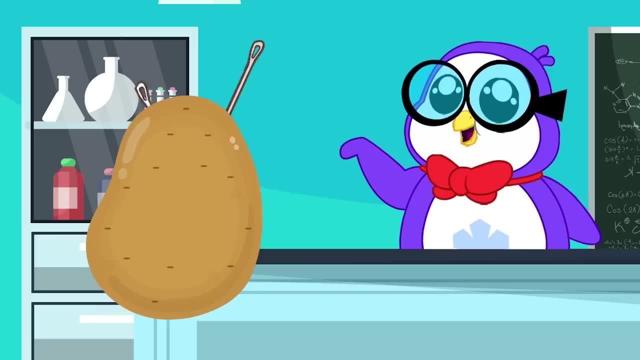 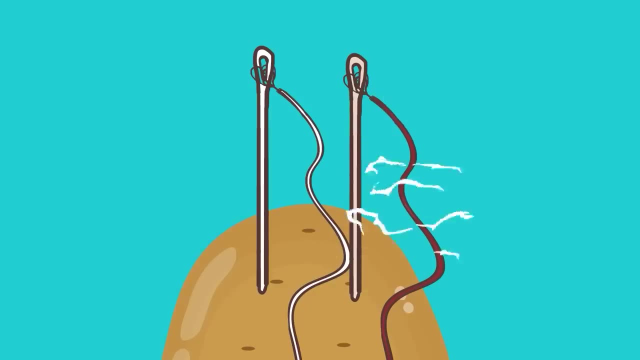 by converting chemical energy into electrical energy. Did you know that the energy doesn't actually come from the potato, But rather the energy comes from the metal dissolving inside the potato. The energy may come from the reaction moves to the copper. strip down the wire. 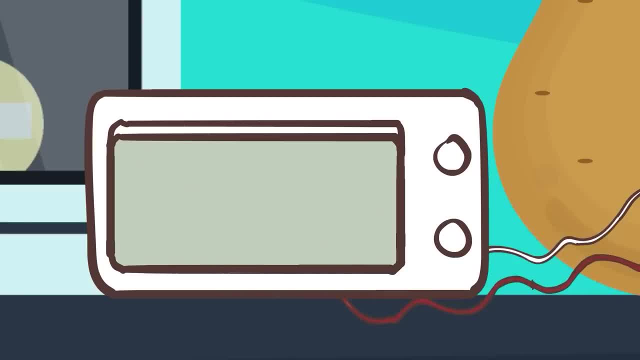 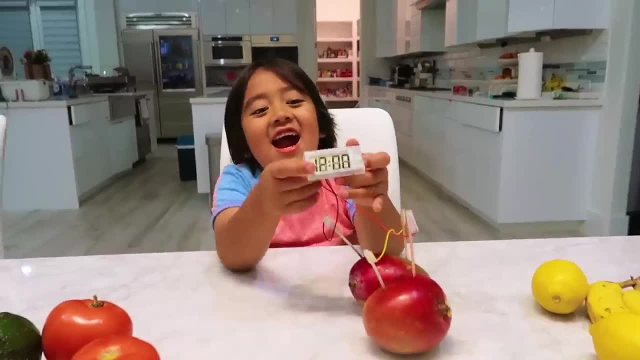 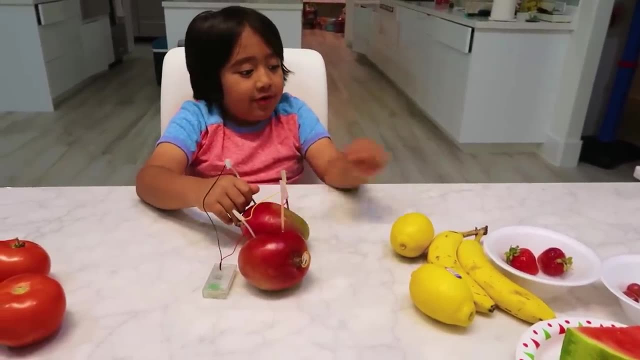 and into the clock, making the clock turn on. That's spectacular. Here we go, Yeah, Wow, everything works so far. Look Which one do you want to try next? I want to try the banana. The banana, Wow, that's interesting. 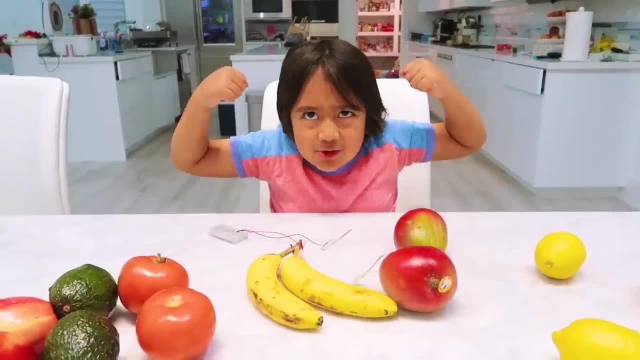 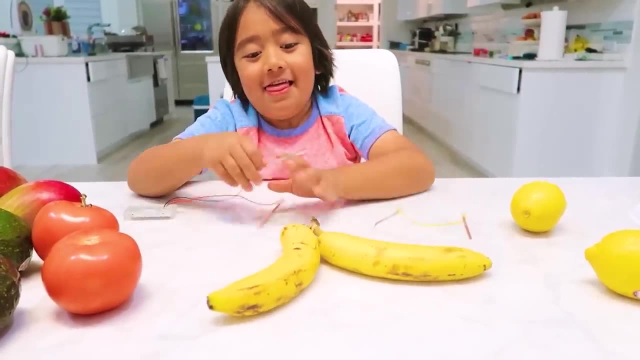 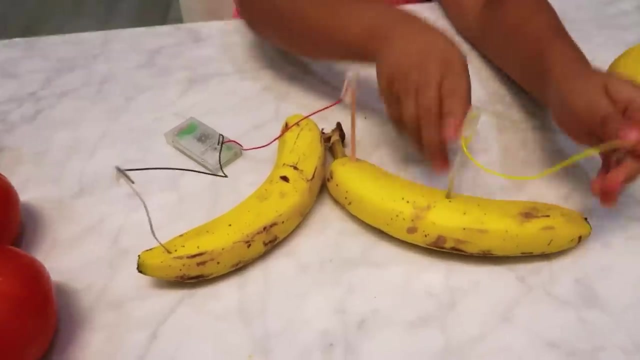 I think it'll work. You think so. I think it has energy. Yeah, Now let's try banana. I'll try it like this. Okay, So it's easier to do positives and negatives. I'll put it here, Put it anywhere you like. 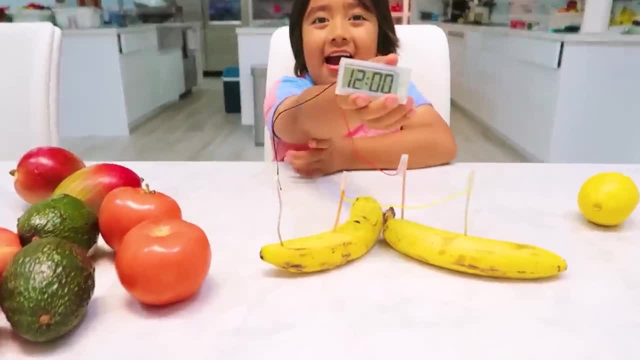 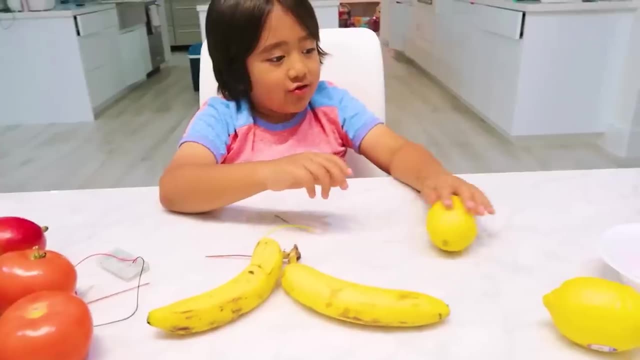 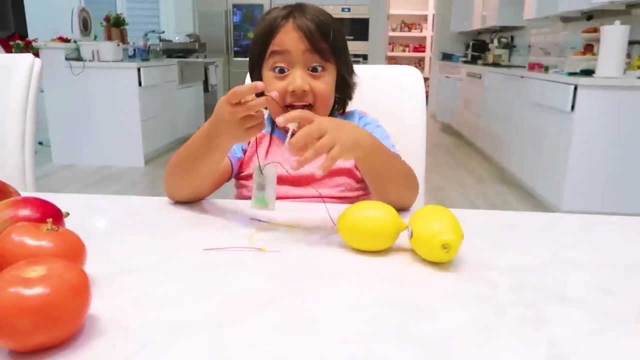 Well, Enjoying a different time. but yeah, Oh, it does work. Yay, You have a banana clock, Woohoo, Now let's try the banana. Whoa. You think trying the lemon's gonna work? Yeah, I think so. Oh, yeah, it's gonna work. 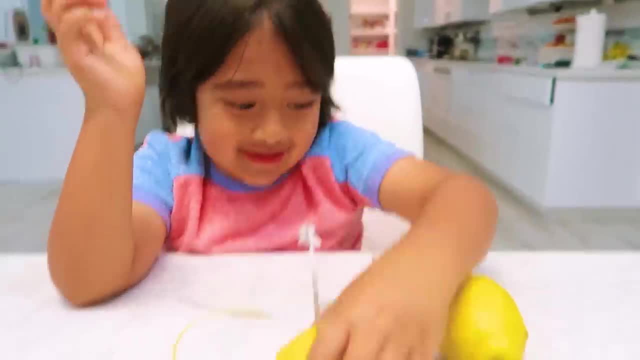 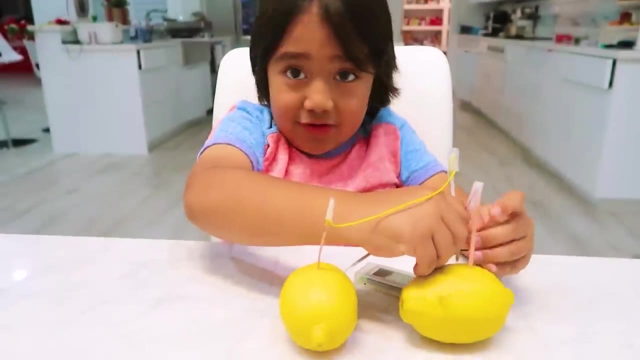 It's hard to poke in. It even has a smell. See, right now it is not on you guys. Three, two, one. What do you think it's gonna do? Work or not? Definitely work. I don't even have to poke it in. 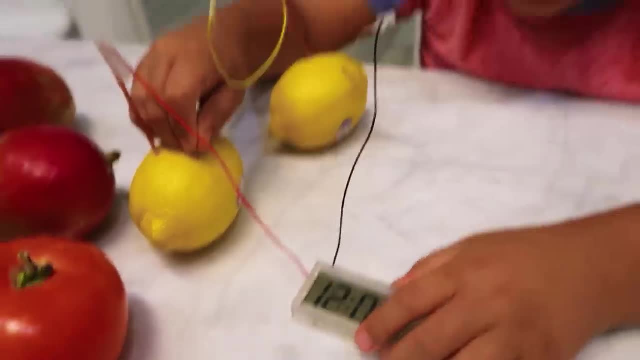 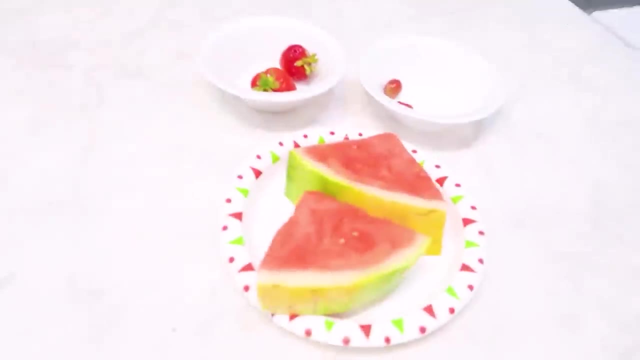 What. That's crazy. So I guess you don't really need a lot of power. So so far everything works, so far. Wow, Which one do you want to try next? These three I'm very interested in? Yeah, I'm gonna try this one. 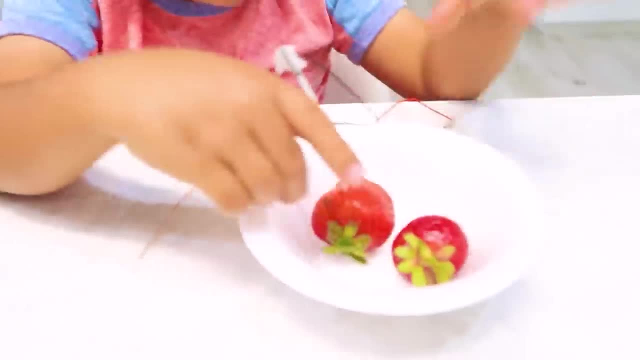 The strawberry. You barely have to poke this in. to poke it in, I wanna see if we can do the same thing we did with the lemon. I wanna see if we can do the same thing we did with the lemon. Oh, good idea. 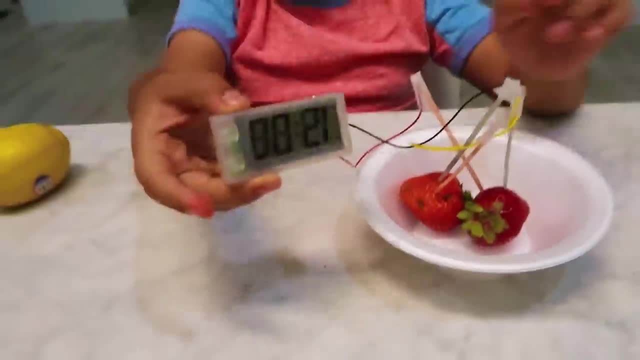 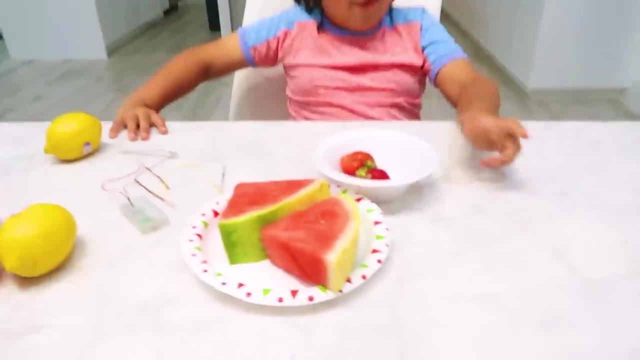 Look, Look at it. Wow, very cool. Which one do you want to do on here, grapes or watermelon? Watermelon, Okay, cause grapes it's so small, I know, Is it gonna work Because it's so tiny. 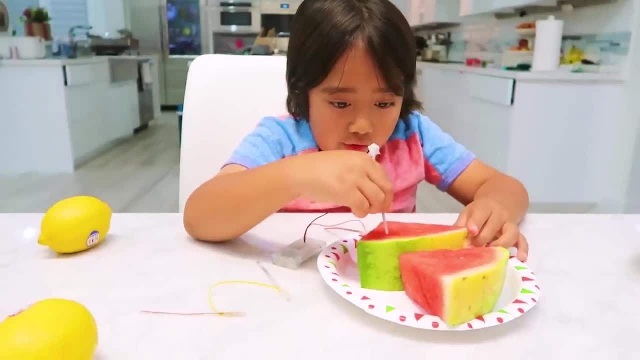 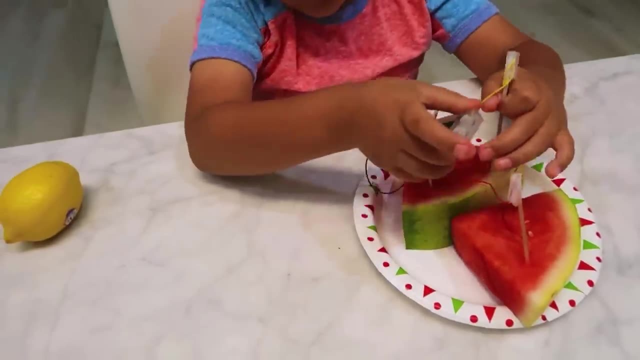 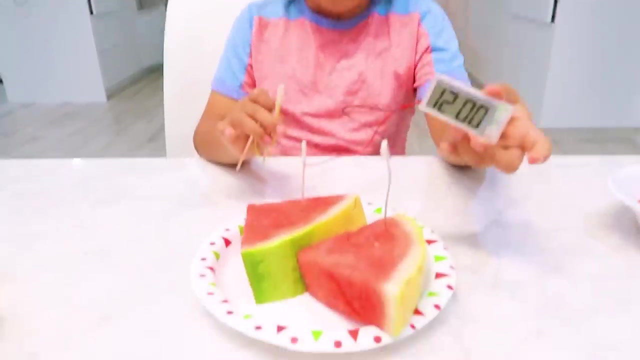 Oh, watermelon's gonna work, Let's see. Okay, Oh, it's so easy to poke in, Is it working? What Guys? I didn't even need to complete the circuit, It just powers off with two. Wow, I didn't know watermelon's so powerful. 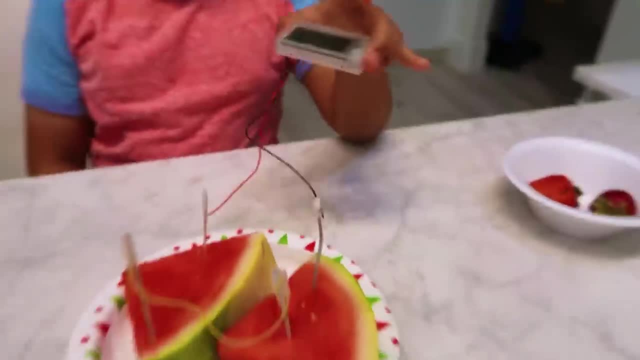 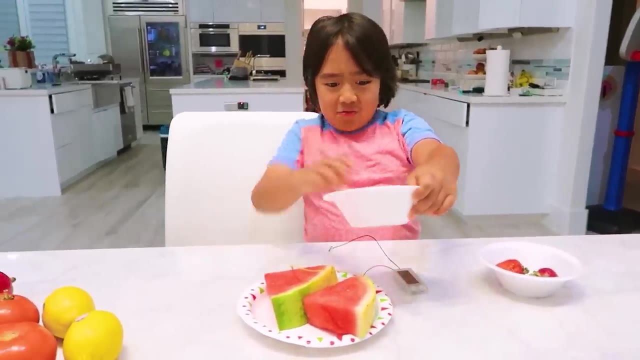 But this makes it a lot more powerful, So it does work. Yay, Yeah, Let's try the last one In the most. Wait, how is this gonna work? I don't know. it's so small. How are we gonna make it opposite and positive? 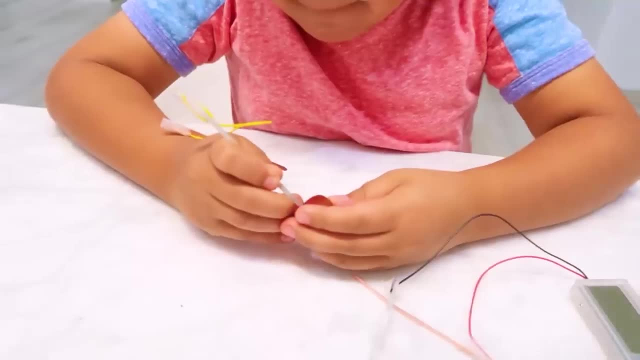 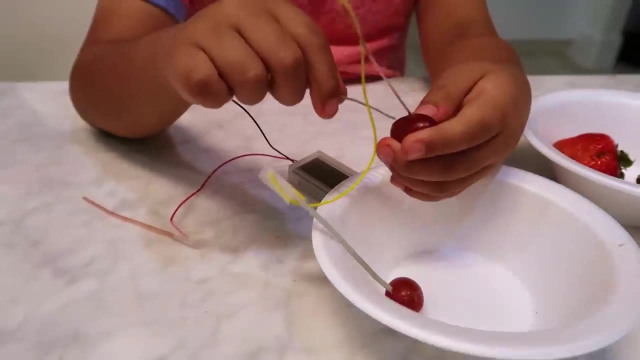 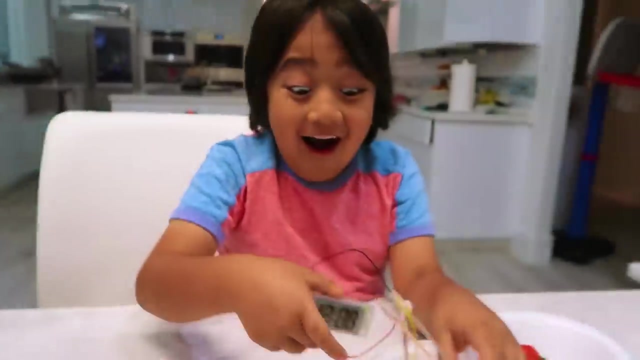 You have to stick them very gently, Can you do it? Yeah, I did one. Now I do the other one And one here. So far it's not working. Let's see What Grapes can power on a clock. 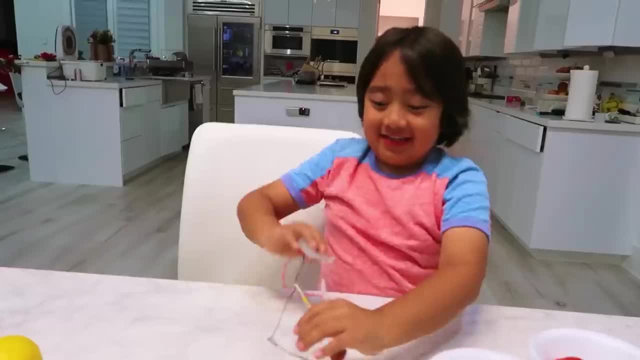 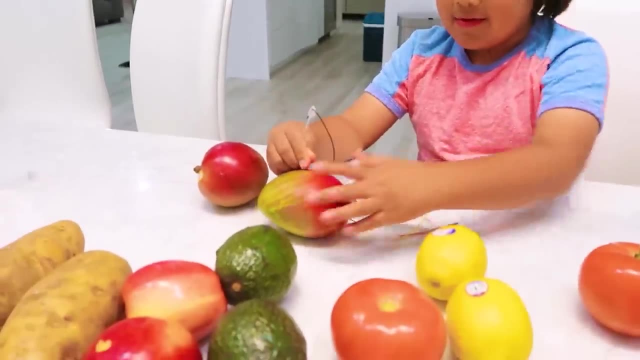 Look at that, you guys. Just two grapes, That's it. That's all we need. Don't need a whole potato, You just need two grapes. What if you just try one of them? With all of them, It's working. 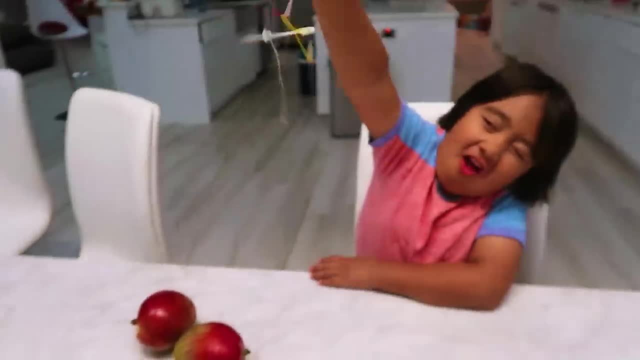 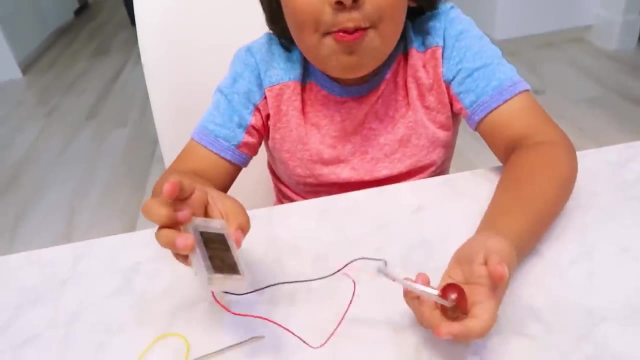 Yeah, all you need is one fruit, One grape. it is. It does work. Look, We don't even need to complete the circuit, It's so powerful. This is the most powerful. Yeah, I think all you need is one, Ryan. 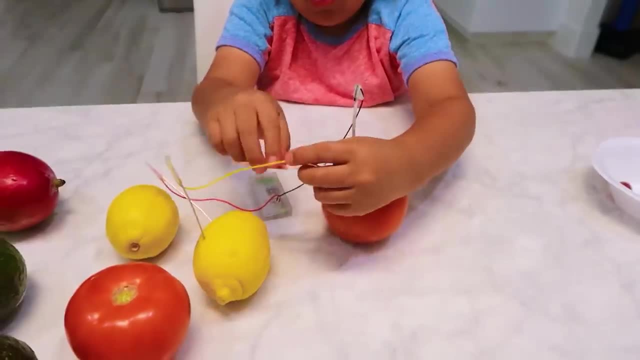 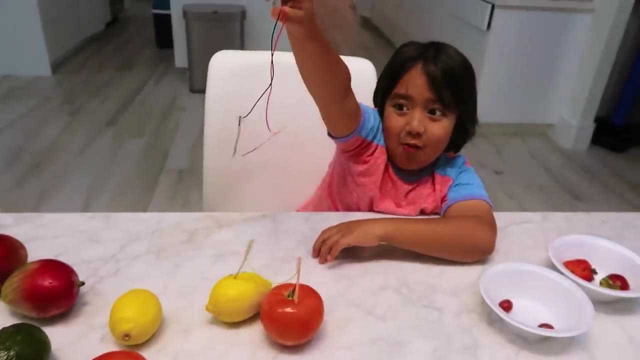 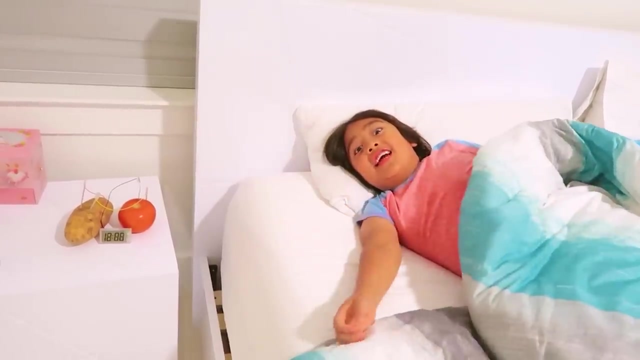 Like this. So Ryan's trying out different ones. One tomato and one lemon. It works, Woohoo, Yay. Okay, guys, I'm gonna take my alarm clock to bed. Let's go. I'm gonna go to bed now. 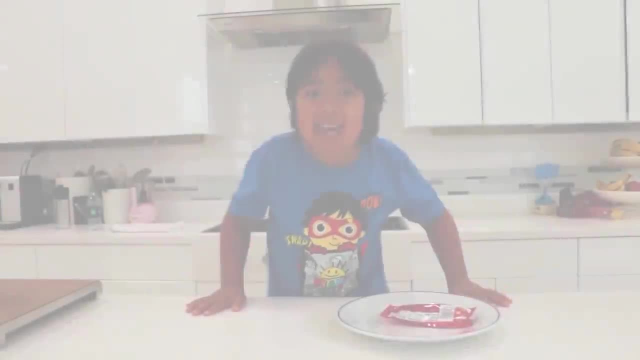 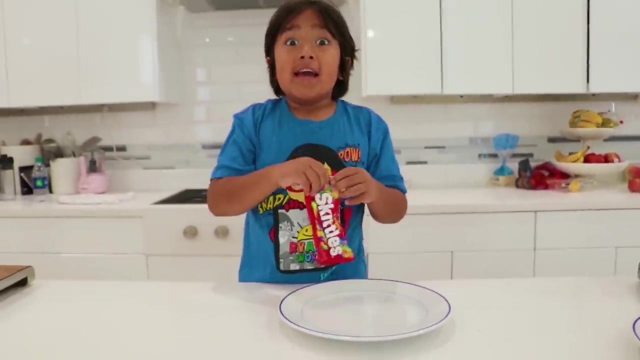 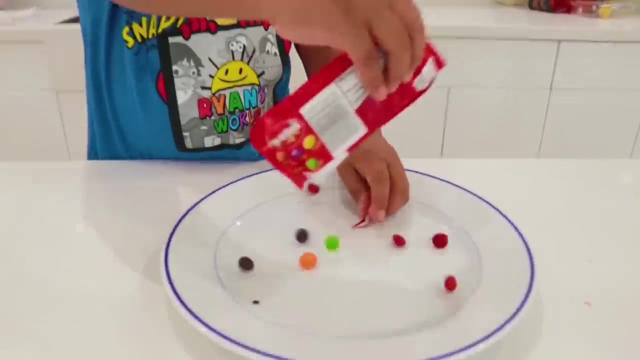 And that's how you make a fruit and vegetable alarm clock. Hi guys, Today we're doing a science experiment with Skittles. We're gonna see if Skittles' color dissolves in water, And I think it does. Now we're gonna spread the Skittles. 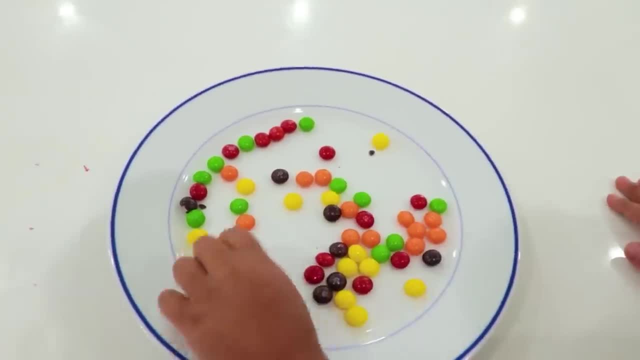 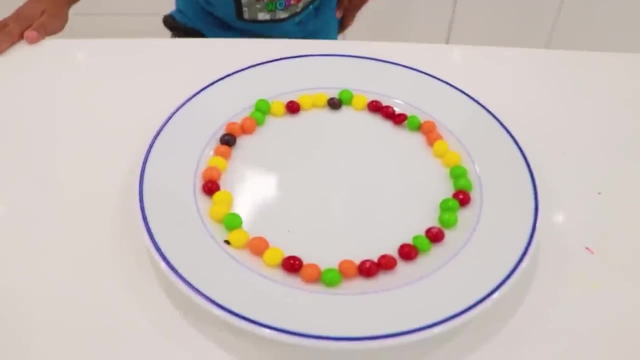 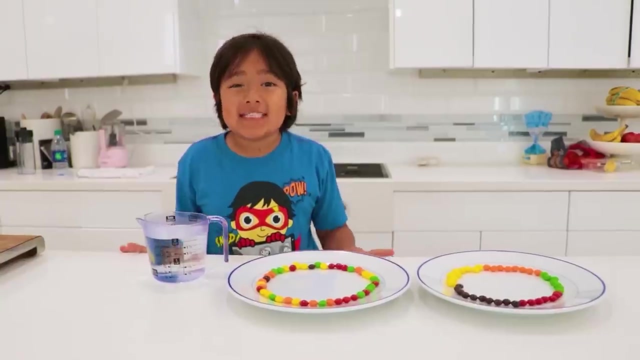 around like a circle on the plate. I'm spreading all the different colors around Like this, All done. Look, You can do it however you like, Cause I made it like this and like this. These are all the colors together. Next, let's pour water onto the plate. 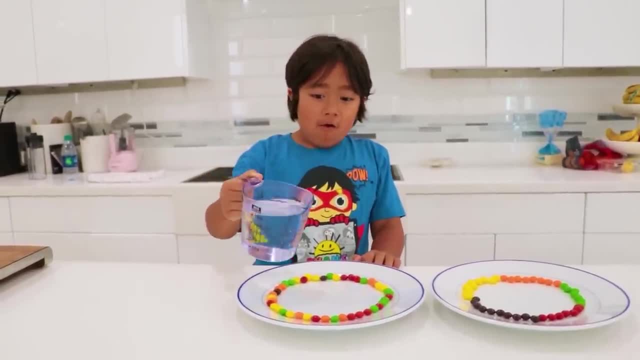 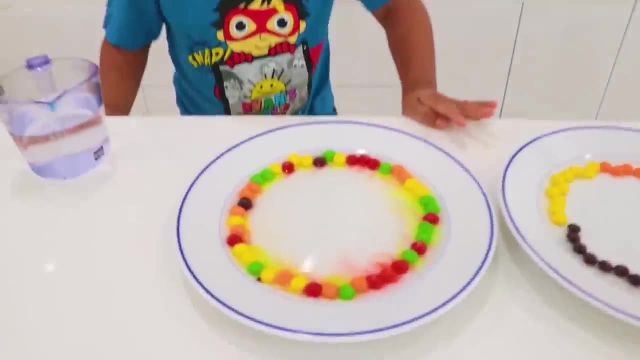 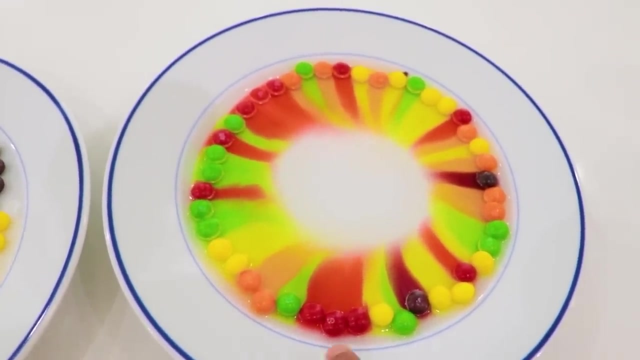 So Ryan's using warm water, So don't forget to ask a parent for help. Now we're gonna see what happens. It's already happening. Whoa, Look what's happening. So cool. The more they mix together, the more bigger they are. 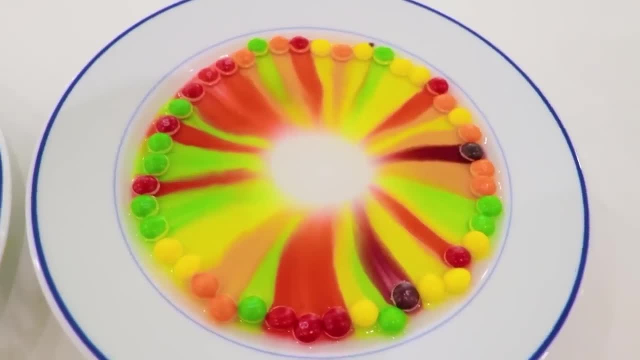 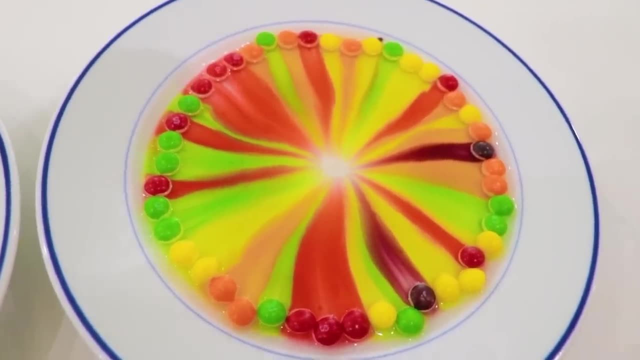 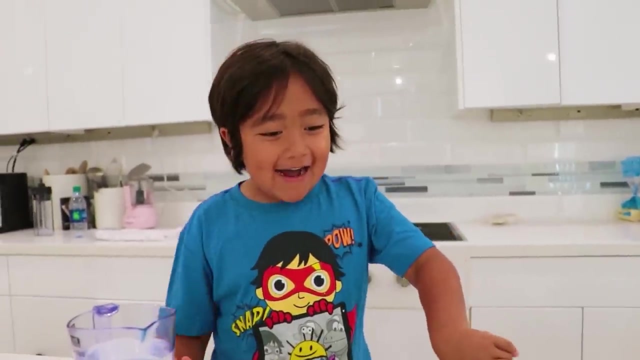 So what you notice is that the color is beating in the middle, right, They are dissolving. That looks cool, Whoa, Whoa. That is so cool, Whoa. And what did you notice? Did the color mix together? 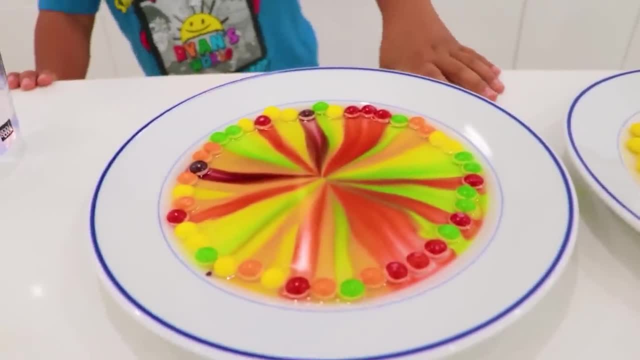 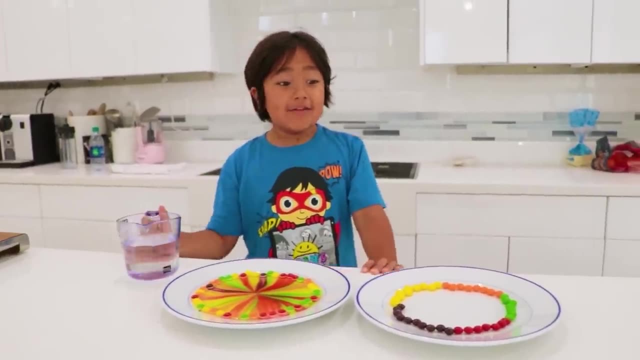 No, Look it separated right. The colors did not mix, only meet in the middle. Now let's try the other one and see what it looks like. I think it's gonna. those colors are gonna be really, really big. 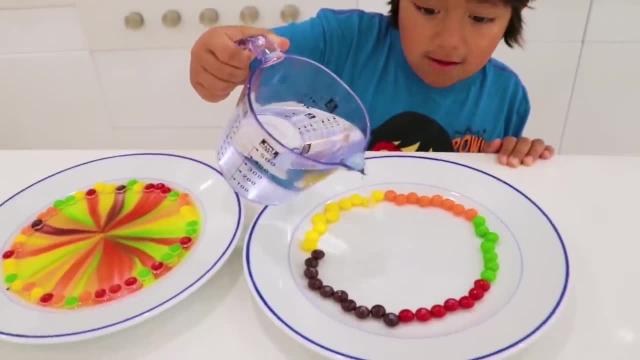 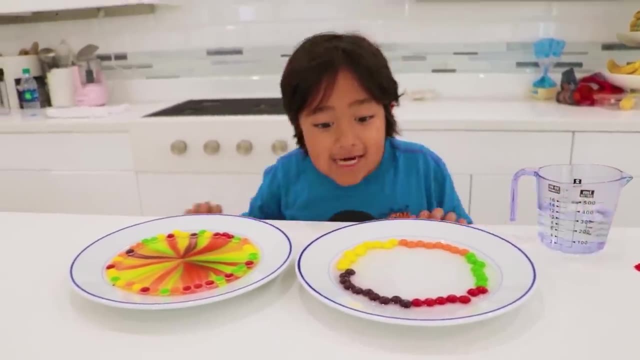 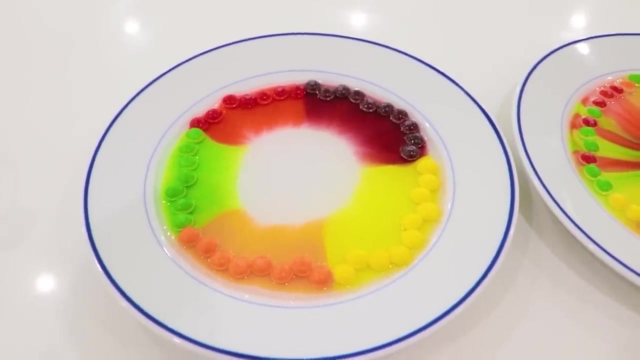 Three, two, one, That's enough. Whoa, what's happening? Whoa, Um, you know, there's like a little toy thingy where it says: press this color, then you have to follow it. It kind of looks like that. 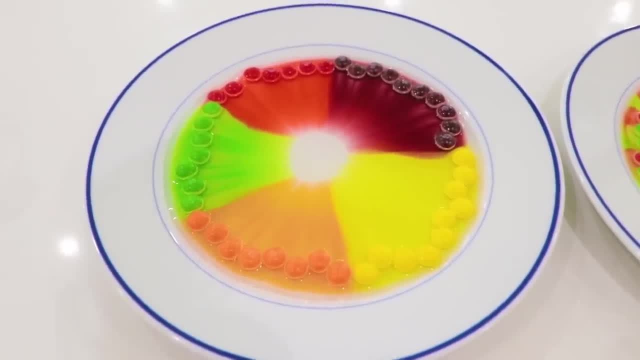 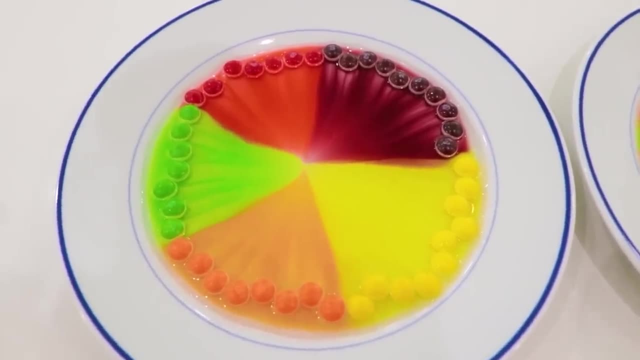 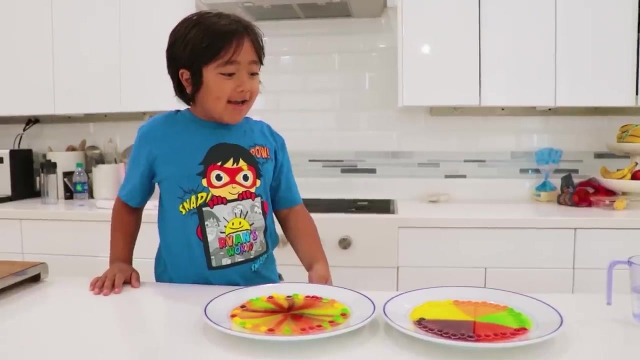 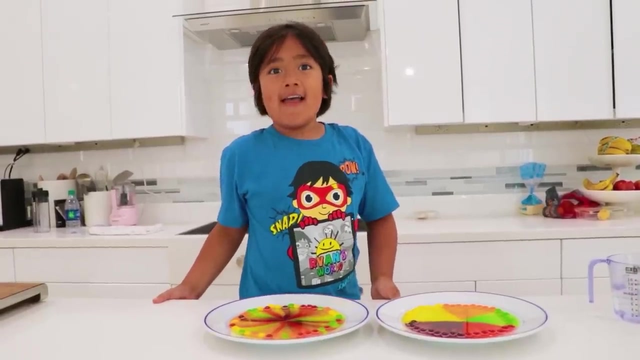 Oh yeah, it does. Whoa, Three, Two, One, Bye-bye, Whoa, That looks like a pizza, It does. It looks so cool, guys, It does. and look, Since we did different patterns, they look differently. 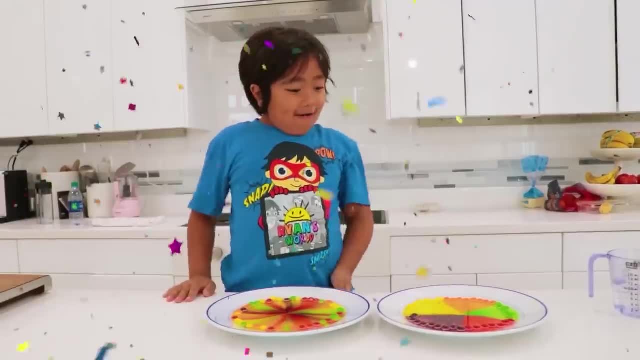 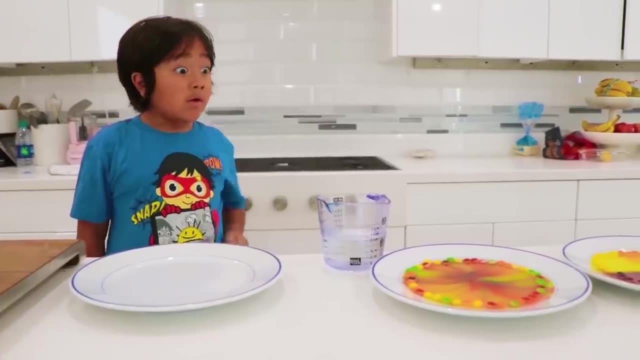 It's like dissolving water. Yes, It did. yeah, The food coloring on the Skittles and the sugar both dissolve in water. That's why we get really cool colors like those. Hmm, If Skittles dissolve in water. 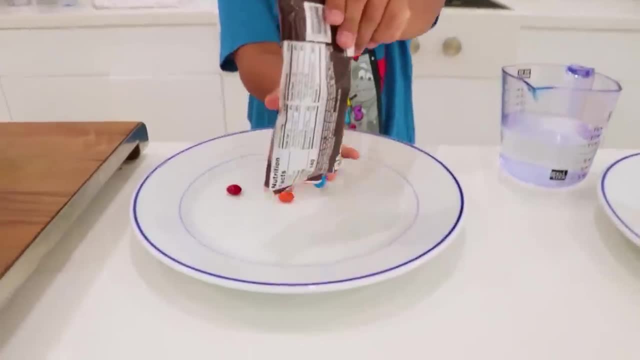 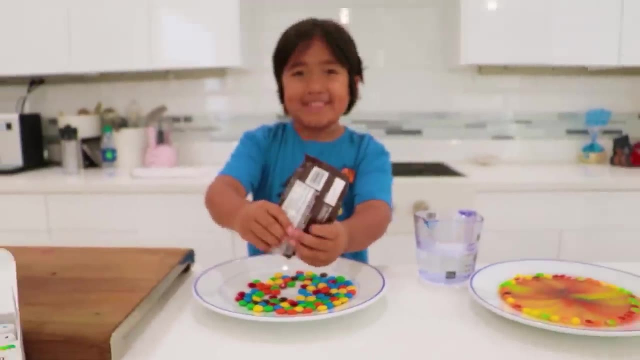 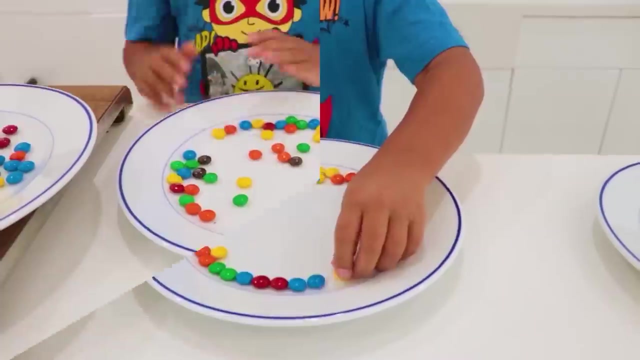 do M&M's dissolve in water? Let's find out. Whoa, That's so much M&M's Now. let's spread them out on the plate Like this. Let me make some of them big Now. I have two of them again. 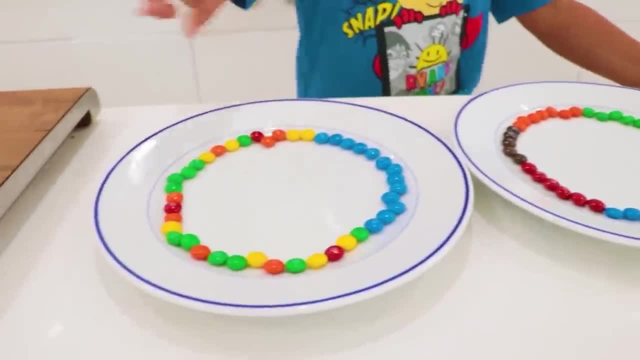 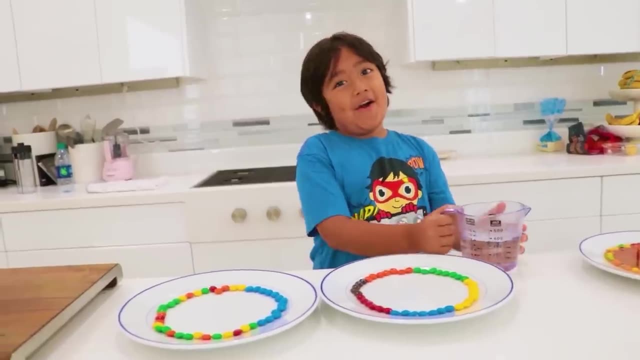 I have one with a lot of colors and I have one that's random. Let's try. We're also using warm water, so we're going to try one with warm water and one with cold water. Let's see if it makes a difference. 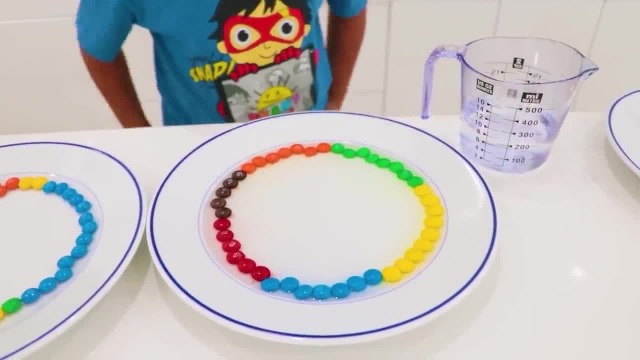 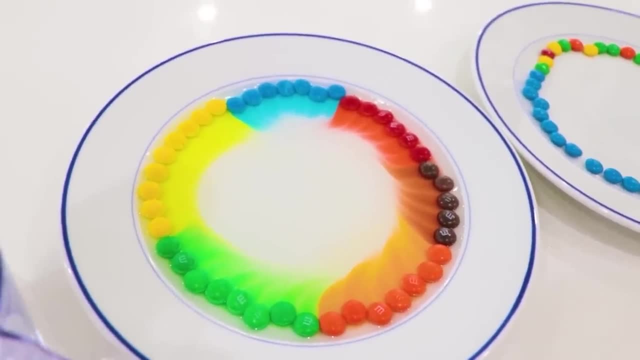 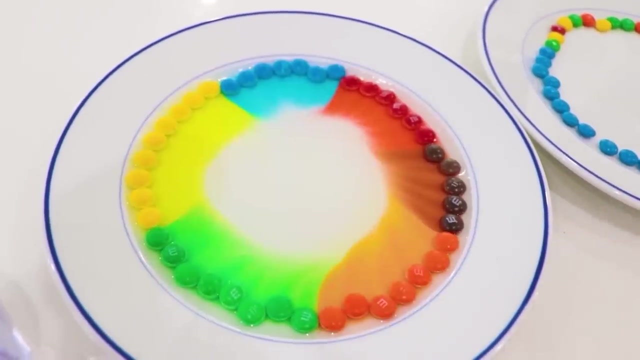 Warm water right here Starting. Is it working? Yeah, it is. Whoa. Do you see the difference between the M&M's and Skittles? Yeah, the M&M's like twist. It looks so cool, Aww. 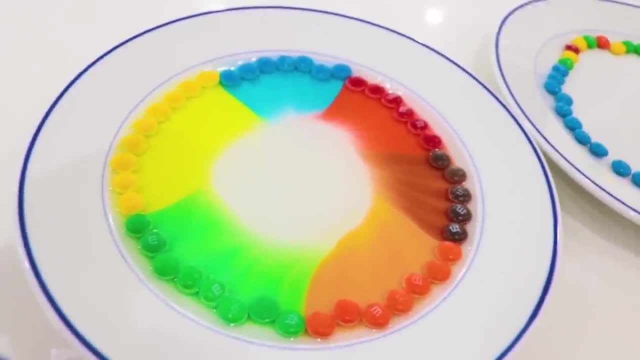 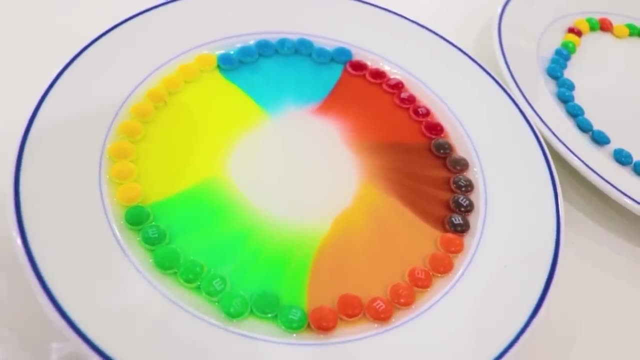 Do you feel like it's the same speed or you feel like it's different speed? It's different speed. Do you think it was going slower than the Skittles or faster than the Skittles? I think faster than the Skittles. 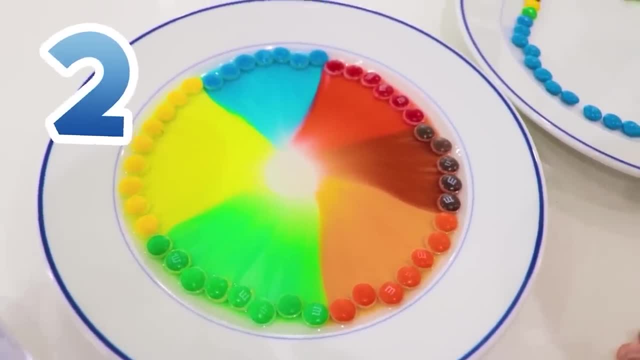 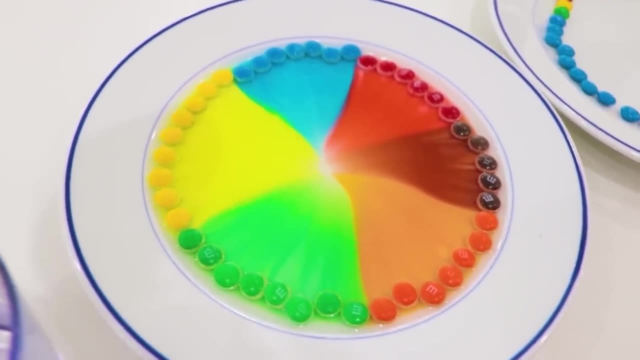 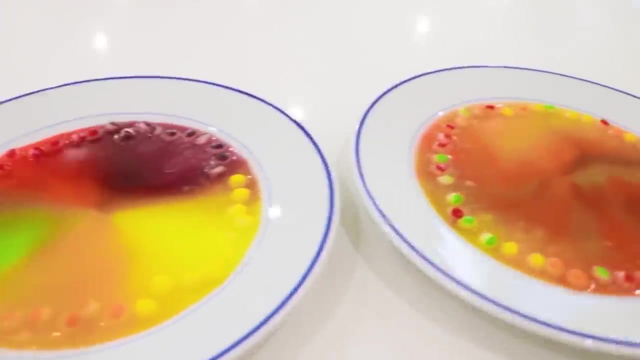 Three, Two, One, Bye, Bye. There you go, guys. M&M's. Which one do you like better, The M&M's or the Skittle one? So we've been letting these sit out for a while, so it looks super different. 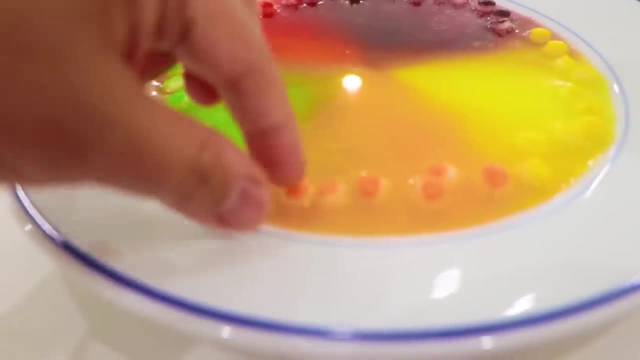 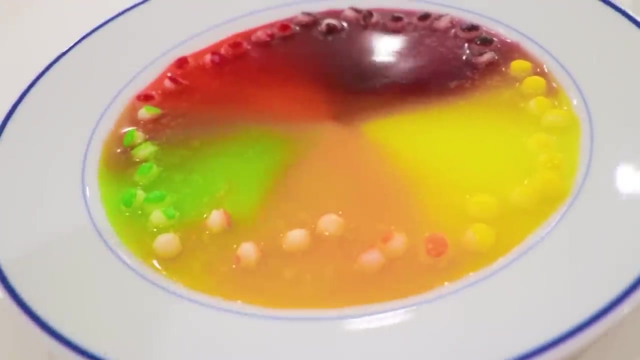 Everything is coming together there And here. if you guys look, it's all the little M&M pieces on the back. It's all white now. so, instead of the color, they're all white, Do you see? Because all the colors are coming out. 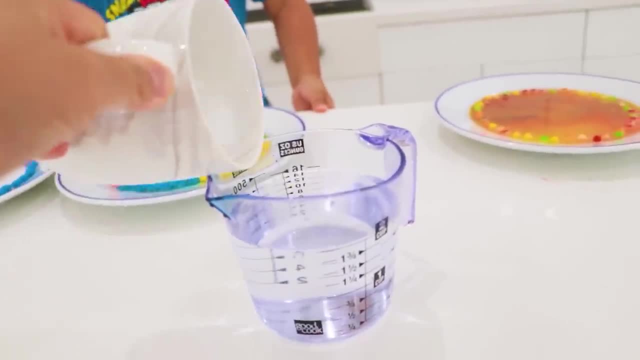 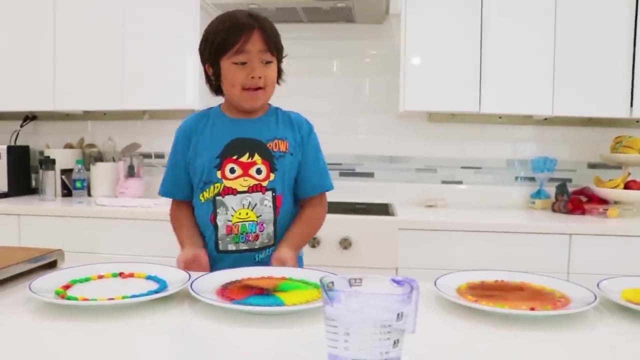 We got regular water from the sink and now we're going to add ice to it to make it ice cold. Ooh, Wait for like one minute. That's right, Ryan, To make the water cold. yeah, Okay, I think it's ice cold now. 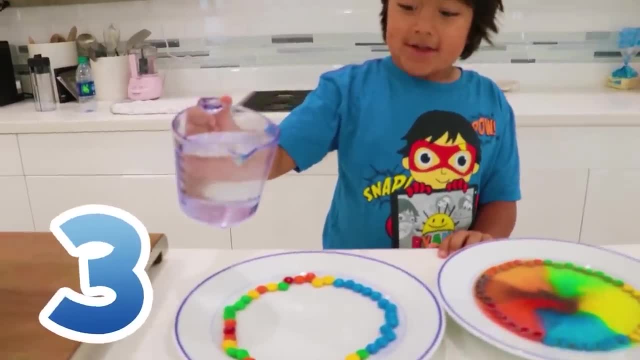 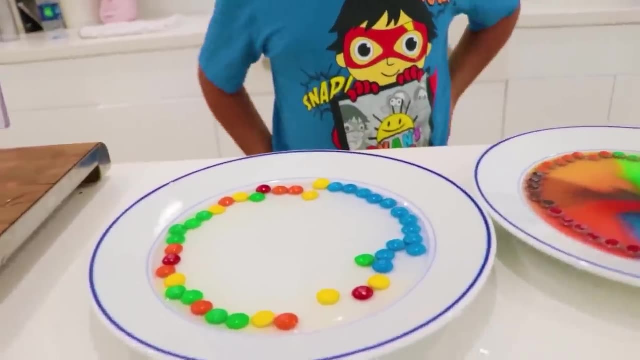 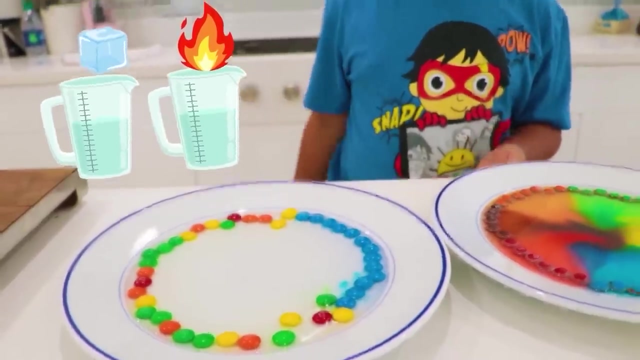 Ooh, Three, Two, One. While we wait, do you guys think it's going to dissolve? Good question, Ryan. What do you think? Do you think the cold water or the hot water will help it dissolve faster? I think the hot water will. 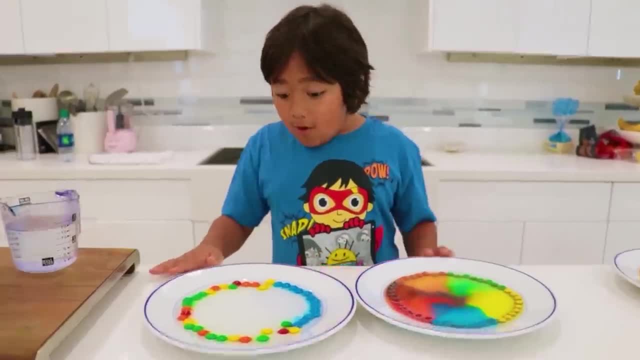 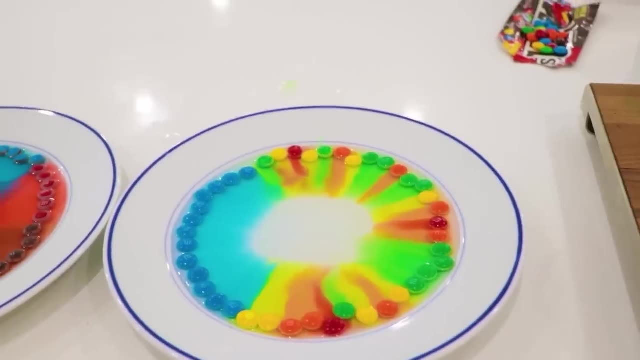 dissolve faster. Okay, let's check it out and see. Wait, It's working. Well, if you move it, it goes faster. We'll wait and see what happens. There's the cold water. as you notice, I think it's going a lot slower. 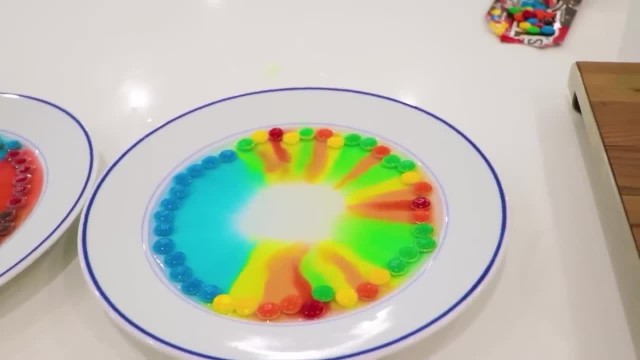 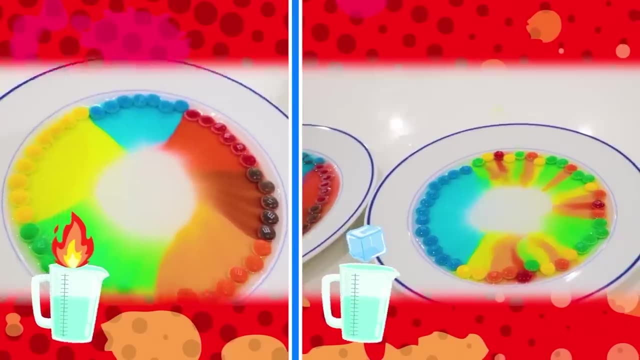 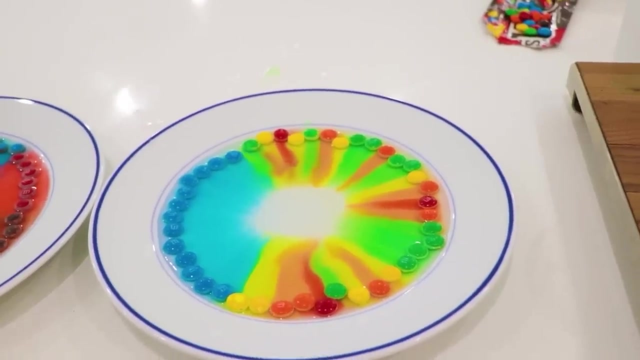 Yeah, We're waiting for a while now. It's still working, Yeah, But it's just not going as fast. Wait, We're waiting. What happens? if you like, blow it. That's a good question. Why don't you do it? 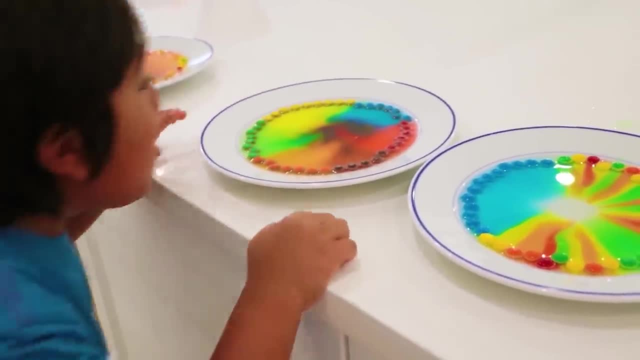 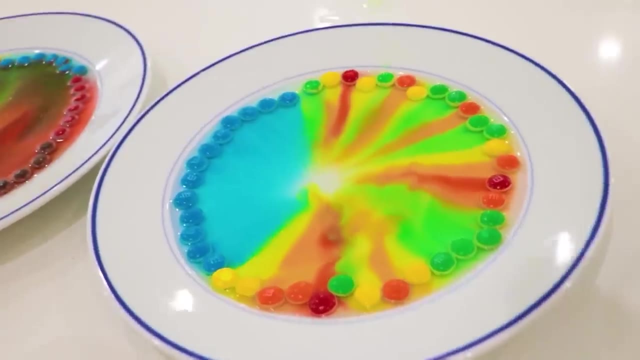 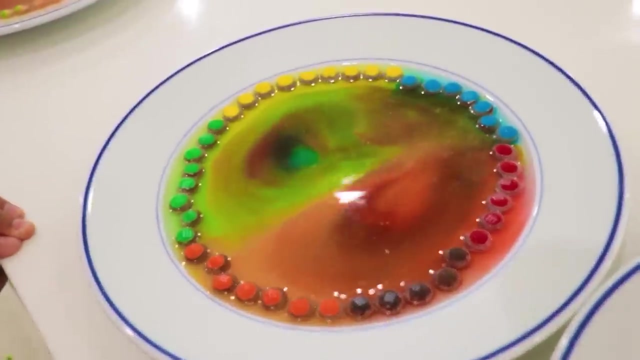 Oh, it doesn't change it, It just changes the water. Okay, so this is still going. Whoa, So it changes the cold water. Wow, It's mixing it all together. Whoa, It's creating like a galaxy color. 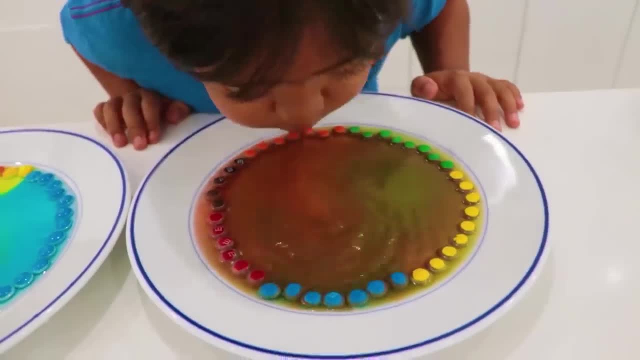 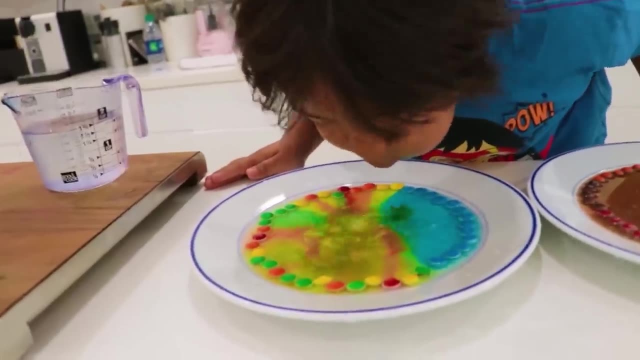 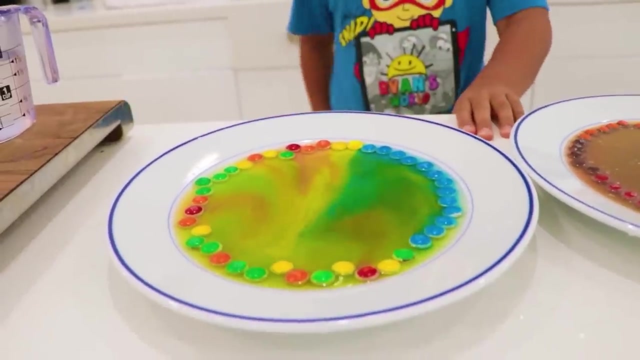 Whoa, That looks cool. Whoa, Oh, the other one looks cool. when you mix, You can try to blow that one too. Now it's all mixing together. It's like a tornado when I blow it. I know. 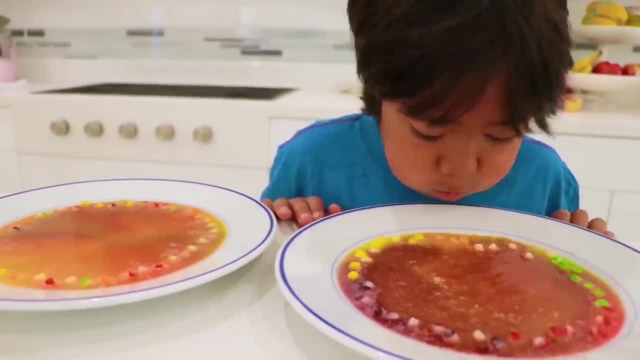 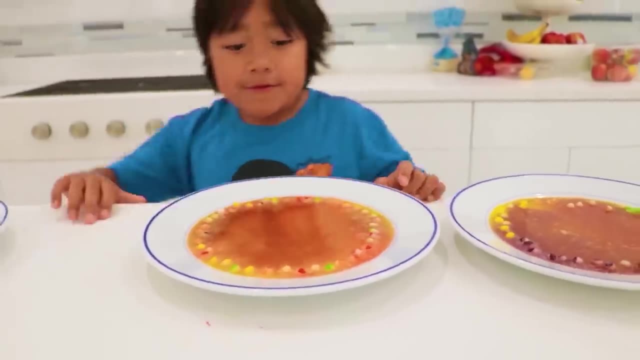 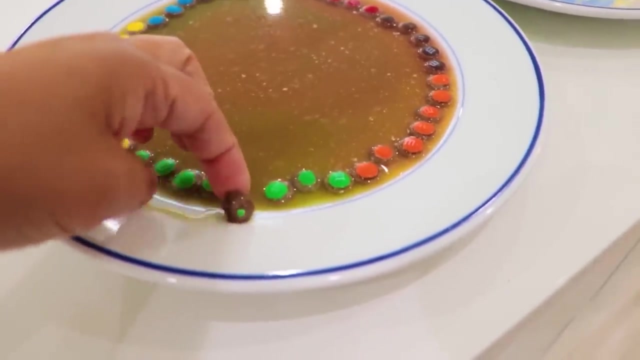 Ryan's trying to spill. I think it's mixing one color. Oh, this is turning orange. Yeah, This is the M&M's here. So it's because it's chocolate. When the color dissolves, you see the chocolate left over. 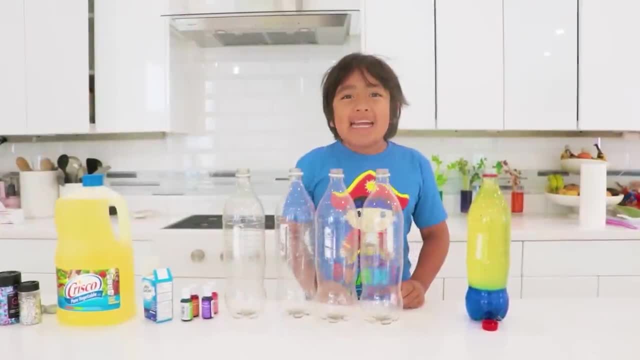 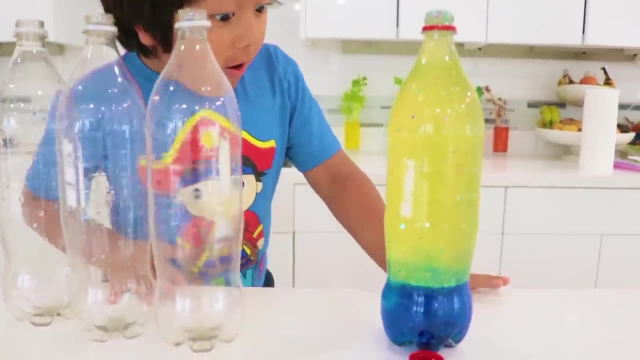 Right, Yeah, and it turns brown. Hi guys, Today we're making homemade lava lamps like this. Okay, so you have to wait a little bit and look what's going to happen. Look, That's cool. You like it. 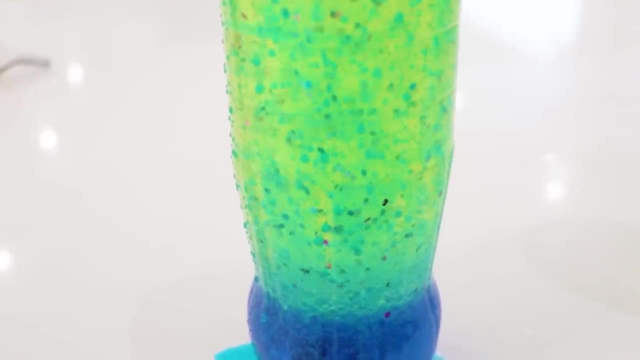 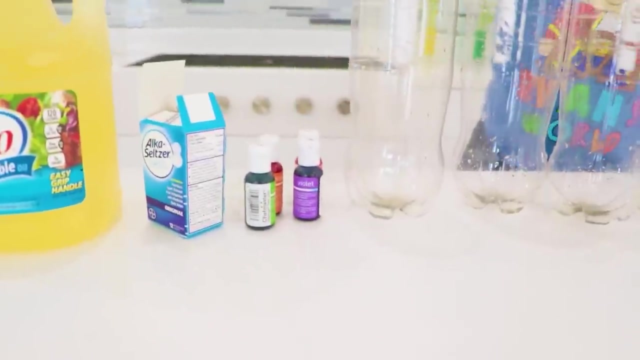 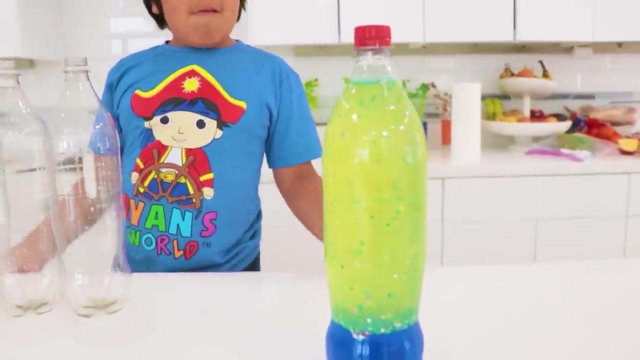 Yeah, So here's what you need: Bottles, food coloring, Alka-Seltzer oil and, optional, if you want it, glitter. Yeah, so this one. we have glitter inside, but you don't need glitter. First step: always ask a grown-up for help. 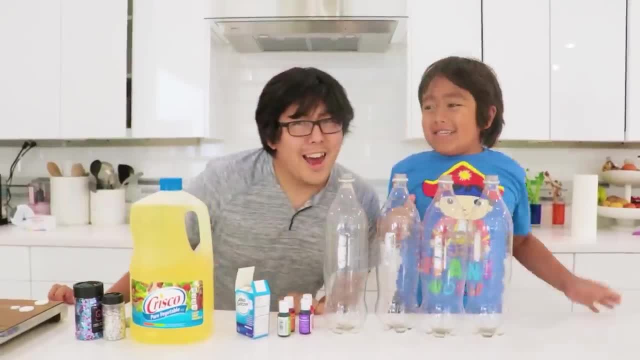 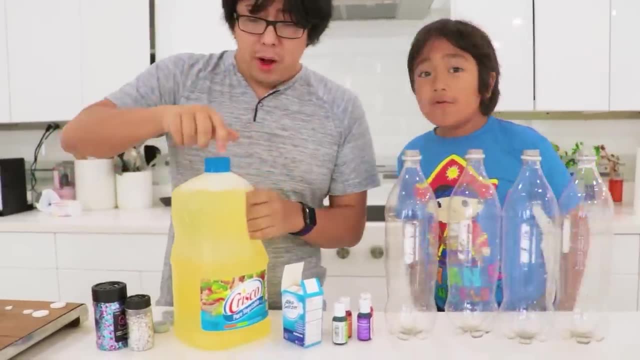 Daddy, What's up, Bryan? Hi? Hey, what you need help on. I need help on baking this lava lamp. Okay, here we go. So we got oil. I need three, four oil in each container. Alright, right on, Ryan. 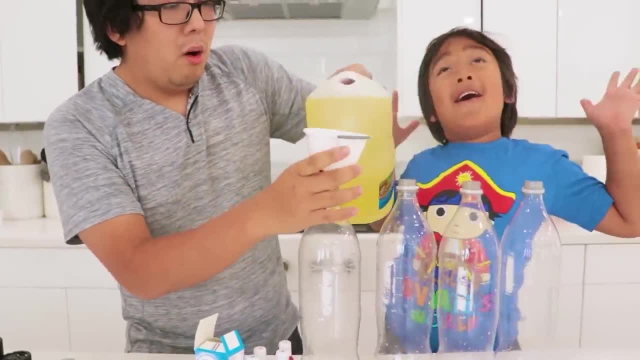 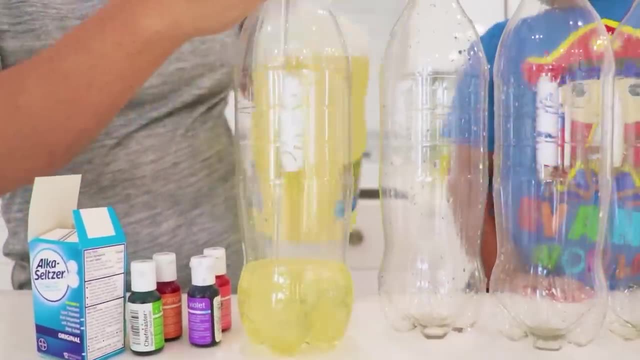 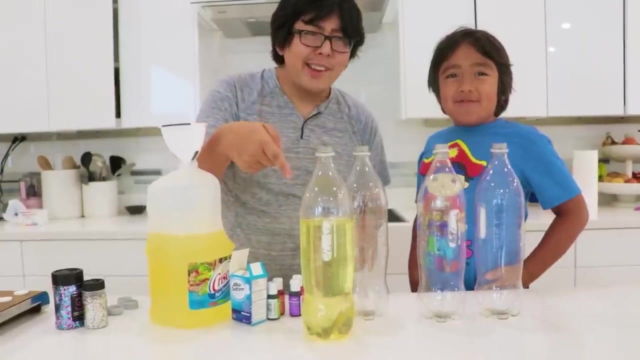 So put the funnel like this. So you want to spill the oil all over? Yeah, Whoa Going in. Yeah, Let's fill it up, Let's go, let's go. You see it coming down. Yeah, One down and three to go. 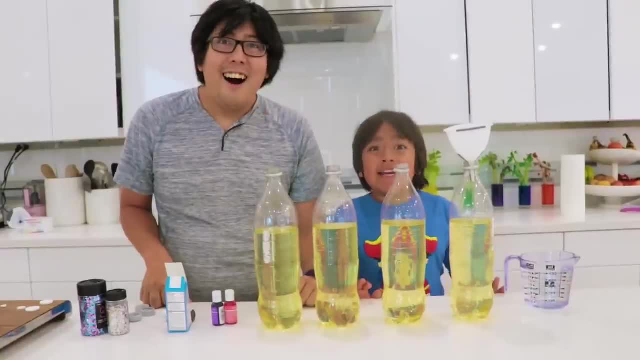 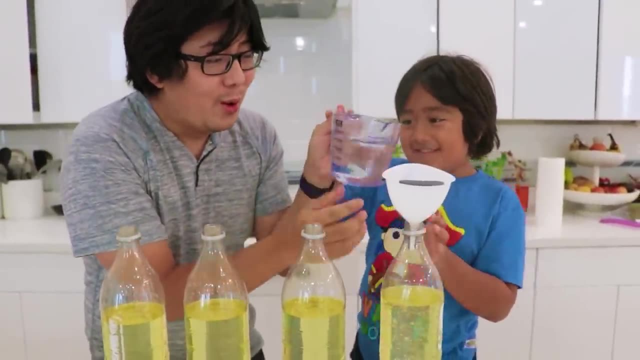 Alright, let's keep going. It's done. Now fill the rest with water. You do that and I'll tell you when to stop. Never mind, I'll do it. I'll do it Always. ask for adults for help. 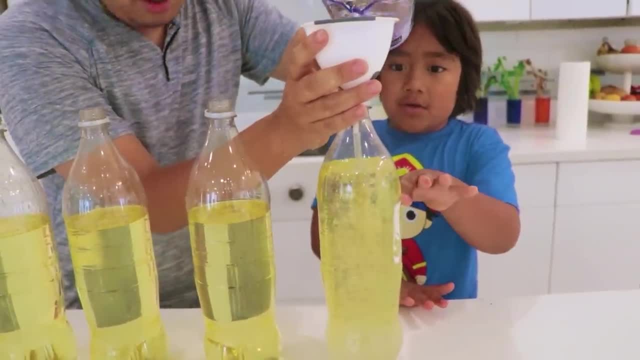 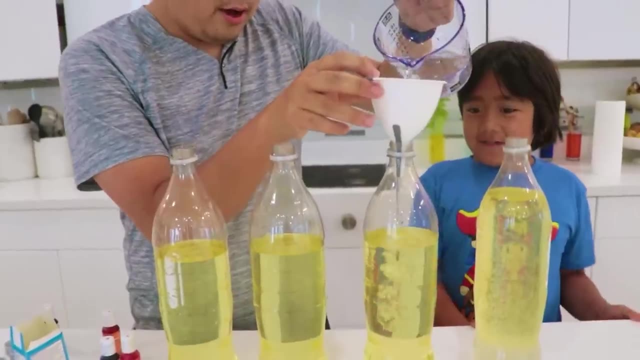 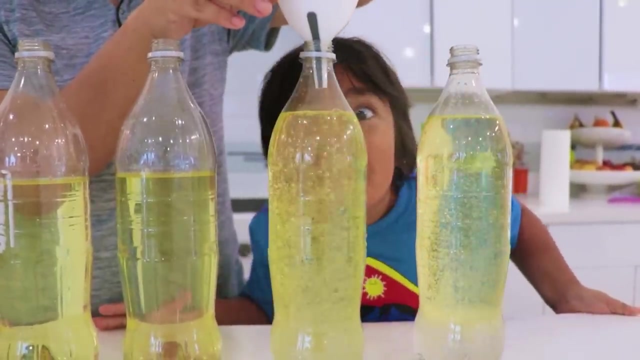 I'll tell you when to stop. Okay, That's good, Perfect, Perfecto. Next we're gonna keep doing. Okay, Ryan, just take a close look and just tell me when to stop Counting on you. You cannot overfill either. 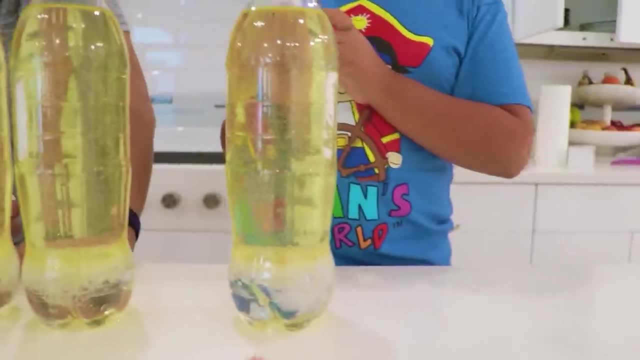 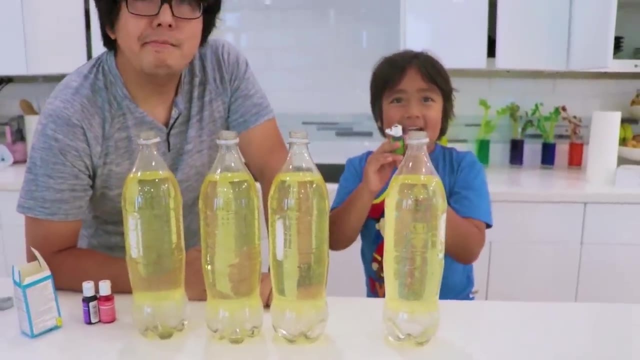 Perfect, We're gonna done here. If you look here, there's two layers: There's water on the bottom and there's oil. So oil and water doesn't mix right. Yeah, Why, Why, Yeah, why doesn't? 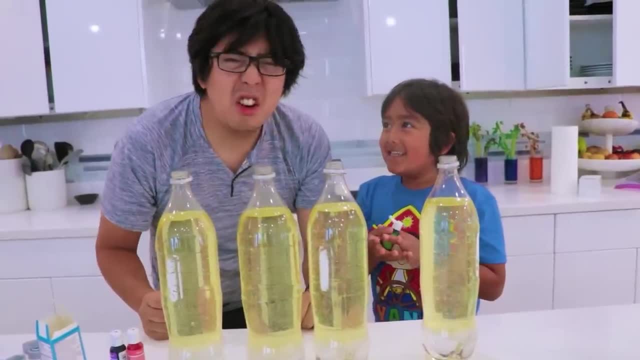 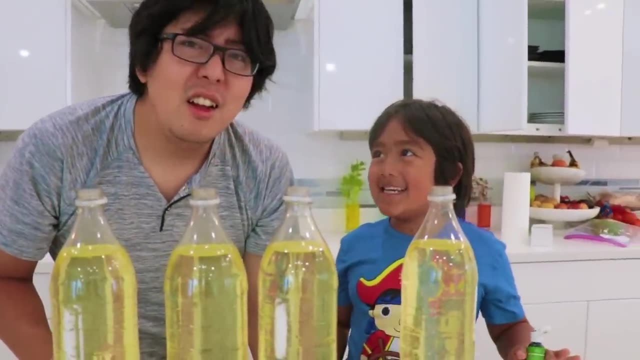 water and oil don't mix, Do they hit each other? Water and oil is just always getting tight. Is that why? No? Because the water's more density? Oh, Good job Ryan. because they have different density, Yeah, water is more dense. 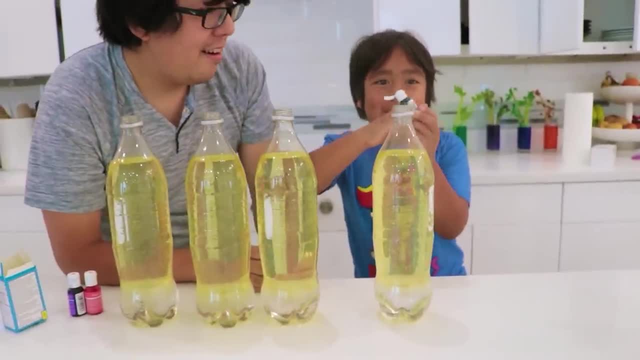 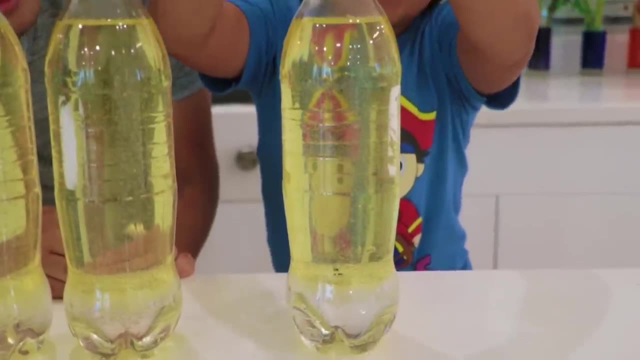 And oil, And now we're gonna put food coloring First. one is green. Okay, maybe 10 drops would be enough. Whoa, you see how it goes all the way down, Like going down. Yeah, let's shake it up. 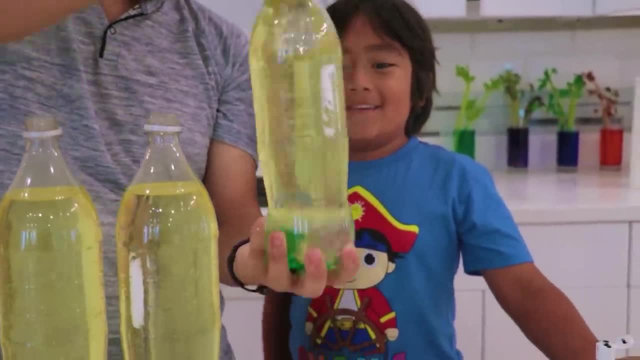 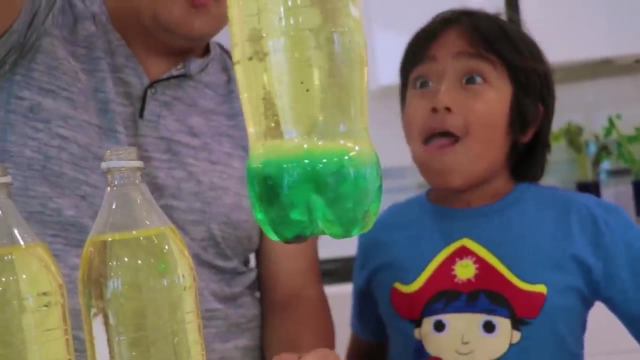 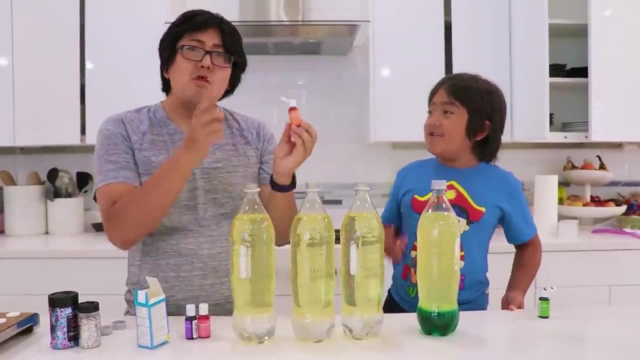 a little bit. just make sure you drop all the food coloring to the bottom. Isn't it interesting how it only colors the water and not the oil? Yeah, What is that? I don't know for real. Next we're gonna do: 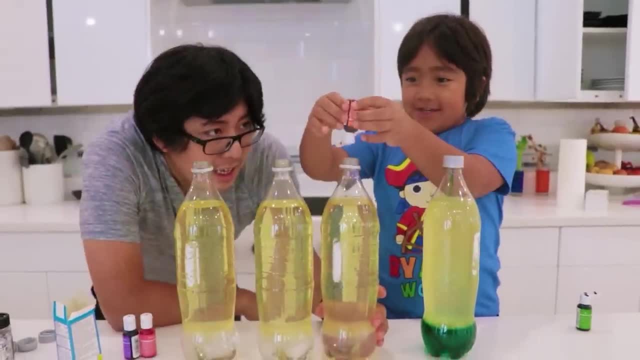 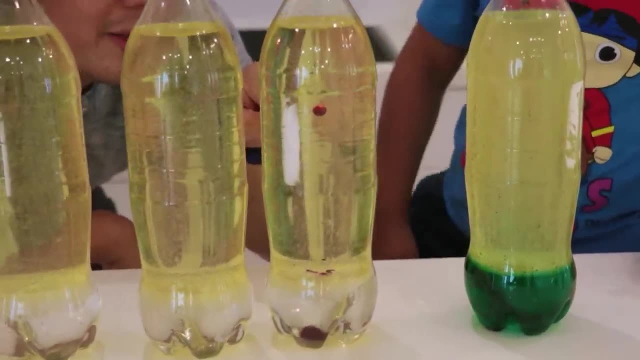 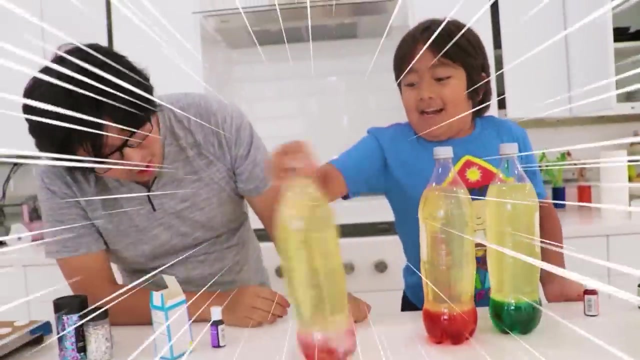 orange Orange, There you go Again: 10 drops. Oh, it's slowly going down. Oh, that one's just staying there. Is it gonna go up? Hey, go ahead, go ahead, Do it, do it, do it, Perfect. 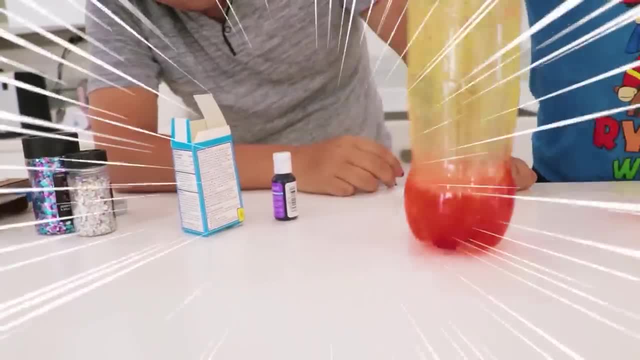 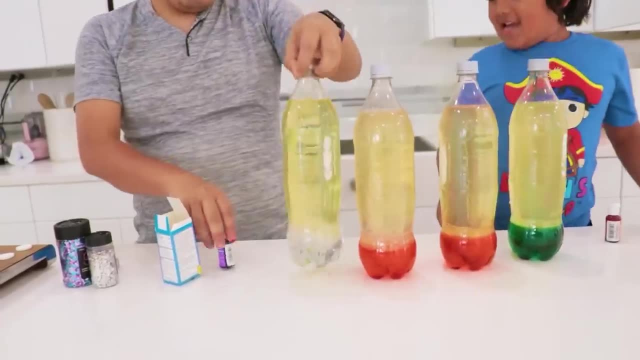 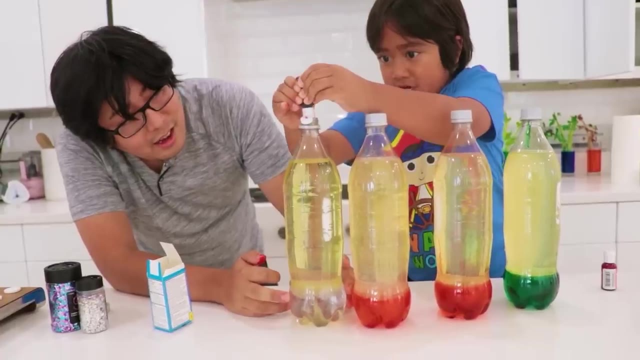 You're doing it better than me. Good job. They kind of look almost the same. Yeah Yeah, pink and orange look the same. Last one: Purple Is purple Purple. This one works, Hopefully. There you go, there you go. 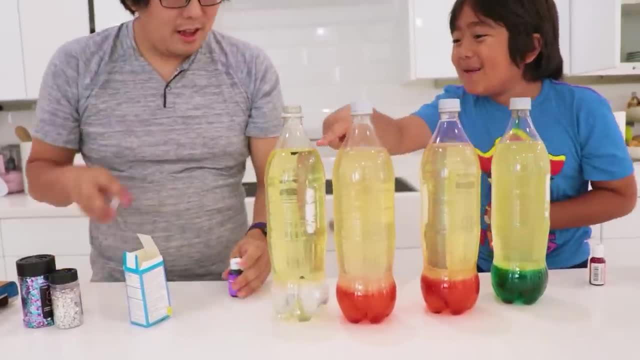 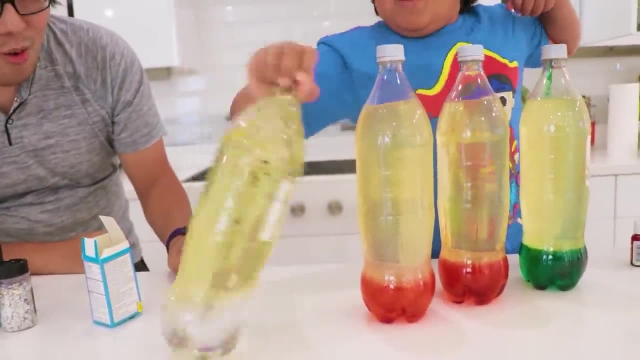 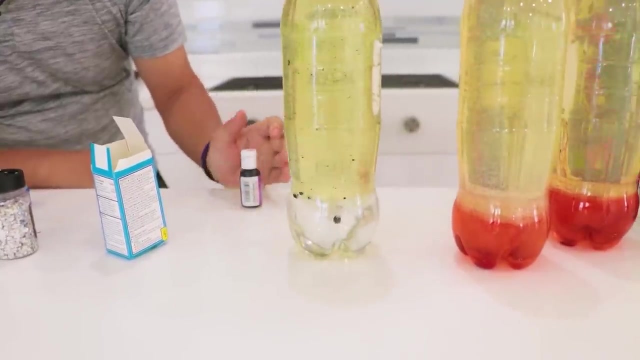 Alright, good job. Oh, they're floating. You gotta get that down. Ryan, Mix it up, please. Okay, Whoa Cool. I don't think it's enough There, there, Stubborn, I don't wanna go down. 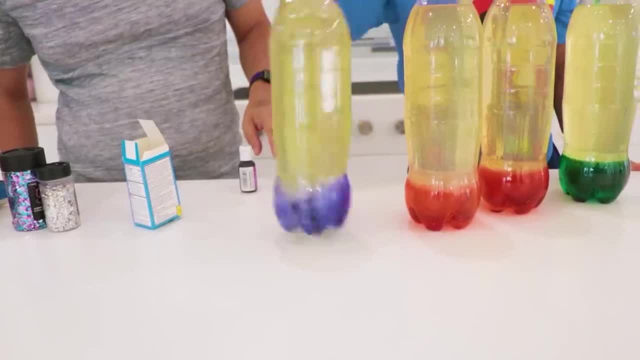 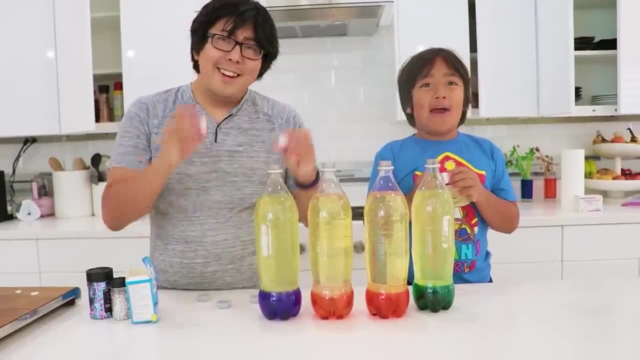 Let's go. let's go. Good, good, It's working. Ryan Whoa, Look at that Nice Perfect. Next step: Alka-Seltzer. Okay, so the piece is a little big, so we gotta break it up. 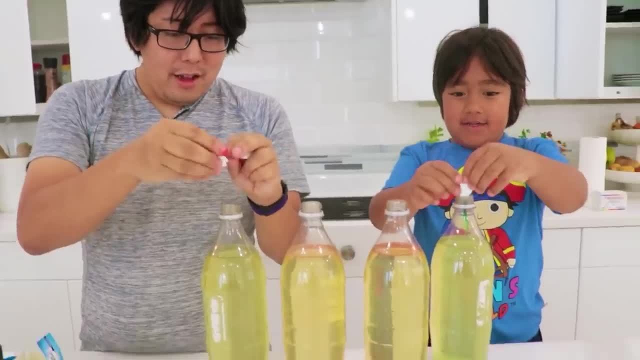 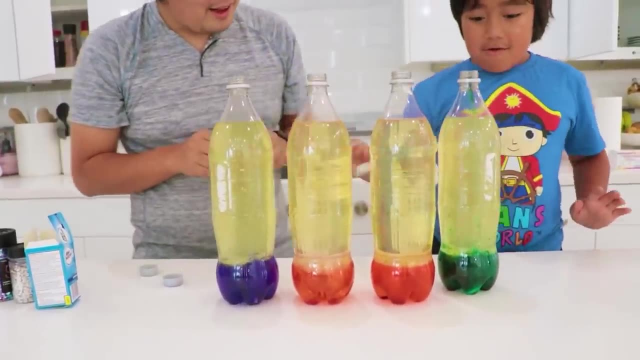 Ah, that's easy. Oh, good job, Ryan, Let's do it together. Three, two, one go Let's see which one looks cool. Close the cap There, there, Not that way. outside, that way. 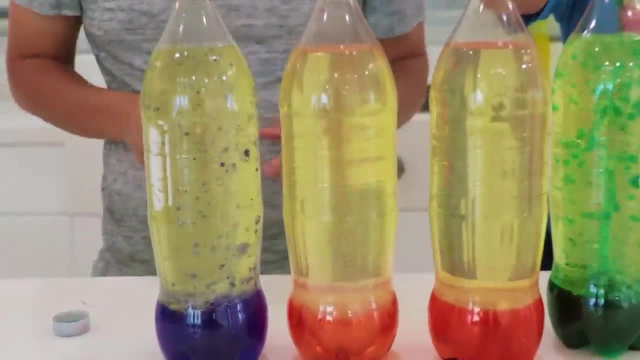 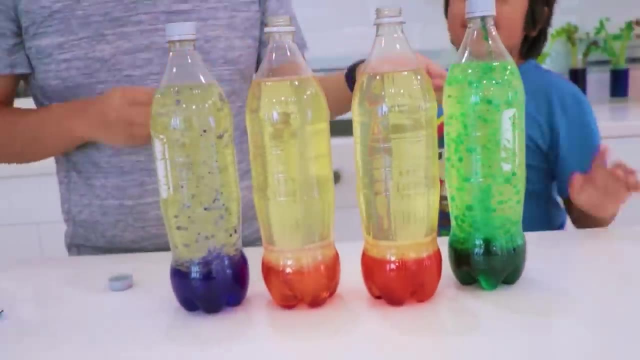 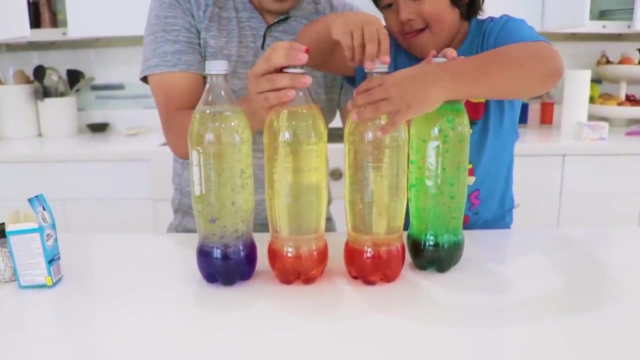 Whoa, it's going crazy. Look at yours, Whoa. Oh, I like yours, Ryan, Whoa. There you go. This one looks good actually. Let's see Cool. Close it before it gets pulled. Ah, I like the orange one too. 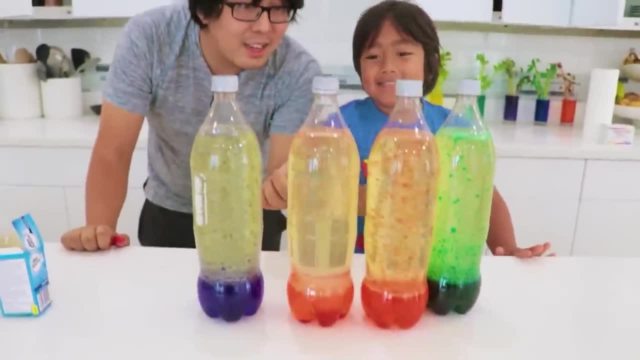 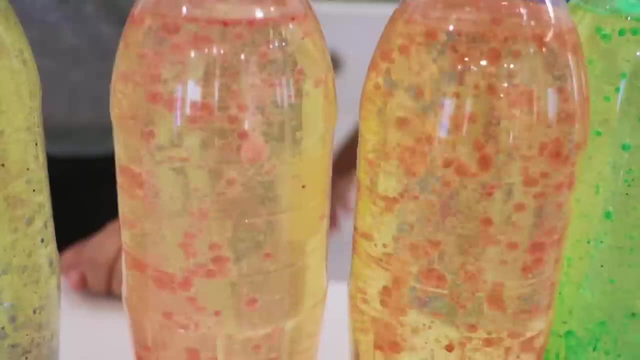 It looks so cool. And the pink one, see, it does look pink. It looks like actual lava. I like it. So when it comes out it looks pink. Wow, I like the orange one because it's actually lava. Yeah, it does look. 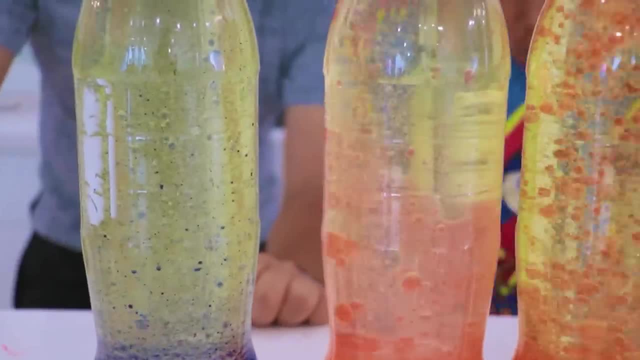 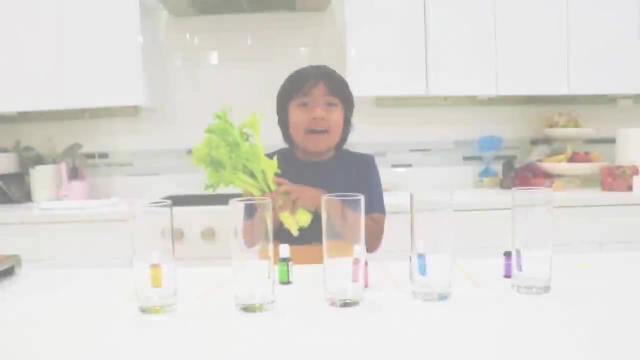 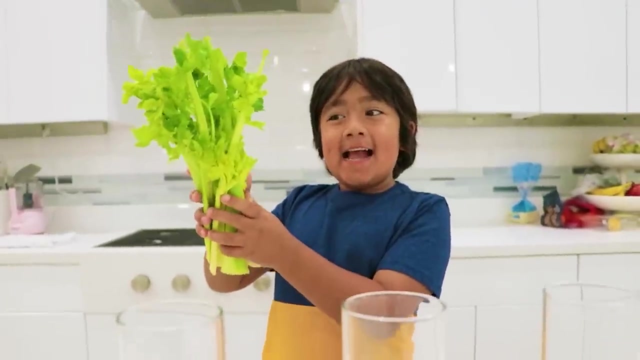 like lava. Nice. There, it is Super easy and simple homemade experiment. Hi guys, Today we're going to learn about how plants absorb water. These are celery sticks, Yeah, so plants need water to grow, right? Yeah? Well, we're going to see what happens if we put. 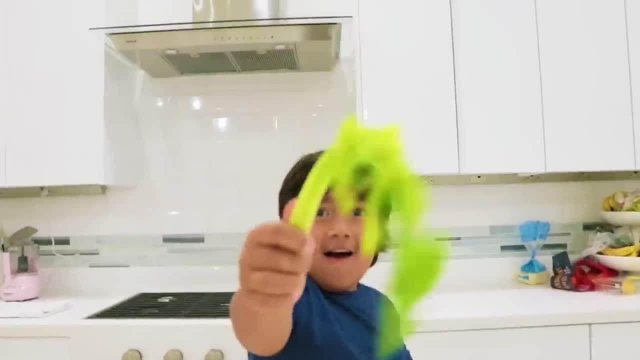 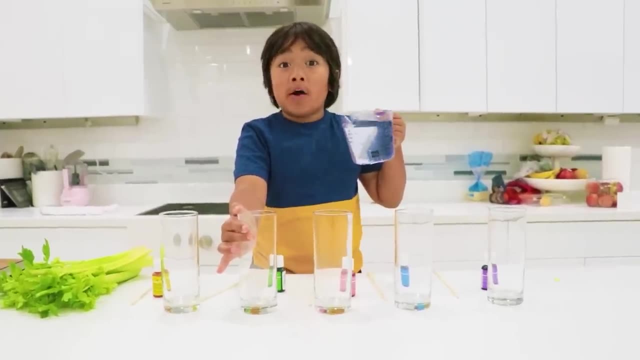 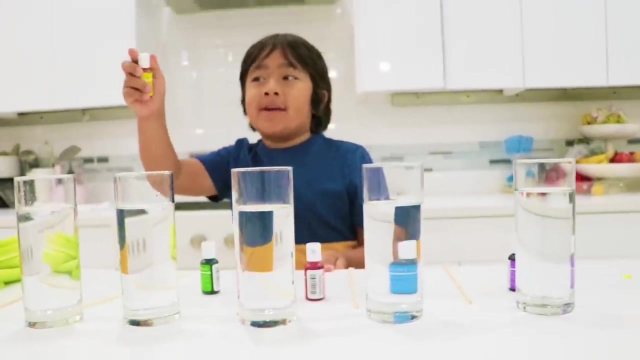 different color in each cup. First step: grab some water. Next, let's pour the same amount of water in each cup. After you fill up the water, let's put food coloring in. First. I'm going to do yellow. Yeah, you can use any color you like. 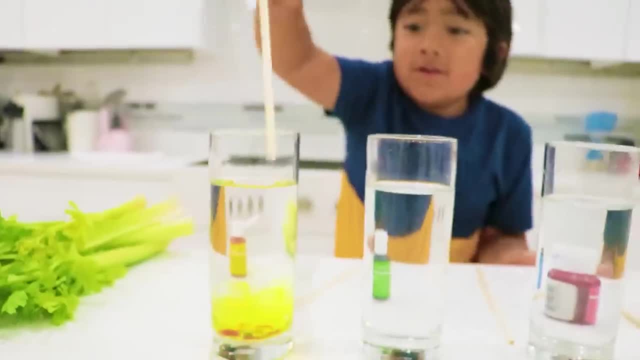 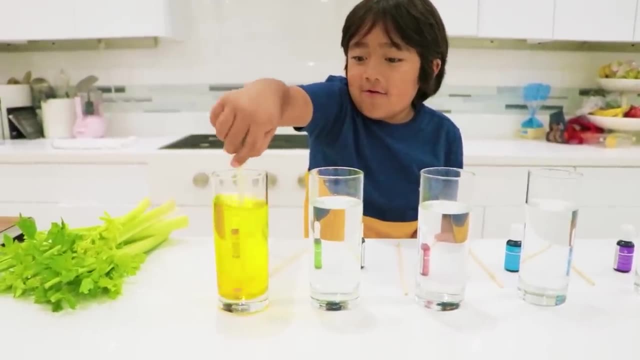 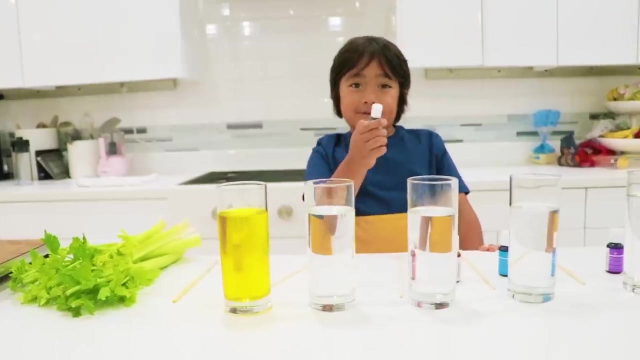 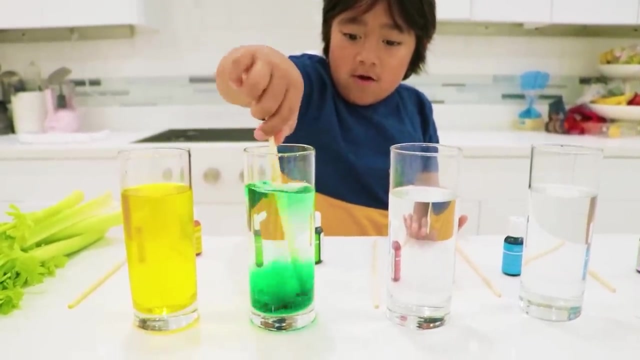 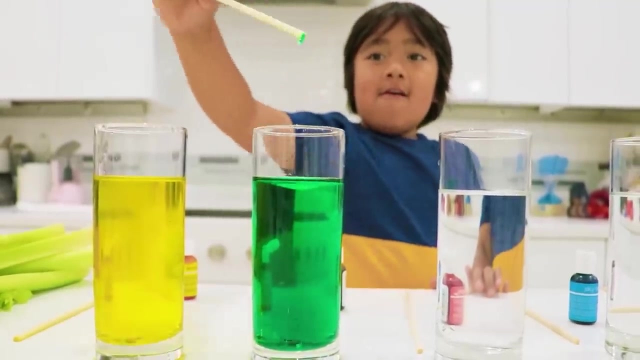 Stir, Stir, Agitate, Agitate. Don't forget to agitate. Oh, it looks like a tornado- It does. Now let's do green Agitate more. Oh, that looks cool. Oh, it's green all the time. 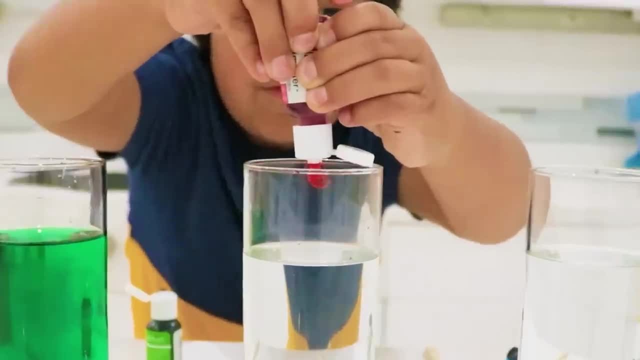 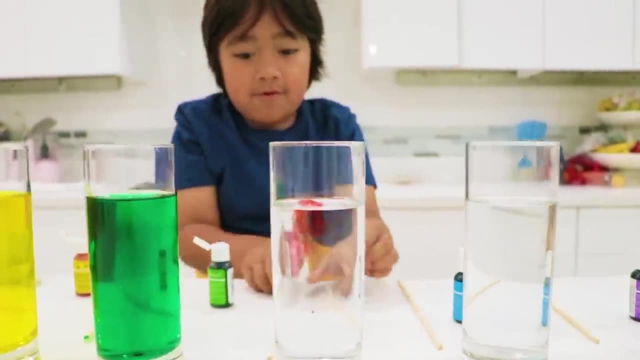 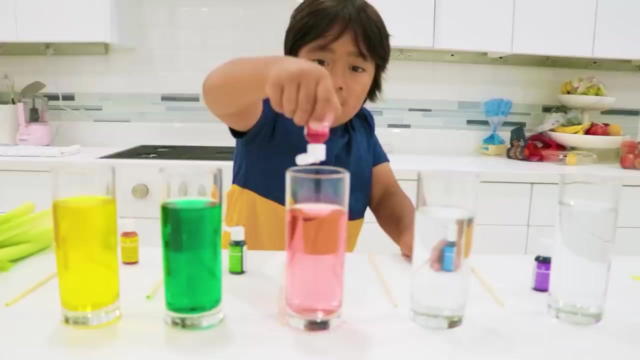 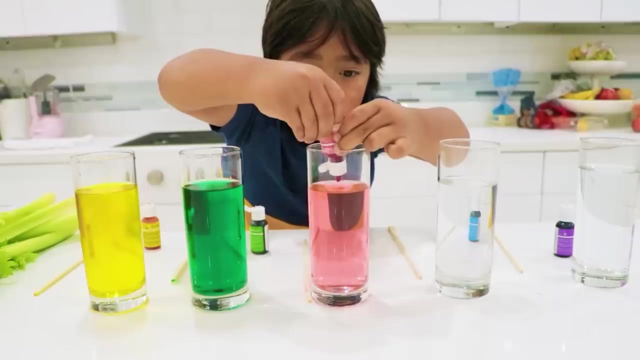 And now we're going to do pink: Agitate, Agitate. Does that work? Agitate. There you go, Cool Agitate. I'm going to add just a few more drops, Agitate, Agitate. Okay, Whoa, this is a lot of pink. 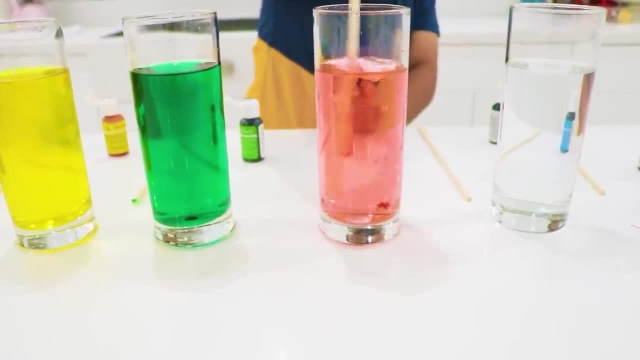 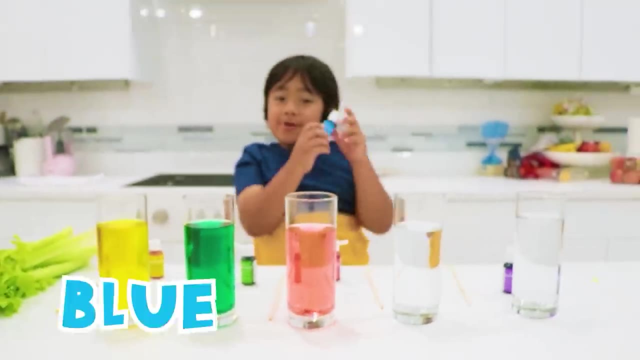 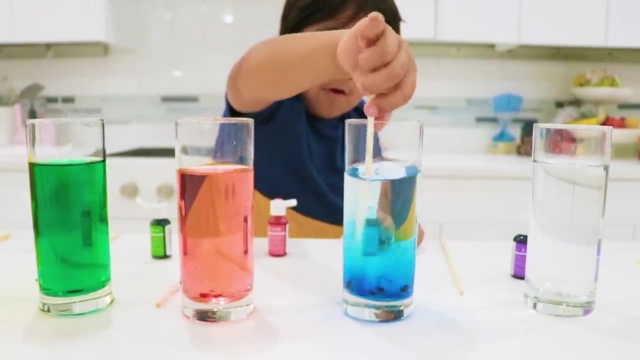 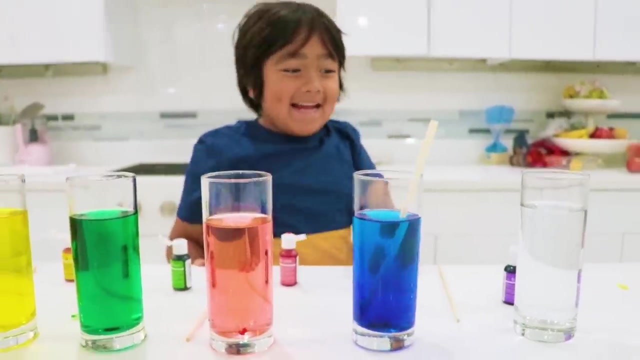 Agitate, Agitate, Agitate. Whoa Okay, now I'm going to do blue: Agitate, Agitate, Agitate, Agitate, Agitate, Agitate. Don't forget to agitate Agitate. What does agitate mean? 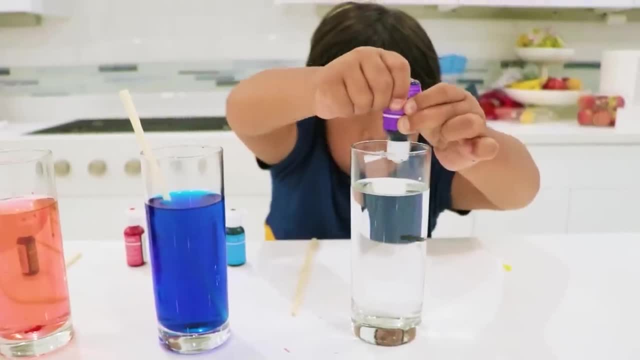 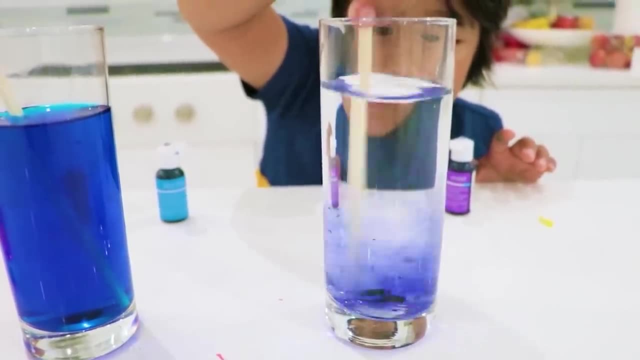 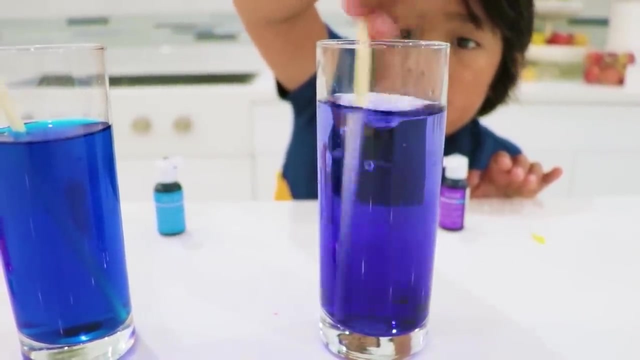 To mix, To mix or to stir. Yeah, good job. Okay, I'm going to hit it. Pow, pow, pow, pow, pow. A little Nice, A little bit more purple, maybe, Yeah, maybe, I think it's good. 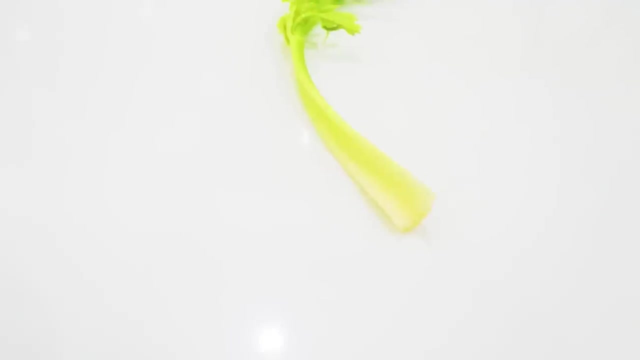 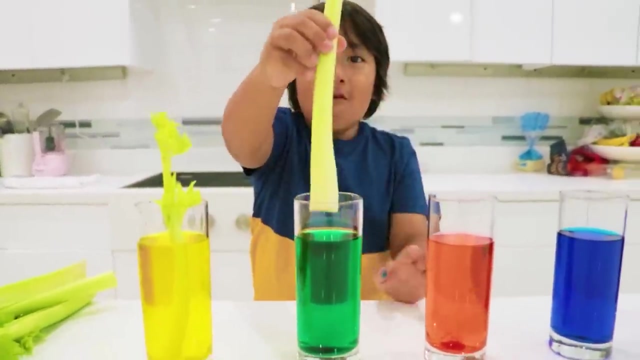 Yeah, good job. Next up, you put the celery into the glass. Before you put it in, make sure you ask a grown-up to cut a little bit at the bottom. There you go, Oh, this one's big, Ha ha ha. 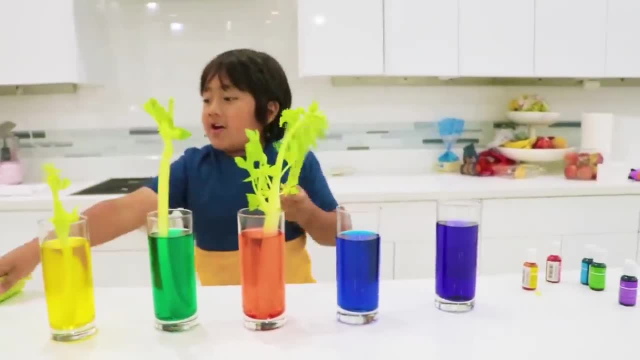 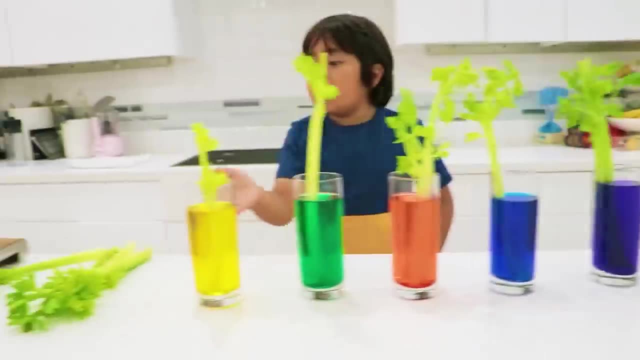 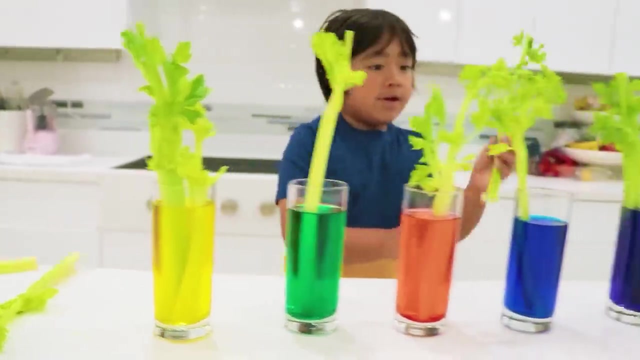 Oh, Oh, ya, ya, Oh, can we put multiple in each one? Yeah, Like that one doesn't have much. Maybe you can put another one in there. There you go, Cool Right here. There it is. So, Ryan, what do you? 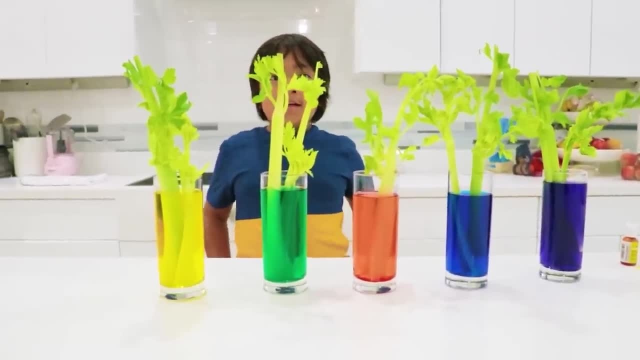 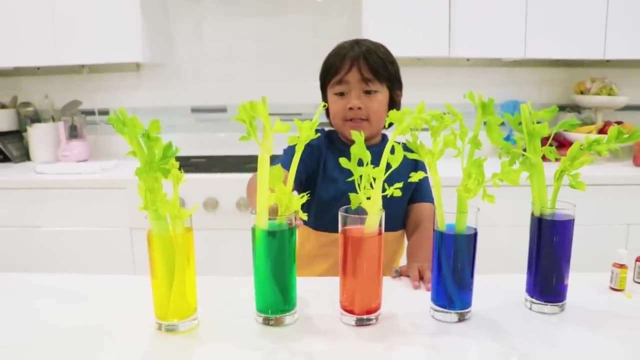 think will happen when the celery absorbs the water. What's your hypothesis? What do you think? I think the celery's going to like turn into that color- Oh really- And some of the water's going to like go away. 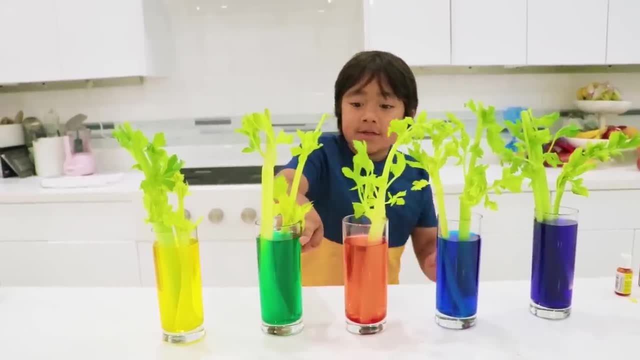 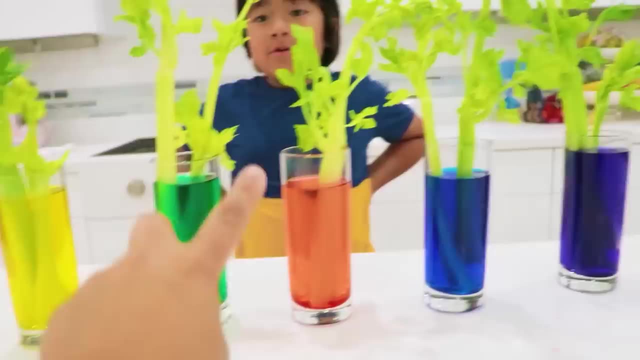 Oh, so you think it's going to absorb the water and the celery will change color. So the glass is going to go like to this much and the celery will change color. Oh, So then if the celery is in a blue, 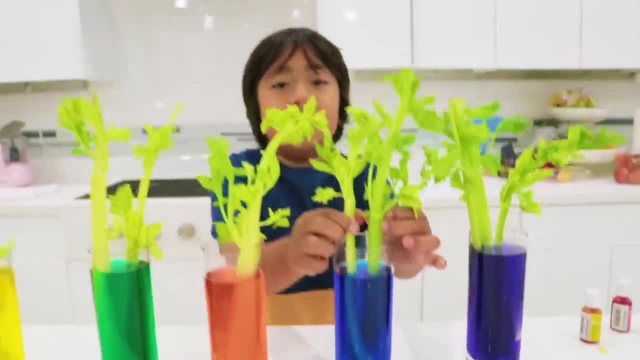 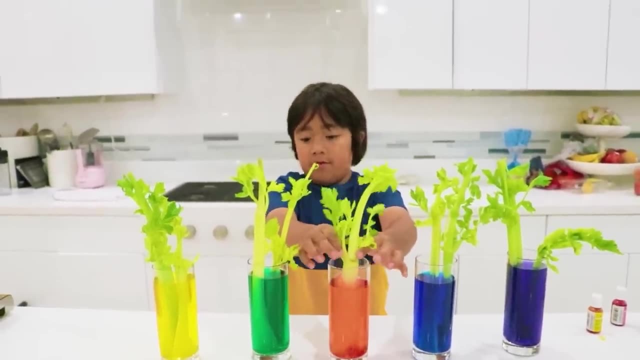 water. what color would it be? Blue, Blue, Ooh, okay, We're going to see if Ryan's hypothesis comes true, So we will be back tomorrow. Hi guys, So it's been a day and here's the results. 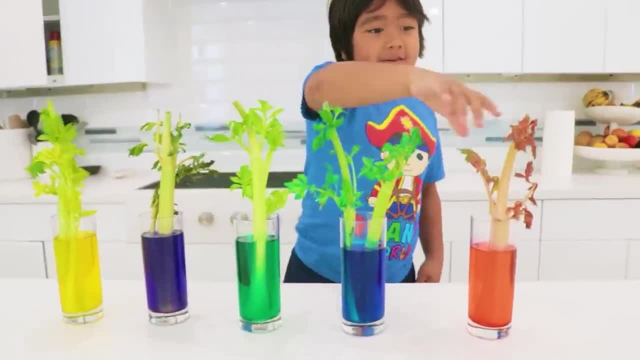 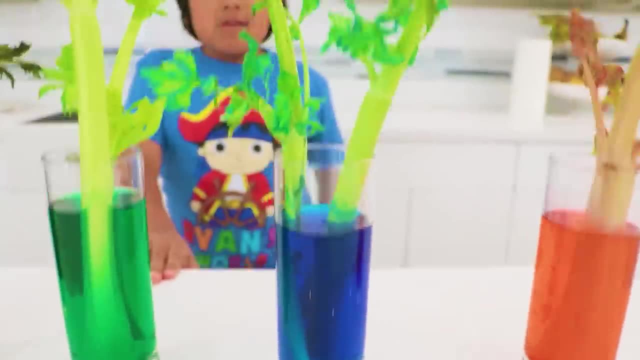 So what's happening, Ryan? So they're turning a little bit of the color, You see, Yeah, so you see the orange and the leaves are turning orange, And then here's the blue one and some of the leaves. So I don't think these are going as 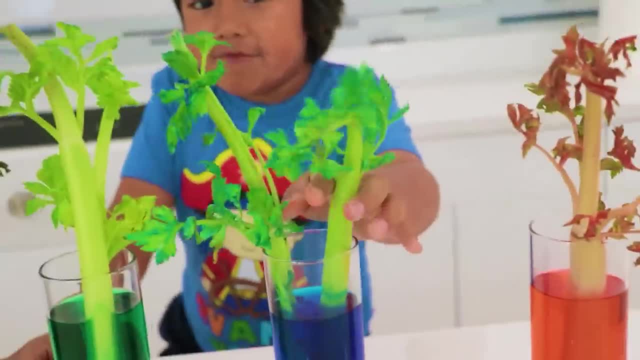 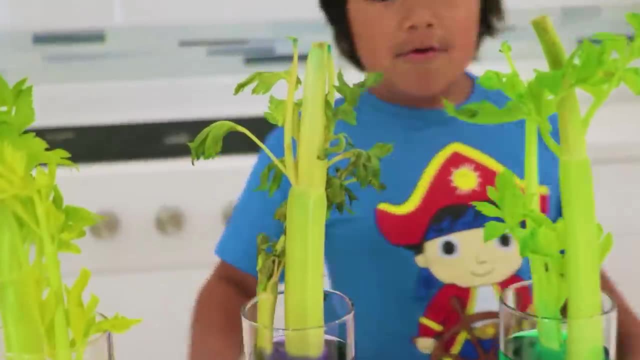 fast, because this one only has one. Yeah, Because these have multiple colors. Oh, you think that's why Maybe This is green, so some of the leaves are turning green, Yeah, And then purple- It's getting there, Some purple. 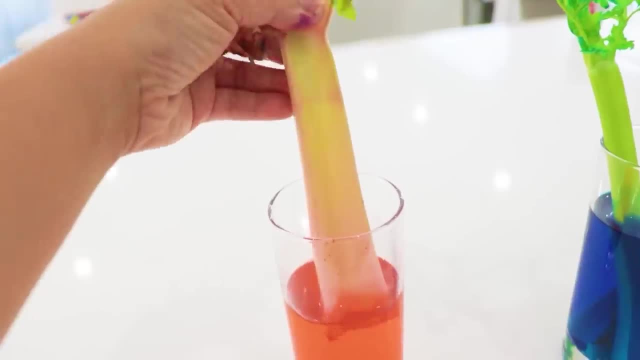 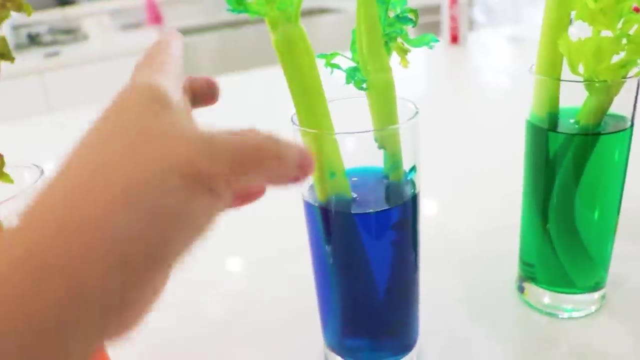 and then yellow. Yeah, it's yellow If you pick it up here, not only on the leaves but also on the stem too. You see orange there. So you guys notice here that the water from the cup has to travel upwards. 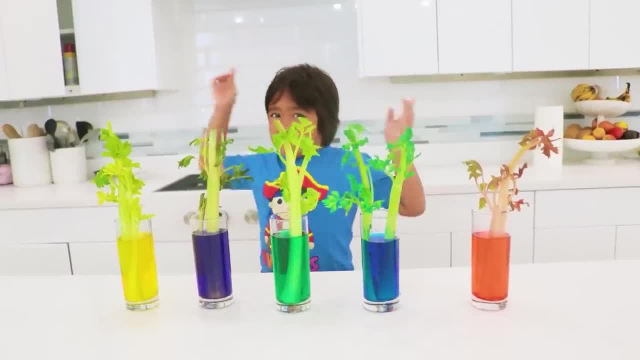 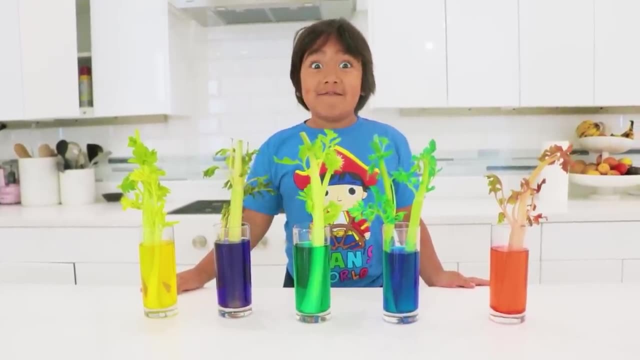 to spread all around the plant. Now we're going to leave it here for one more day and we're going to see what it looks like. Bye, See you tomorrow, which is actually in like five seconds. This is what happens on day two. 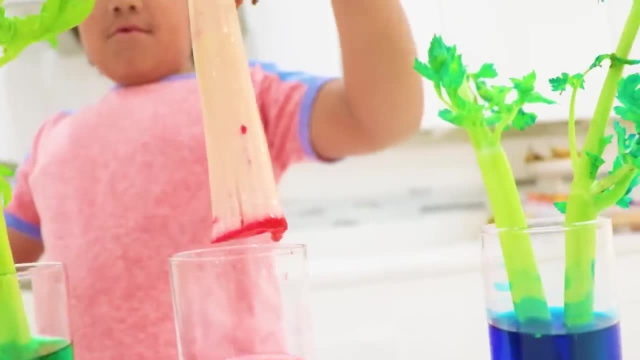 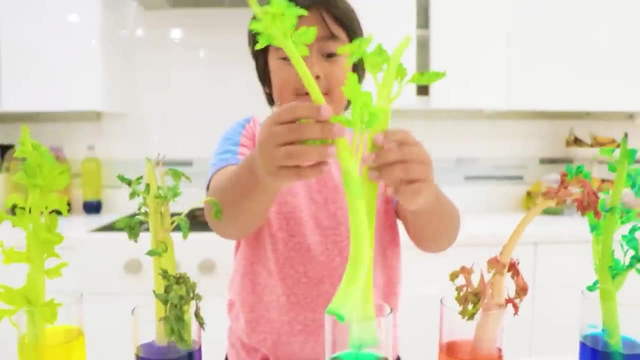 This orange one is really good. It looks like fall And the bottom. do you see how it's also orange? Yeah, it looks pink kind of. And then this blue one looks pretty good And this green one- Green as usual. 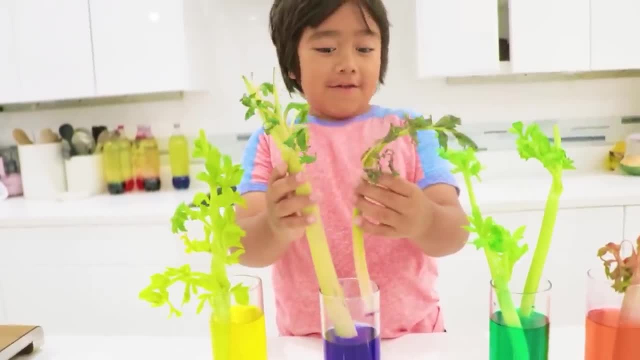 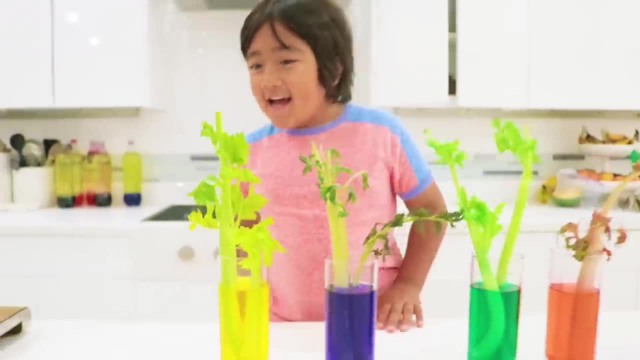 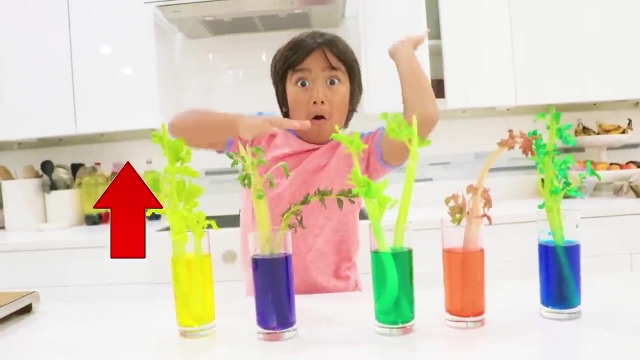 And purple- Whoa, this looks cool. Yellow- Oh, the leaves did turn yellow, huh, Oh, yeah, Yeah, so it's really cool to learn about how plants are able to move the water from the bottom all the way up, right. 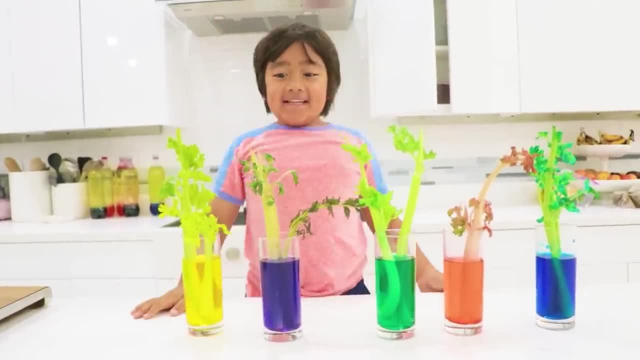 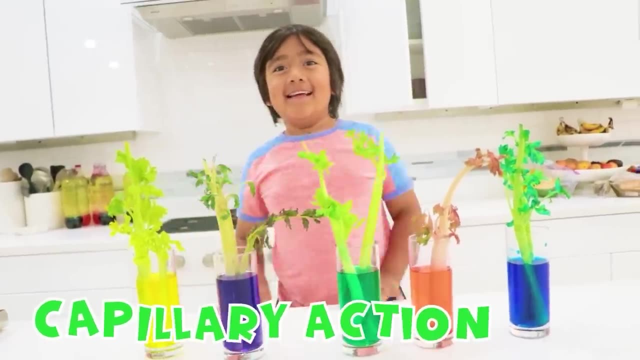 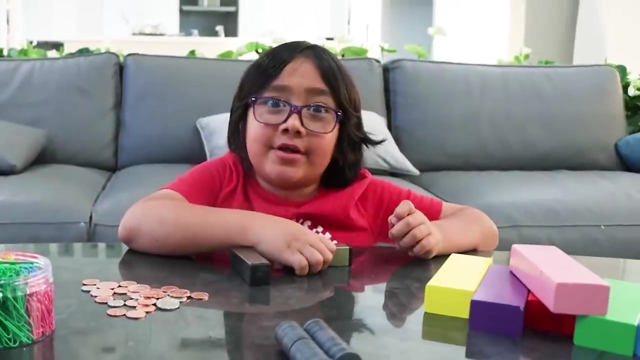 Against gravity. You know what that's called, Ryan? That's called no gravity, No gravity. That's called capillary action. What Capillary action? Capillary action, That's right, Hey guys, today we're going to learn. 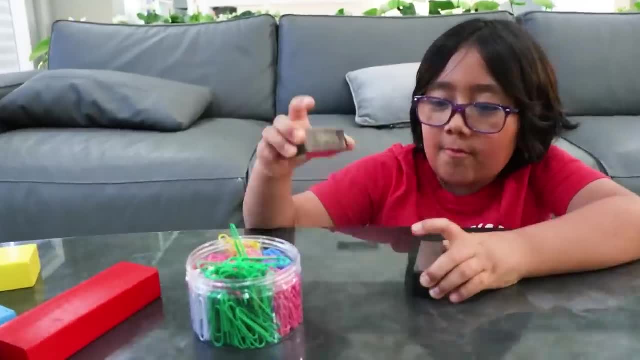 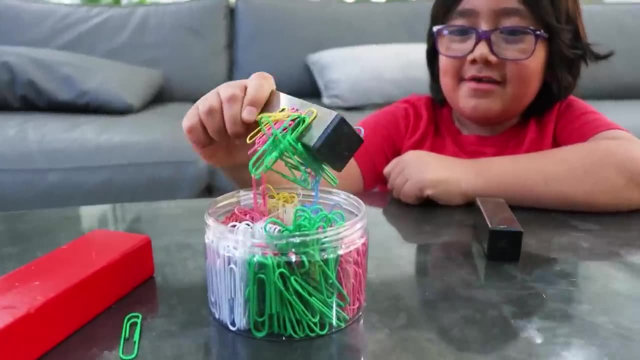 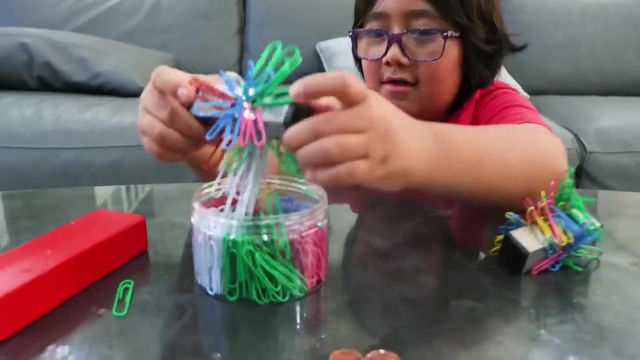 and play with magnets. Alright Ryan, first I wanted to see how many paper clips you can pick up. Okay, Oh, oh, oh, I got a lot. Oh Oh, oh, that's pretty full. You can see all the paper clips sticking on the magnet. 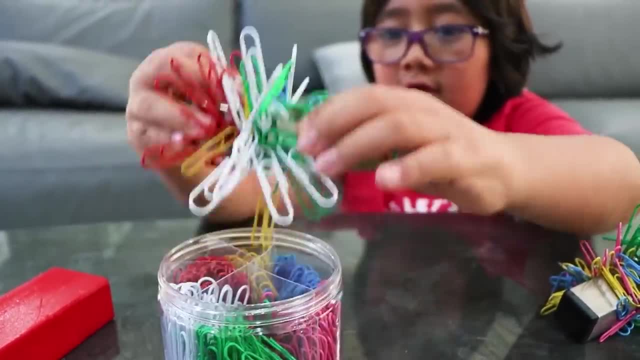 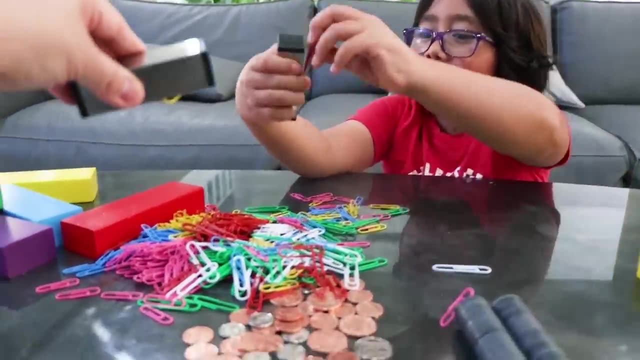 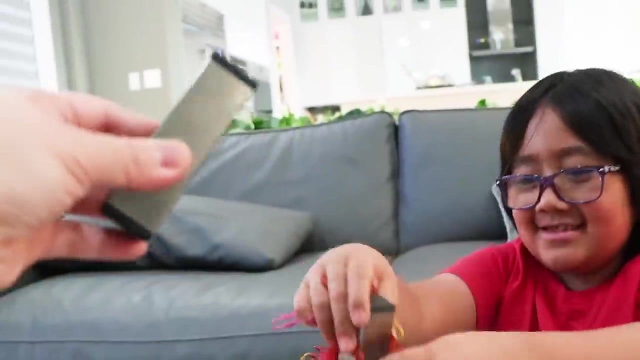 Whoa Looks crazy, huh, Yeah, Okay, we're going to do it together. You ready? One, two, three Whoa, Oh, oh, oh, Alright, it's sticking to each other, It's magnetized. 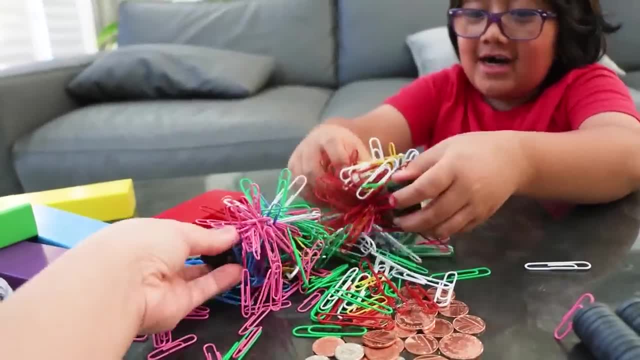 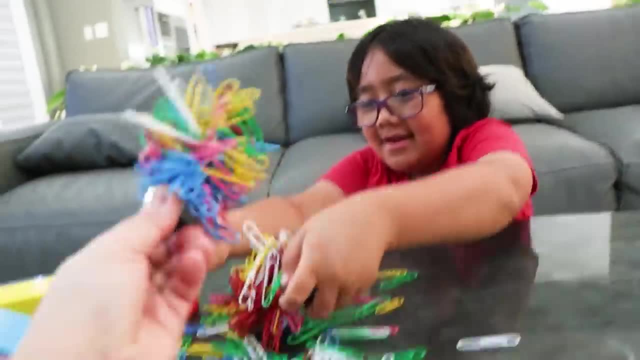 See who can pick up more. I can pick up more. Look at mommy here. Oh, you got a lot, Yeah. So a magnet always have like a positive side and a negative side. So I want you to try to put these two. 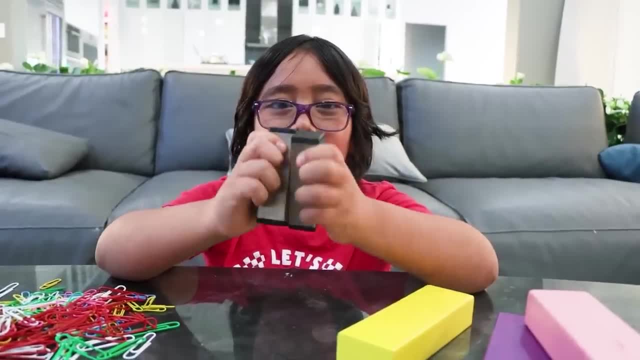 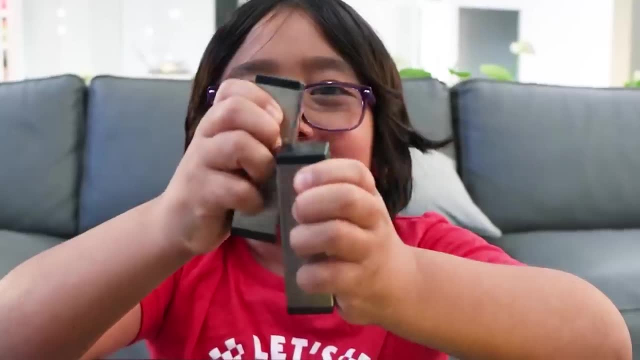 magnets together. Okay, Three, two, one. So that's easy, right? Okay, now I want you to take one magnet and flip it to the other side. Now try to put it together. Oh, this is in possible. They repel each other. 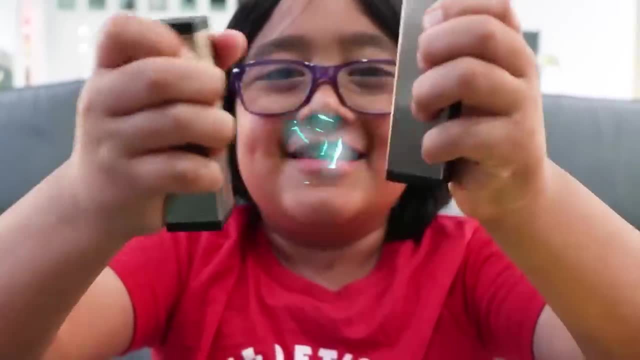 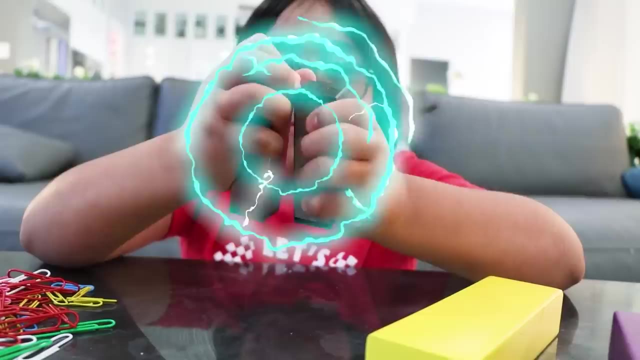 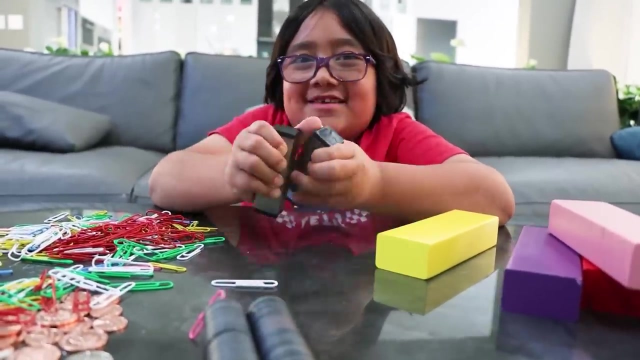 Yeah, there's like an invisible like wall here. Invisible force, Yeah, invisible force. Can you put it together? No, right, No matter how hard Ryan tries, it's not going to work. No, huh, Next I'm going to. 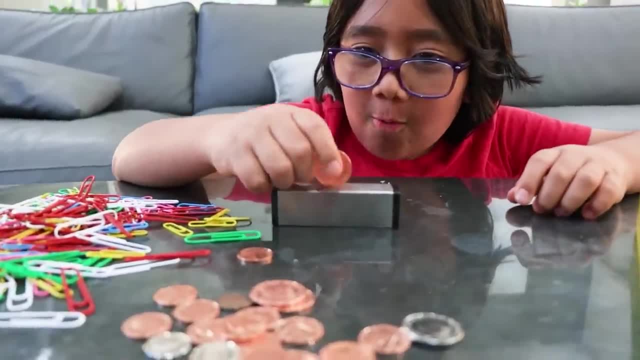 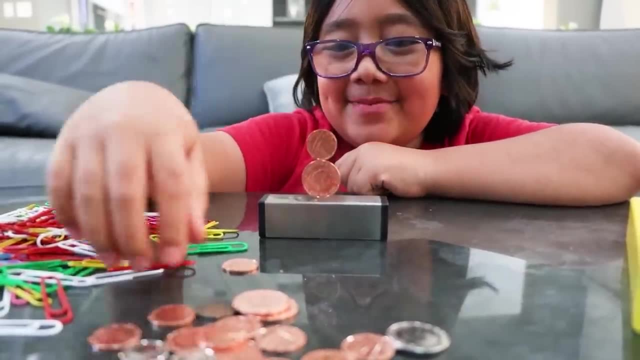 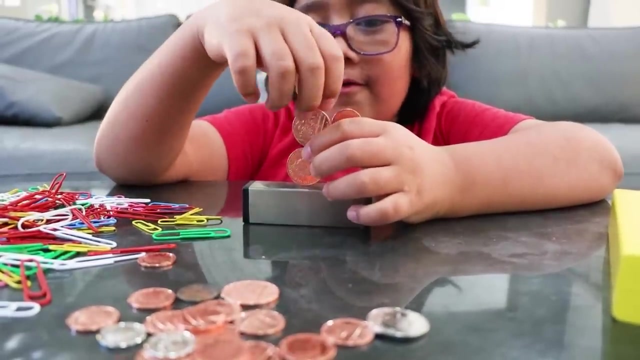 do the penny stacking challenge. Look, Boingy, boingy Stack it up. Whoa Wait, I should do another big one. Oh, oh, oh, oh, oh. So I'll do it like this, And then this: 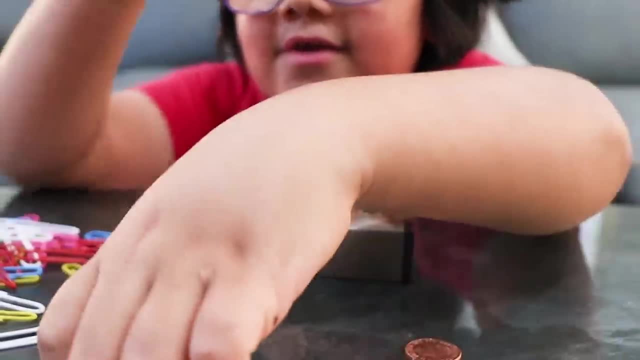 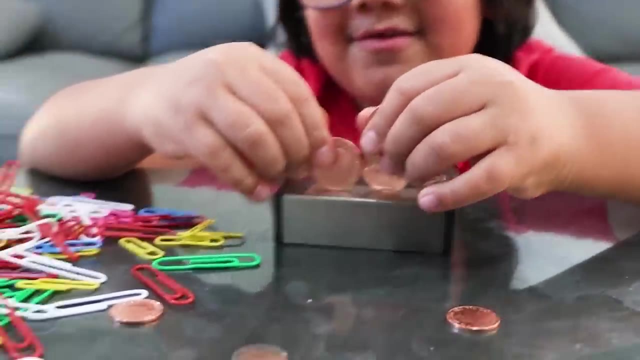 And then this: There you go, And then a little higher. Oh oh oh, How high can you stack? This is hard, It is hard, huh. Okay, while you do that, I'm going to try it too. 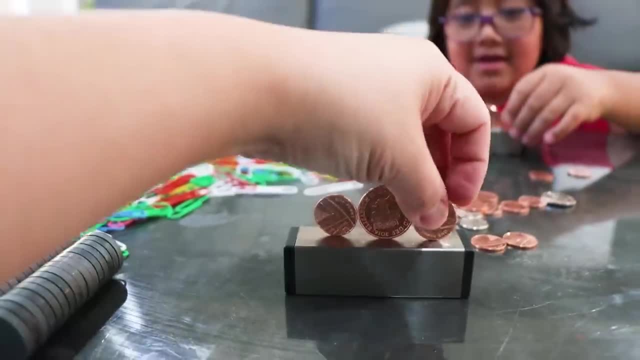 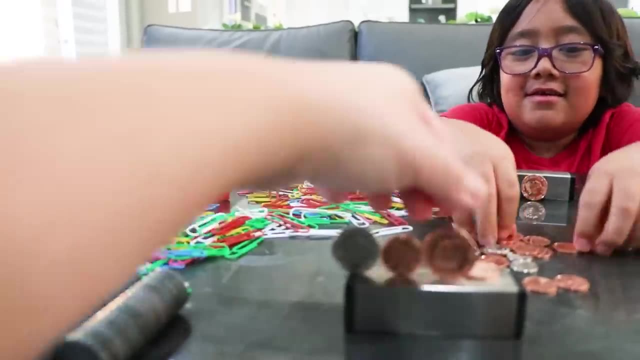 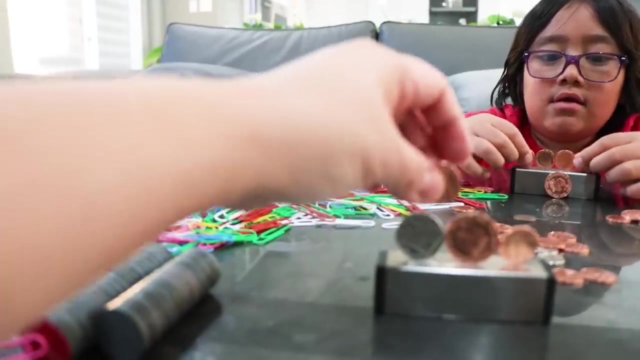 How did they do this? Look, I got three so far. Ryan's still working on his penny So hard. I know Whoa mine keep falling. Yeah, Maybe we're doing it on the opposite side. Why would we? 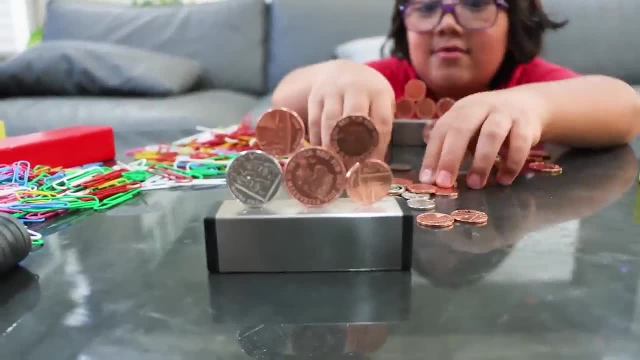 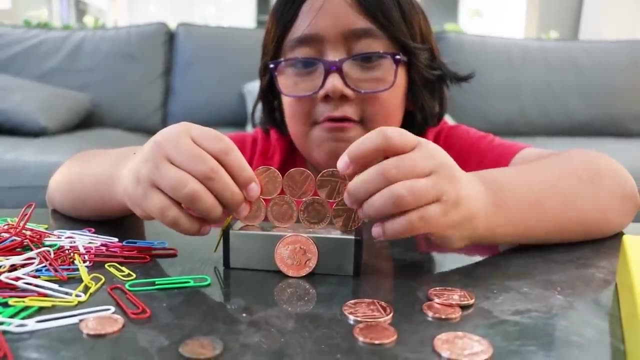 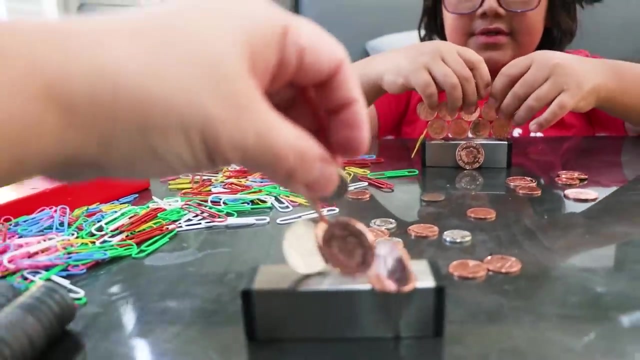 Got it, I got this. Look, this is beautiful. Whoa, there you go, Looking good, Nice, Nice. Oh oh, these are too small coins. Mine fell. Yeah, don't use those coins, Don't use these. 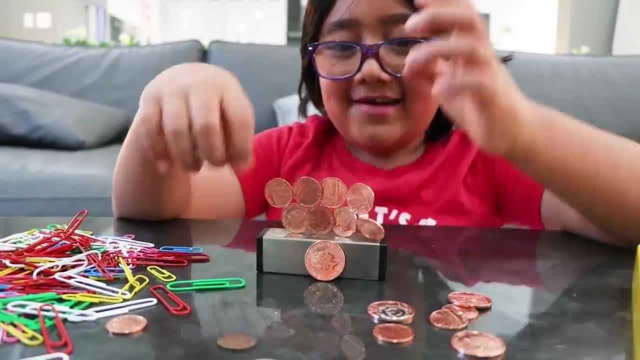 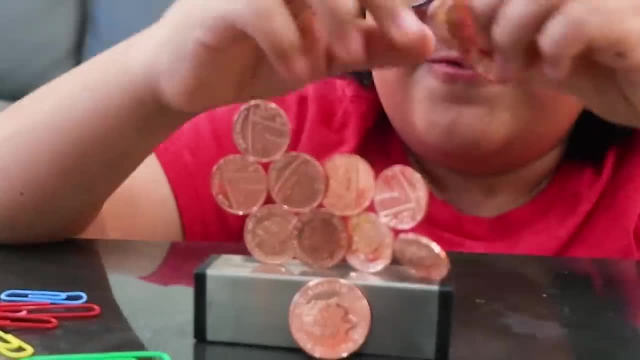 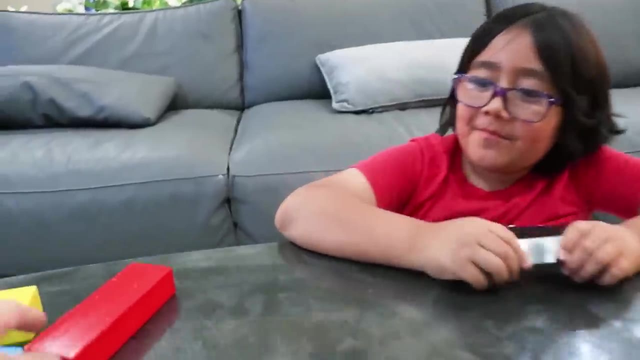 Oi, oi, oi, oi, oi, Whoa. Okay, maybe this. There you go, Yes, Looking good, Oh oh, oh, look at that. Next we're going to stack the blocks here. I want to show you guys this really cool trick. 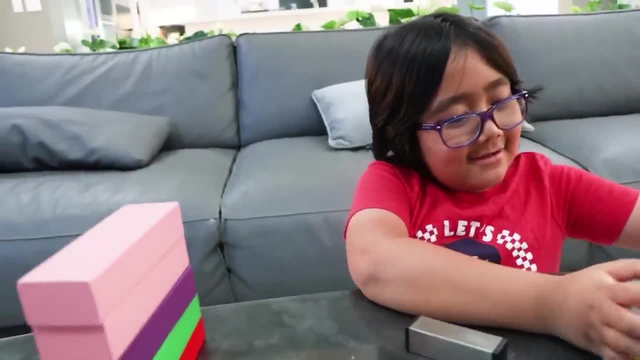 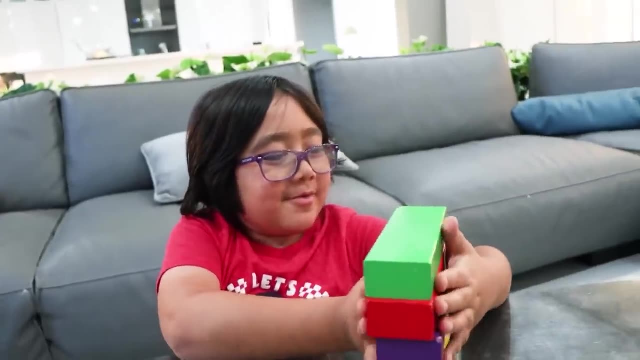 Okay, so I'll stack this side. Okay, just literally stack it up. Okay, Okay, like that, There you go. Wait, maybe I know what you're doing. I don't know 100%. Like that, There you go. 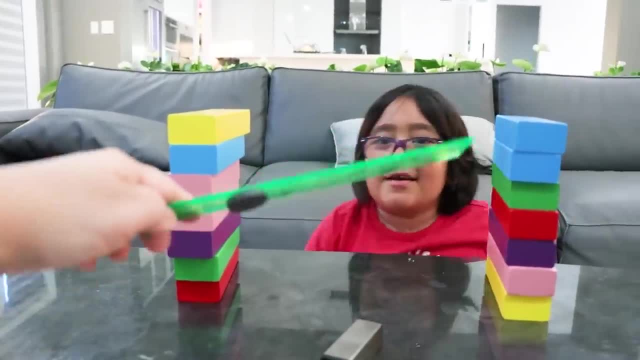 Okay, I have a ruler here where I put a magnet stuck into it. Okay, now I'm going to put this on top Here. hold this, It's going to be like this. There you go, You can put it on top. 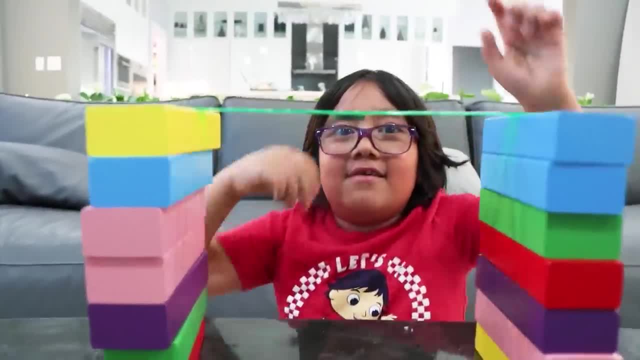 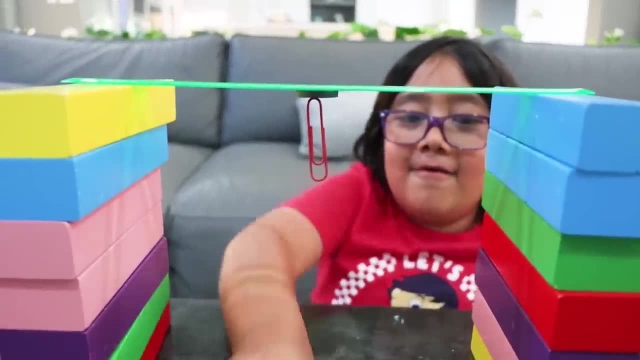 Okay, Okay, And obviously, since the magnet is stuck right there, you know that a paper clip can just go to it, right, Like so. Do you see the paper clip? Yeah, Then I have a string connected to a paper clip here. Do you see the paper clip? 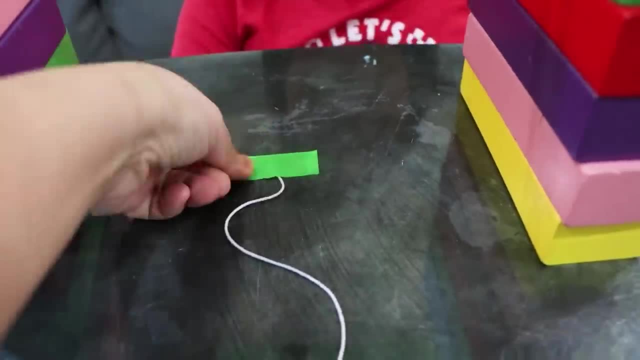 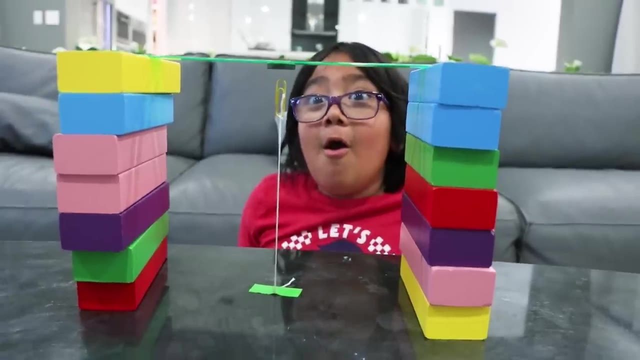 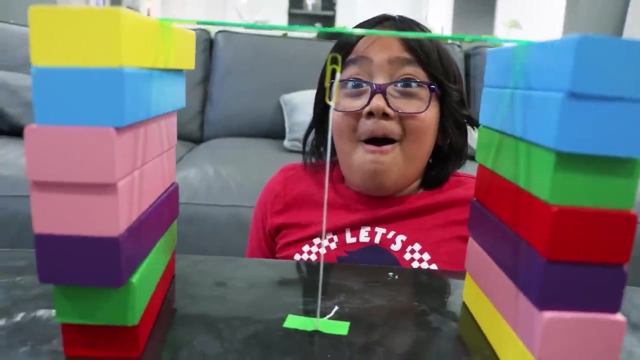 Okay, I'm going to stick it to the bottom. Okay, Okay, Let it go. Okay, Let go of your hand. Oh, Did you see that? What happened? Look at that face. Do you guys see what happened here? 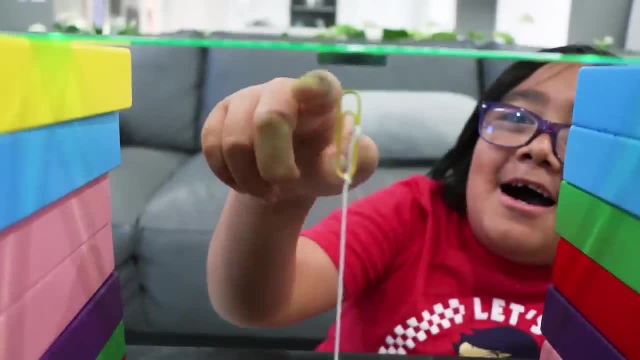 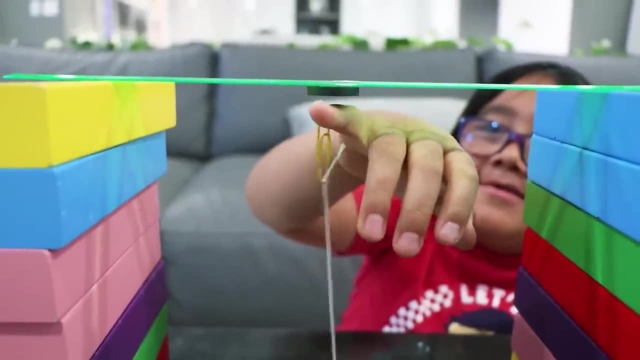 What? Look? what happened to your eyes? Look like it's floating. Can I put my pinky through? Maybe? yeah, I can put my pinky through. Yeah, because it wants to be attached to the magnet. Do you see that?